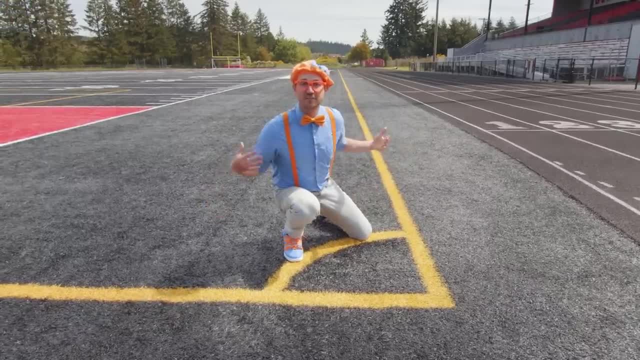 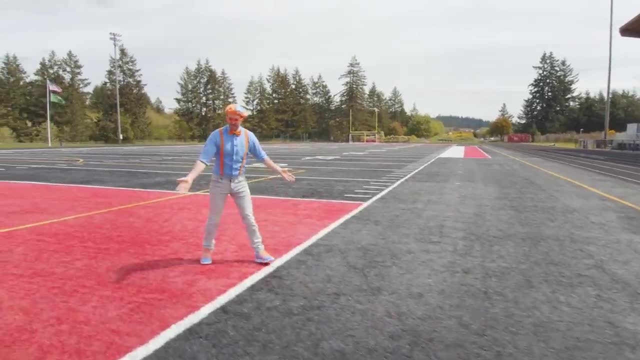 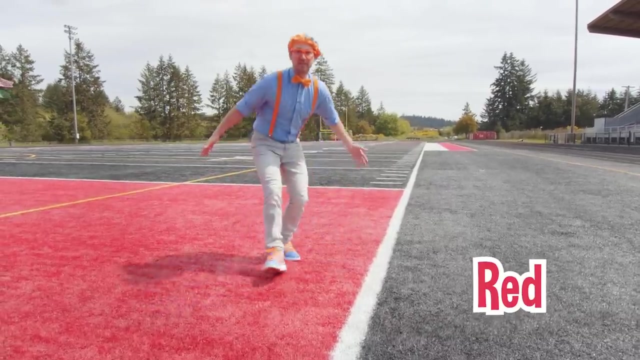 This paint symbolizes the outside, Outside of the soccer field. Yeah, so all the yellow lines on this field are soccer lines, Hey, But there's a lot of other colors, See, like these white lines, Yeah, And this red color, Yeah, you can play a lot of different sports on this field. Wow, What a cool field. 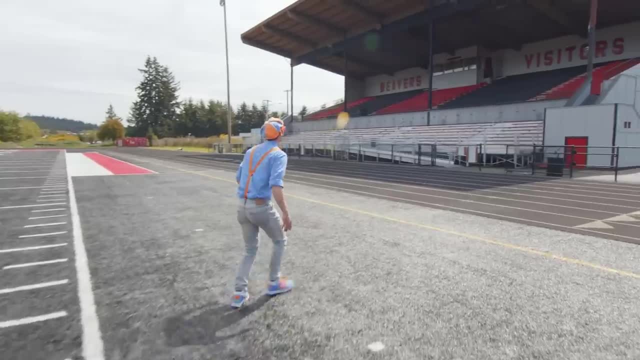 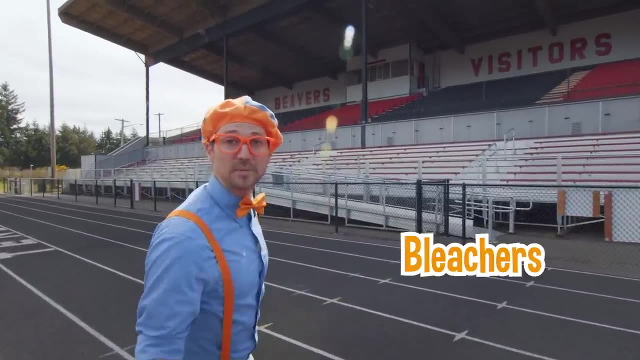 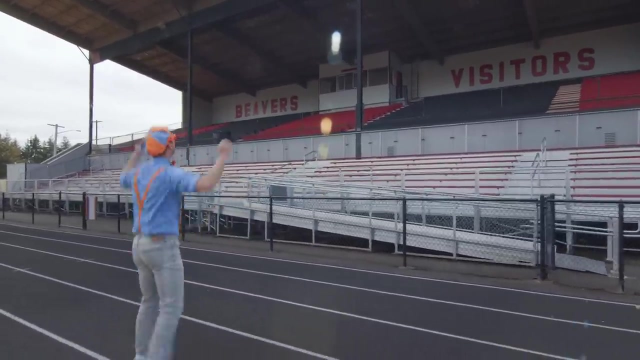 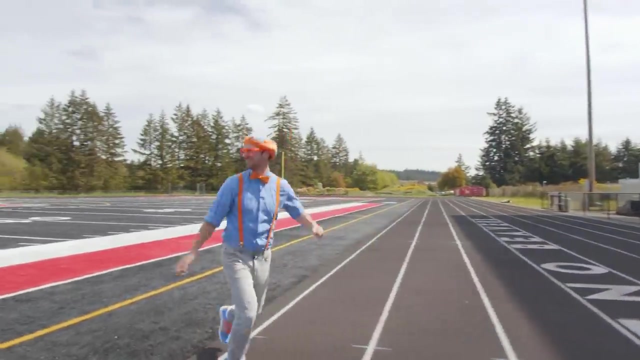 Whoa, Look over here. Wow, This is awesome. These are the bleachers. That's where all the fans sit. Hello, Hey, Yeah, All the stadium fans. they get to root for their very own team. Woohoohoo, Whoa, The very center of 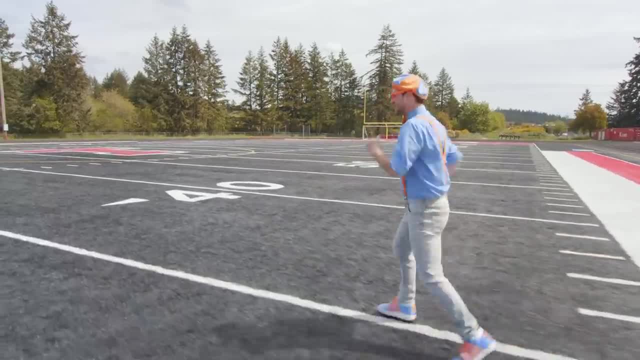 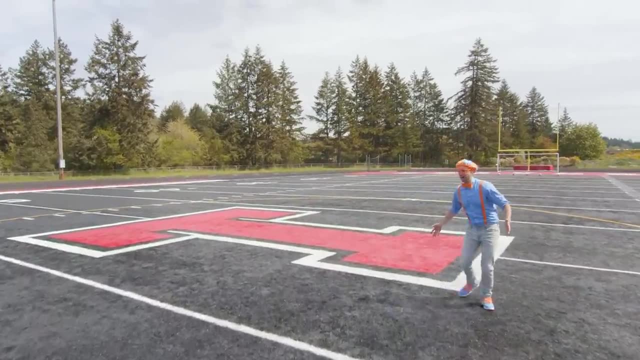 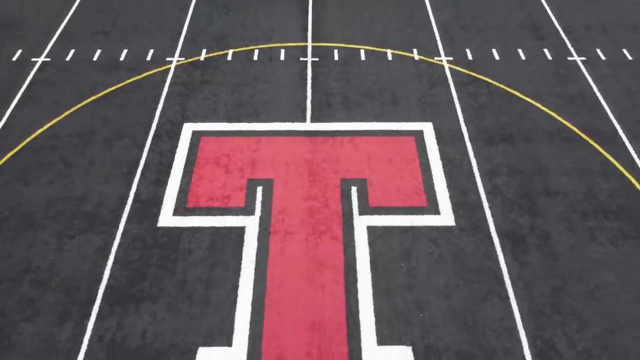 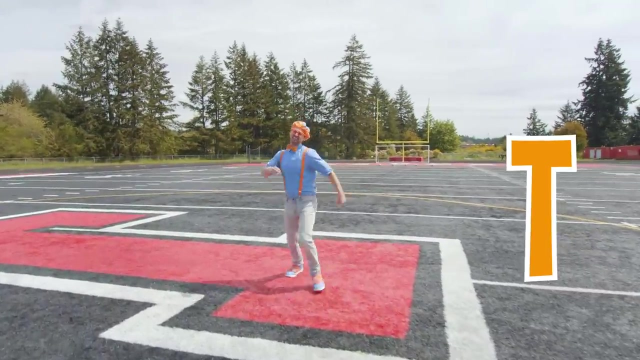 the soccer field has a letter on it. Let's go see. Wow, Now this is a big letter. Whoa, do you see what letter that is? Yeah, you're right, It's the letter T? T for Tenino Washington. 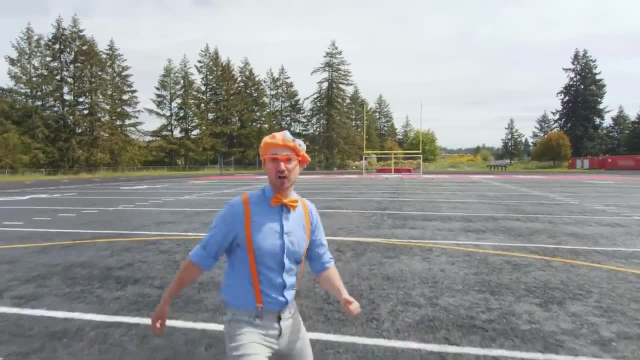 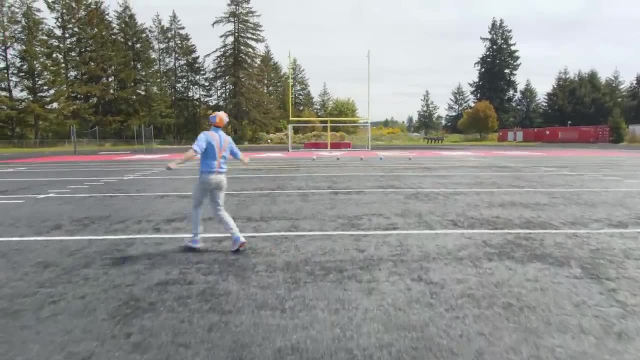 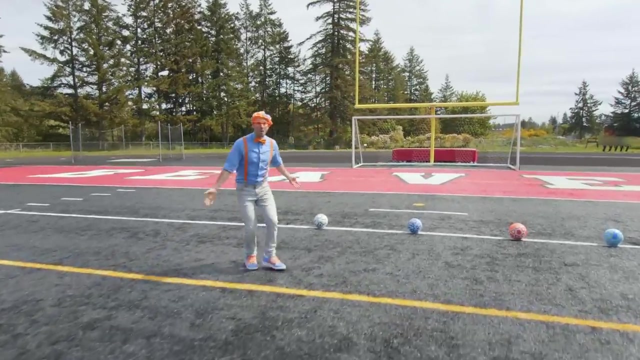 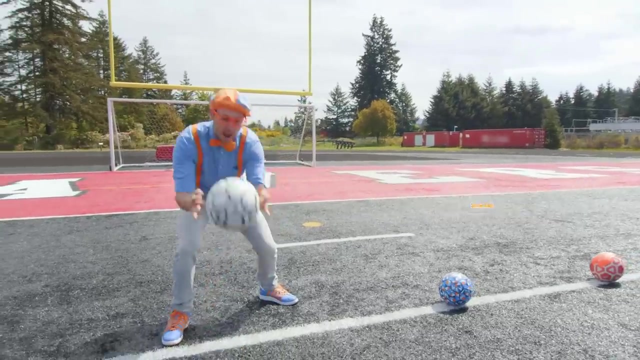 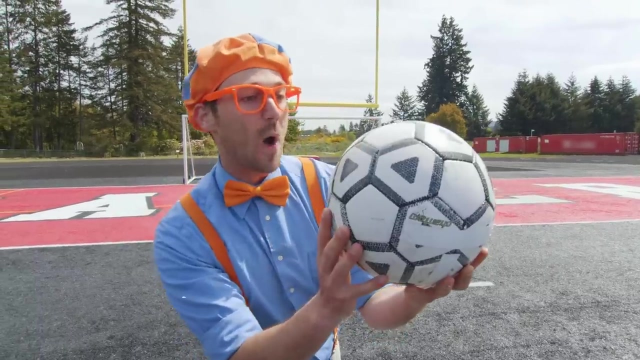 Yeah, Whoa, there's some more soccer equipment down here. Let's go. Whoa, do you see these? Yeah, these are soccer balls. Wow, check it out, What a cool ball. This ball is a color: white and black. 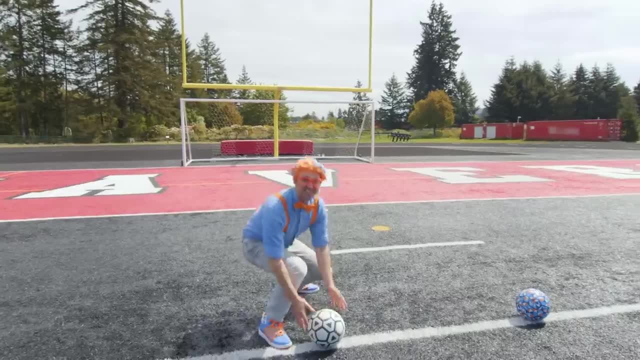 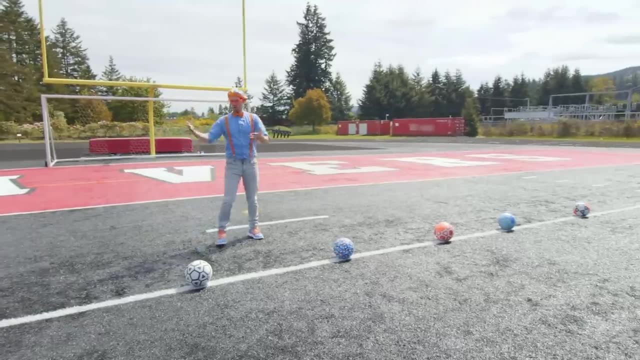 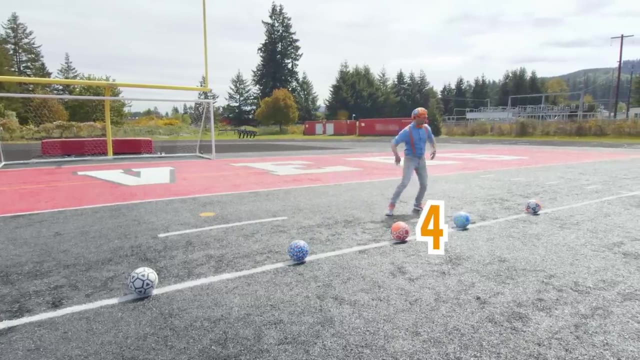 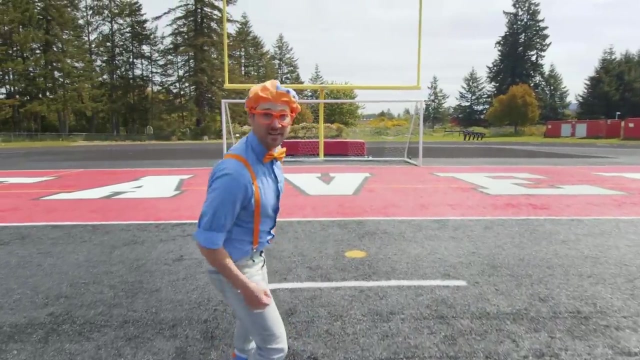 Watch this. Yeah, in soccer you don't use your hands. Hey, let's count these soccer balls. Looks like we have one, two, three, four, five soccer balls. Whoa, do you see that behind me? That is the goal. 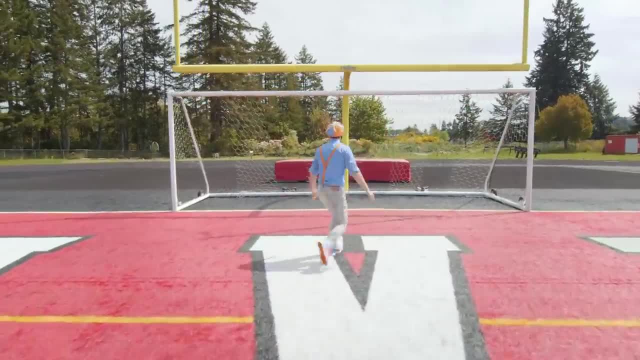 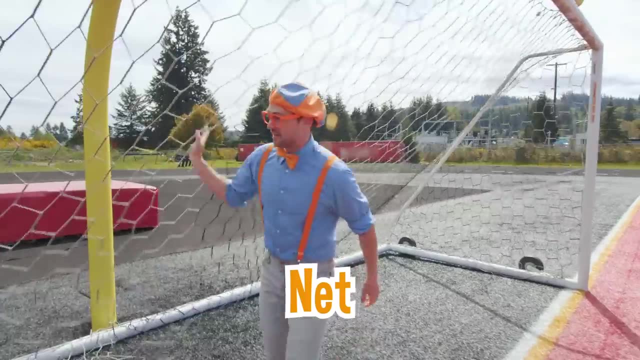 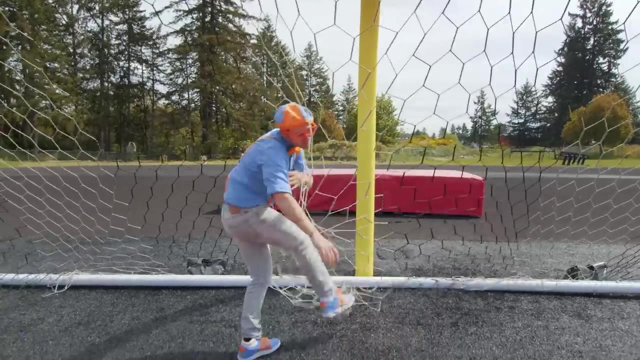 Let's go check it out. Wow, do you see this? Yeah, all this netting. If someone kicks the soccer ball into this netting right in here, Whoa, whoa, whoa, oh, oh, I'm stuck. 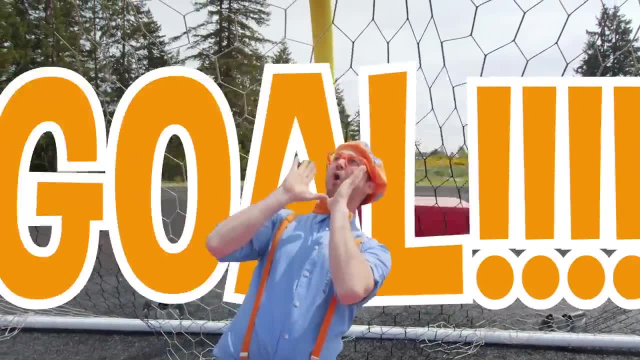 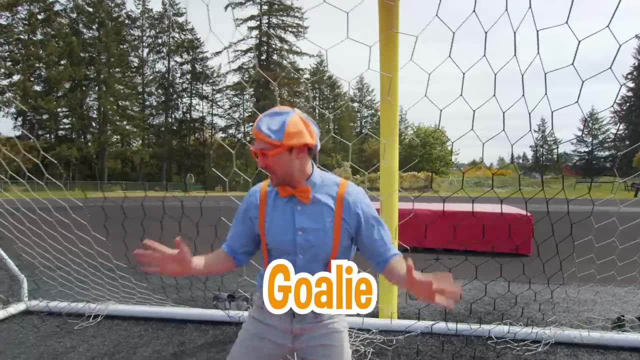 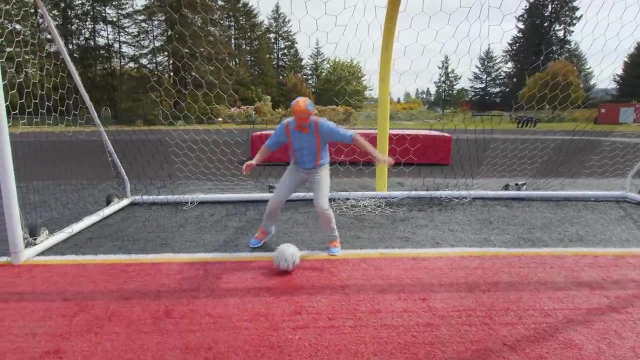 Wow, then that means you got a goal. Whoa, then that means you got a goal. And who stands right here is called the goalie. Yeah, they make sure that nothing goes past them. Whoa, I'm ready. Yeah, do you see how I use my feet to kick the balls out? 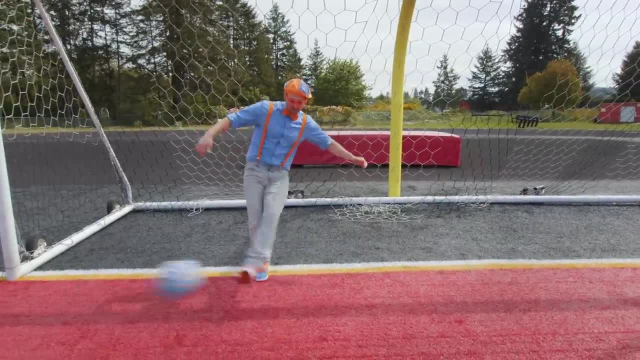 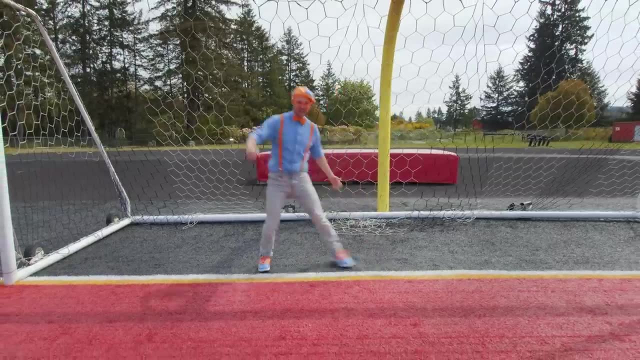 To kick the balls out of the way. Whoa, the goalie's job is to make sure that no balls go past. Yeah, whoa, yeah, this is fun being a goalie. Whoa, do you see how I caught that ball? 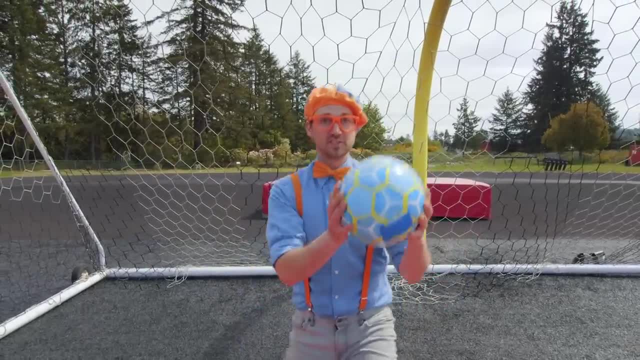 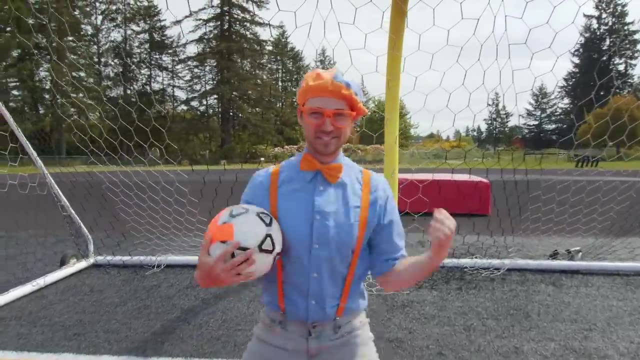 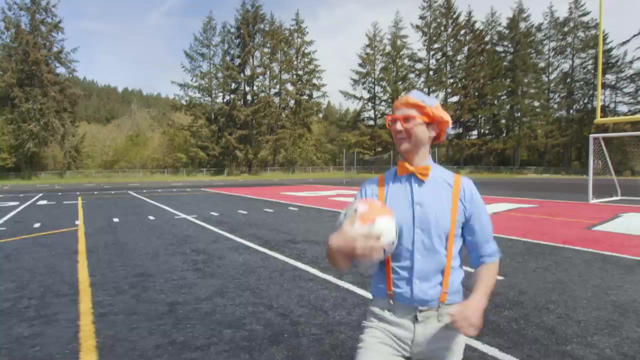 Goalies are the only players in soccer to be able to use their hands. Woo-hoo, whoa, I am such a good goalie. Ha, woo-hoo, Whoa. who's that? That's my coach. yeah, Oh, hey, Coach Kevin. 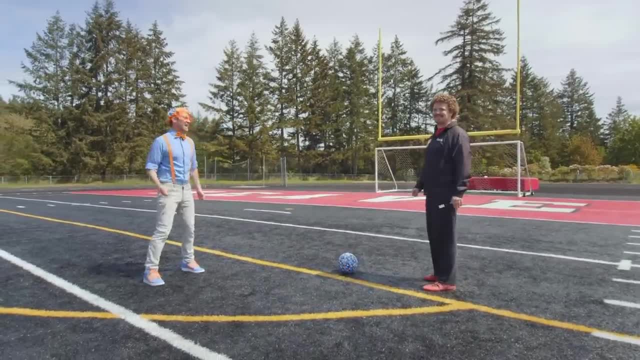 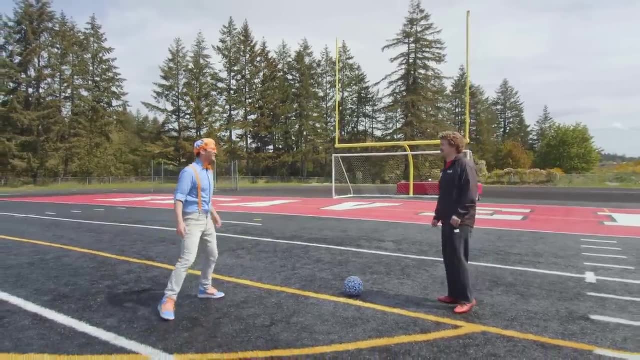 Hey, Blippi, How are you doing today? Good, how are you? Oh good. Hey, I heard you are the best soccer coach in all of the 9-0 Washington. is that true? Oh yeah, Oh, that's awesome. 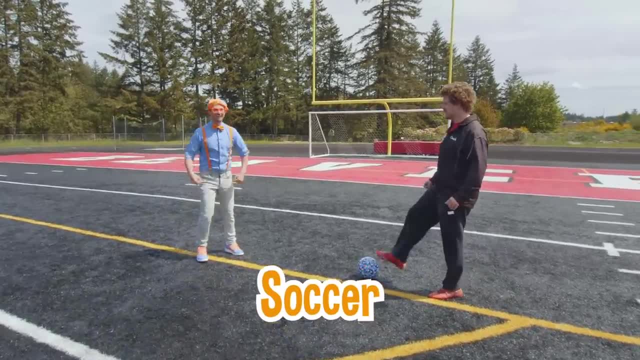 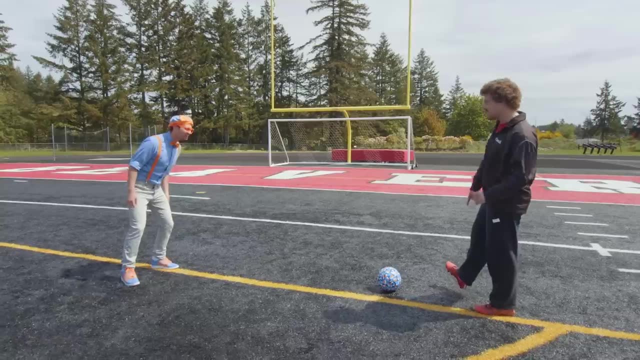 Hey, will you teach us some soccer lessons today? Yep, let's do some soccer, Okay, well, what do we start with? We're gonna start with some passing. Okay, that sounds fun. how do you do it? All right, so you wanna have the inside? 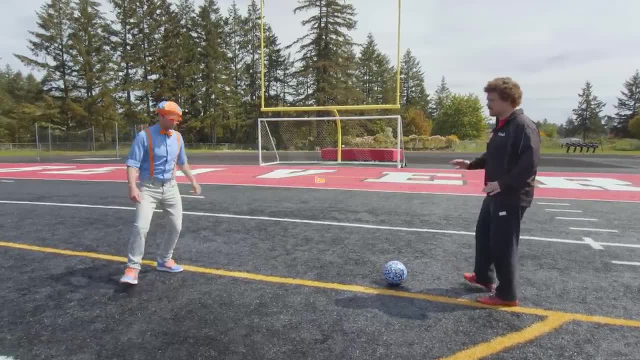 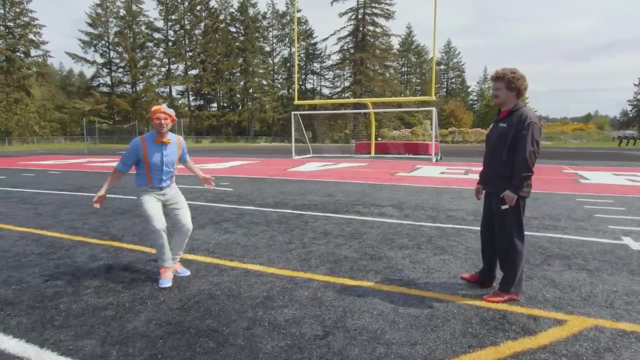 the inside of your foot. when you pass, you're gonna point your toe up a little bit to keep the ball on the ground. Okay, Yep, here we go. All right, Whoa, that was such a good pass. Let me try. 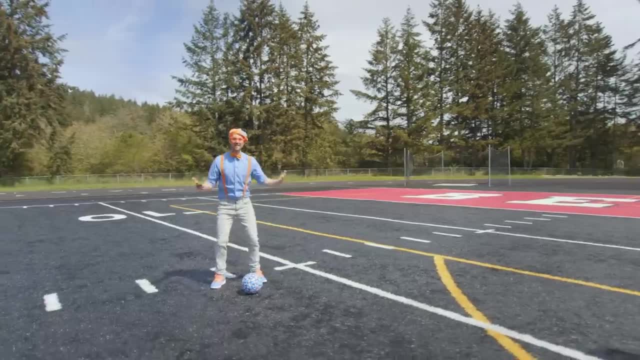 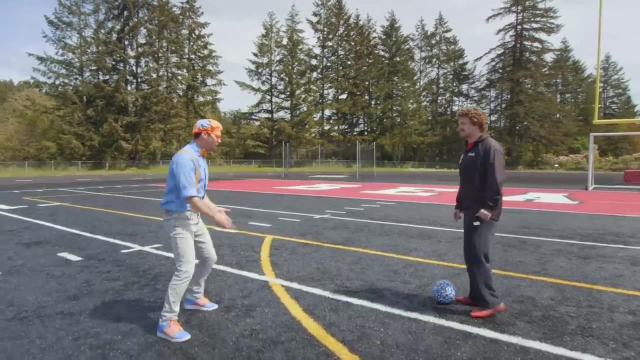 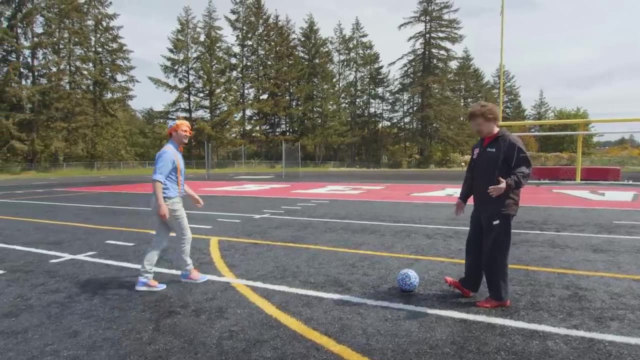 Okay, I set the ball down, I use the inside of my foot and I pass it. Whoa, I did it. Whoa, You stopped it. how did you do that? Yeah, we call that trapping in soccer. So same kind of idea. we want our toe up. 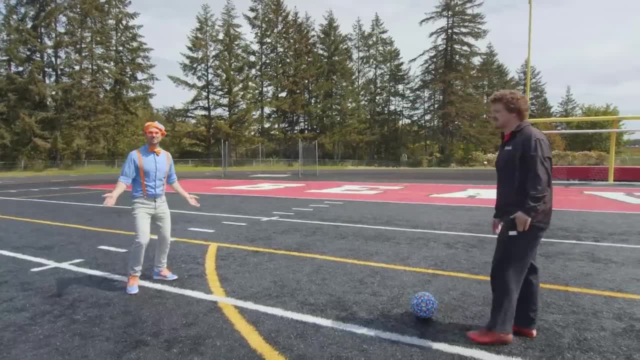 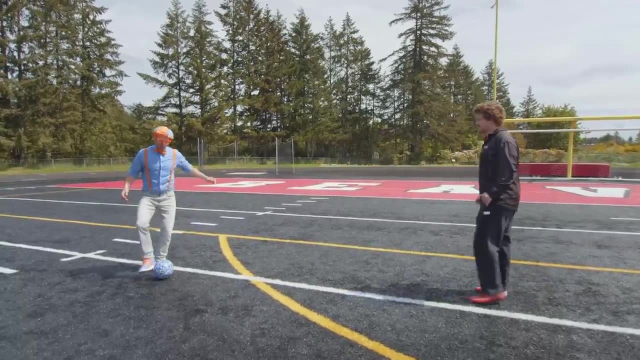 in the inside of our foot and we just kind of catch it with our foot. Okay, so trapping is basically like stopping the soccer ball. All right, let me try. Whoa, did you see that I stopped the soccer ball with my foot? 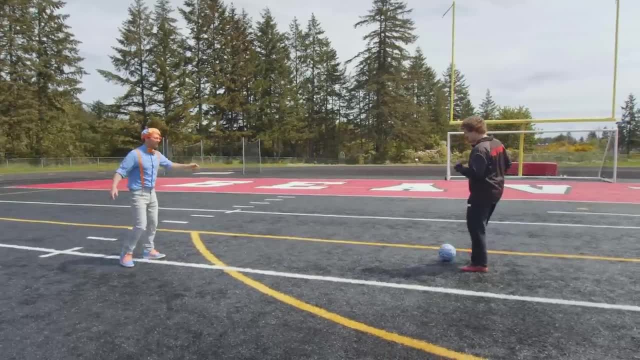 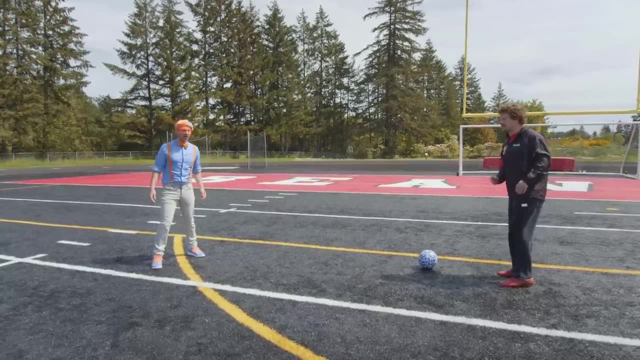 Okay, let me pass it back to you. Whoa, this is so much fun. Well, what's next? Now we need to pass and move, pass and move at the same time. Okay, all right, let's try it. 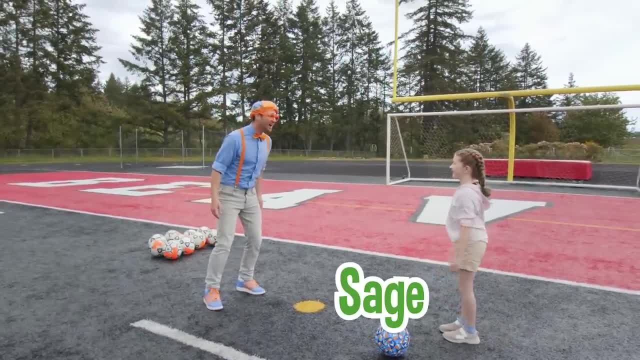 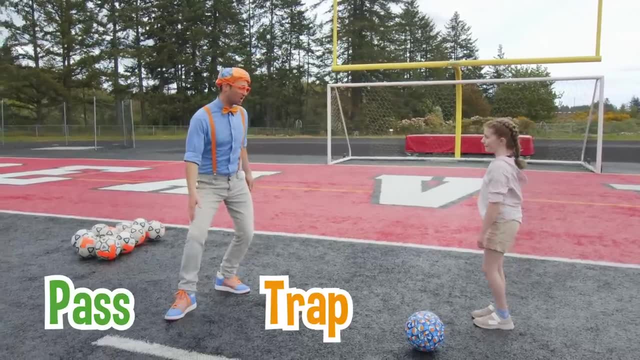 Whoa, who are you? Hi, I'm Sage. Oh nice to meet you, Sage. I'm Blippi. Well, hey, I just learned how to pass and trap the ball. Will you teach me how to shoot the ball? 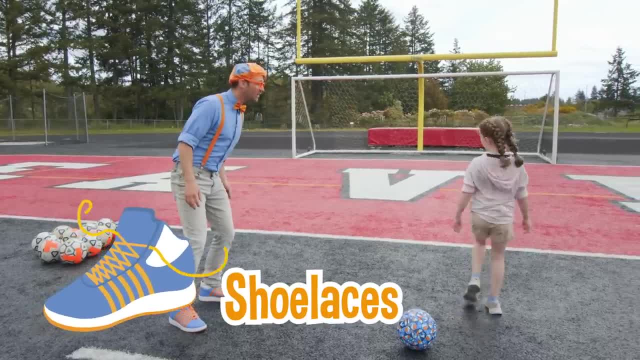 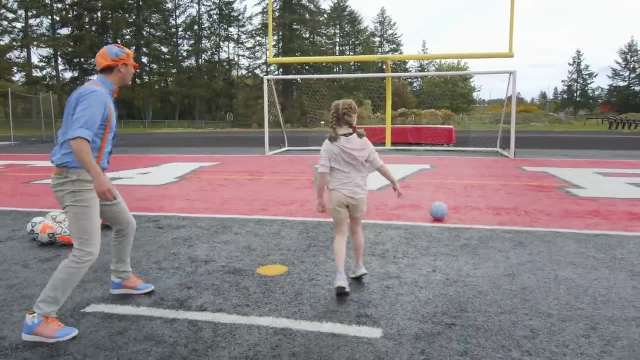 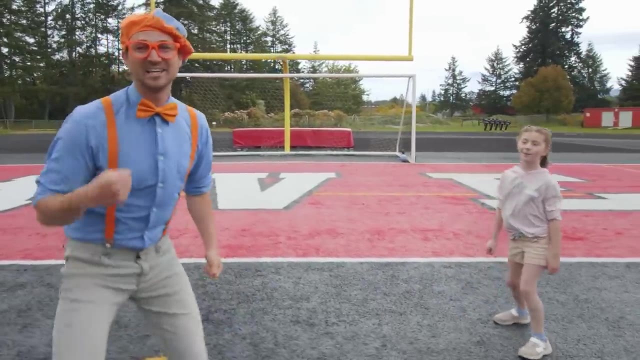 Yeah sure, All you really need to do is use your shoelaces to kick the ball into the goal. Okay, that sounds pretty easy. Will you show me? Yeah sure, Whoa, that was awesome. Good shoot. Yeah, she just made a goal. 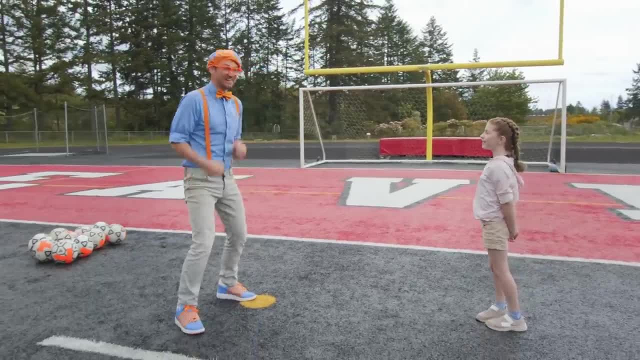 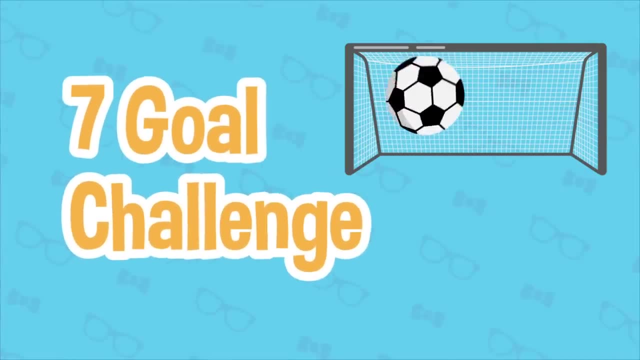 Well, hey, do you mind if I try? Yeah, sure, Good luck, Blippi. Yeah, thank you so much. Sounds like a great challenge. It's the seven goal challenge. Blippi needs to get seven goals to earn the soccer medal. 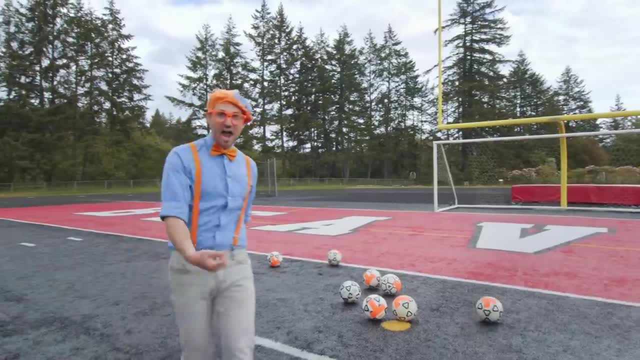 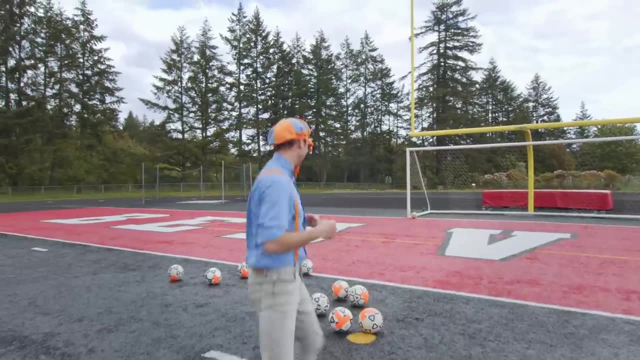 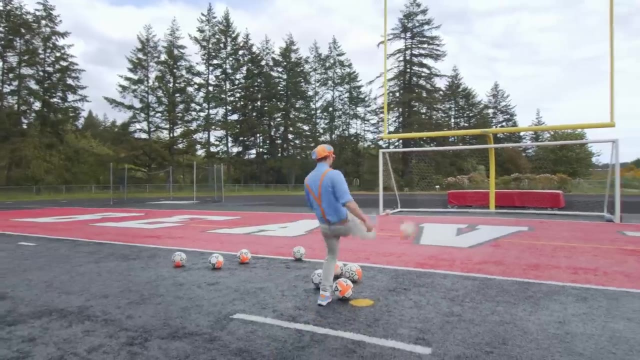 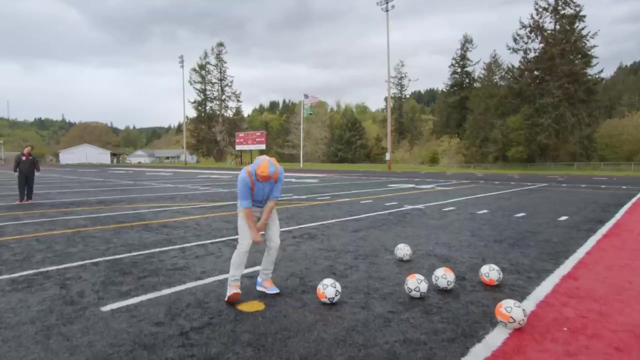 Will you count the goals he makes? Here I go: Woo-hoo-hoo-hoo, I did it. Yeah, another goal. Whoa, that was awesome. Aw, That's okay, I'll just try again, Ha-ha. 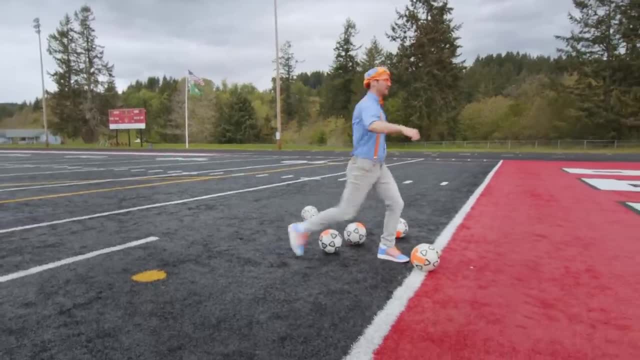 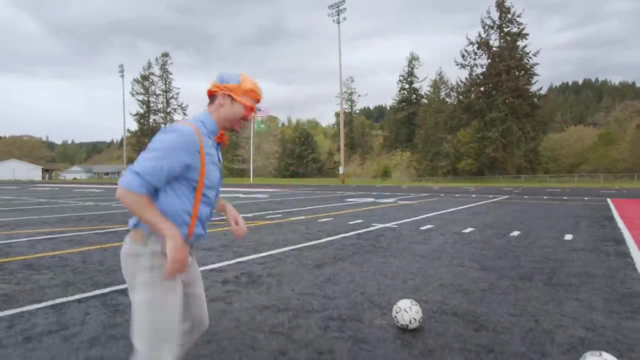 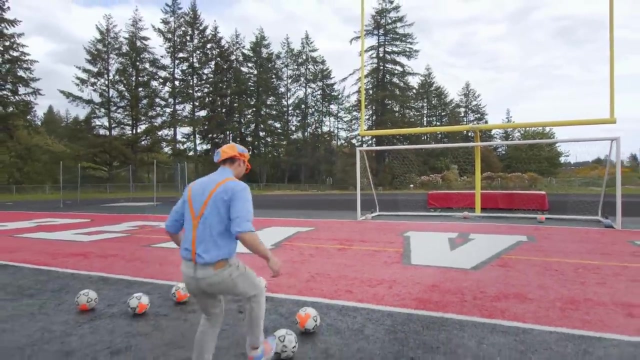 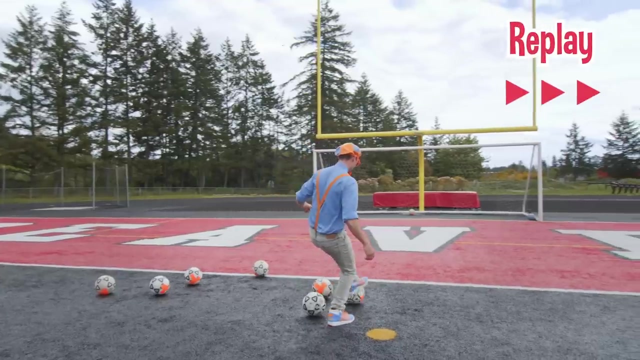 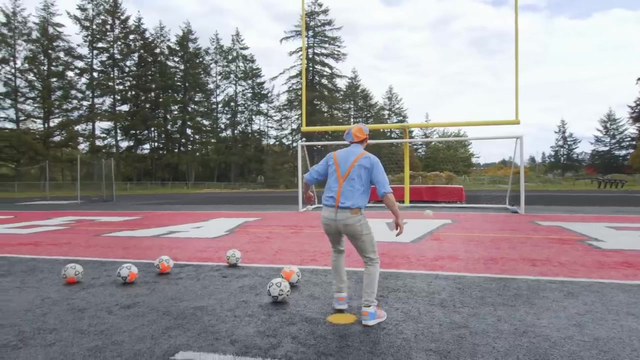 Yeah, I love soccer. Yeah, that was a swish Ha-ha-ha-ha, Whoa-ho-ho-ho, Goal, Goal. Blippi did it. Let's see an instant replay. Look at that form. 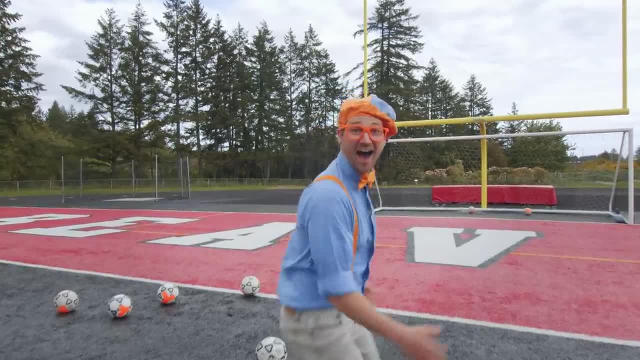 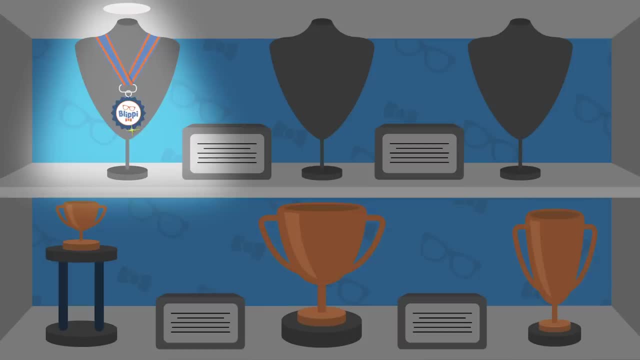 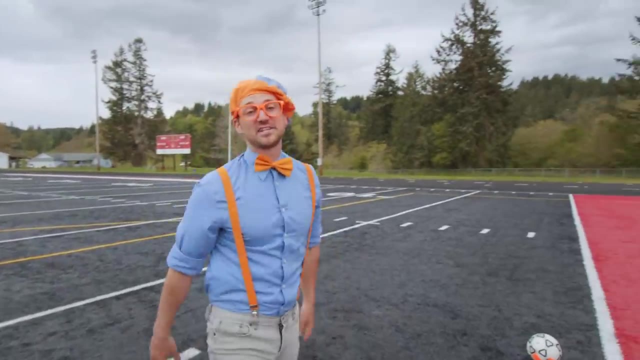 Nothing but net. Soccer takes a lot of hard work, but with some training and practice you can become a champion. Way to go. Blippi, Yeah, Wow, that was awesome. I just scored seven goals. Yeah, Wow, that is so many goals. 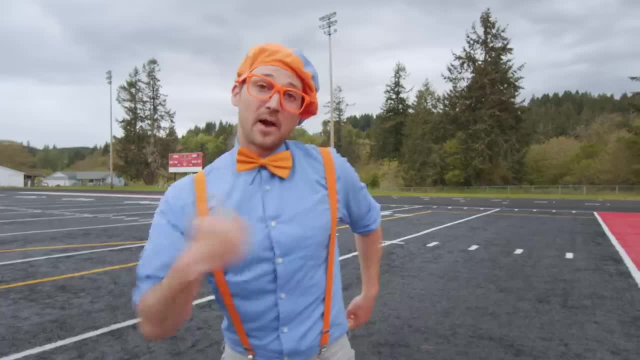 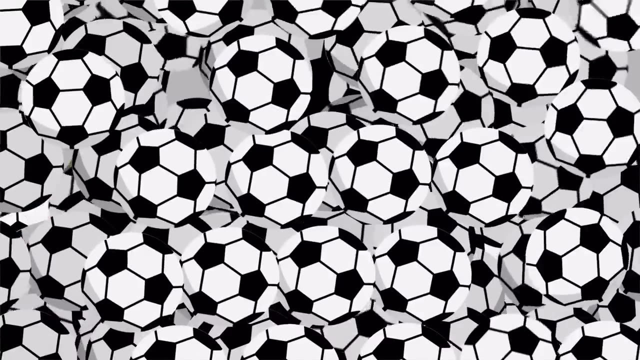 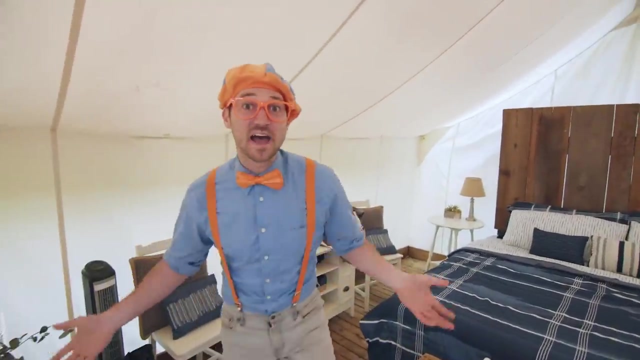 Wow, soccer is such a fun sport. Well, I should probably get going back to the summer games tent to see what else there is. Thank you so much. See you later, Bye-bye. Whoa, wasn't that fun learning how to play soccer together. 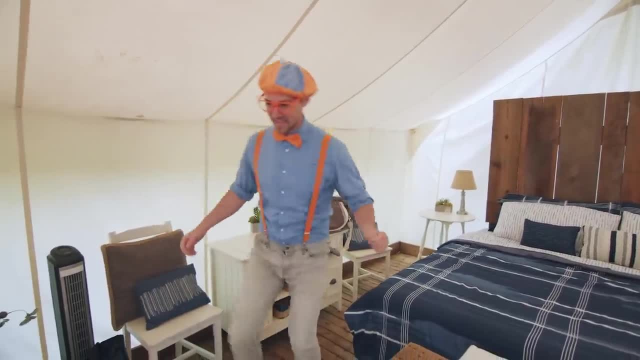 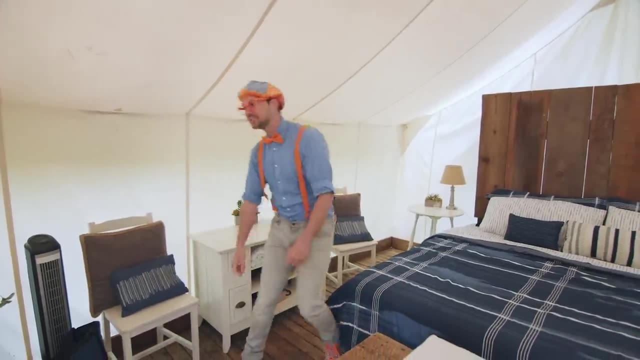 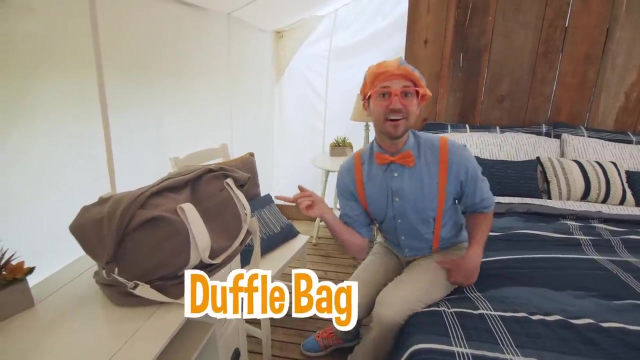 Yeah, it was so cool kicking the soccer ball with our feet, Yeah, woo-hoo. And using your hands only if you're the goalie. Oh jeez, I am so tired I should probably take a breather. Oh look, a duffel bag. 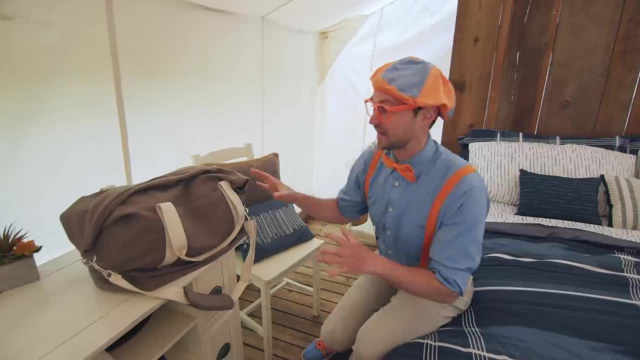 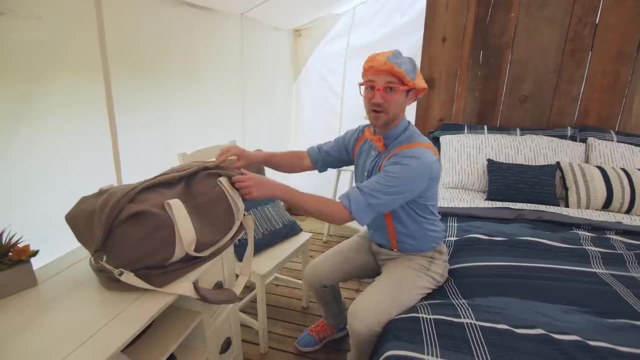 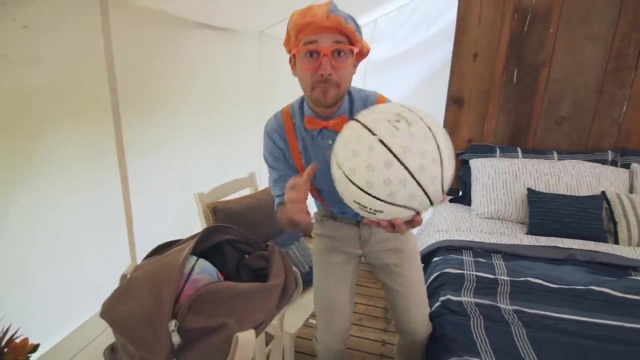 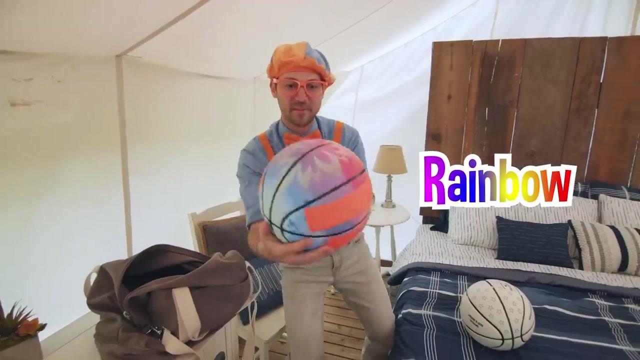 I wonder what they put inside this duffel bag. A duffel bag is used to store things in it, and in this case, sports equipment. Yeah, I wonder what's in here. Whoa Yeah, Basketballs: A white basketball and a rainbow-colored basketball. 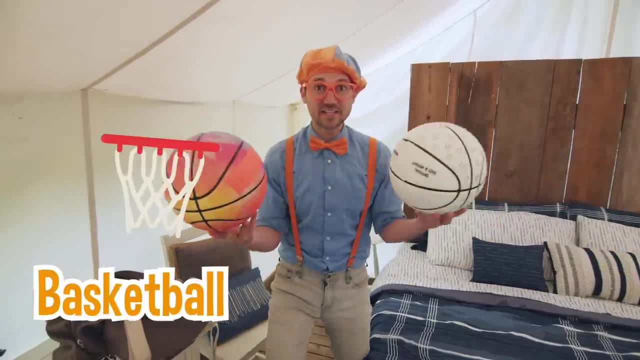 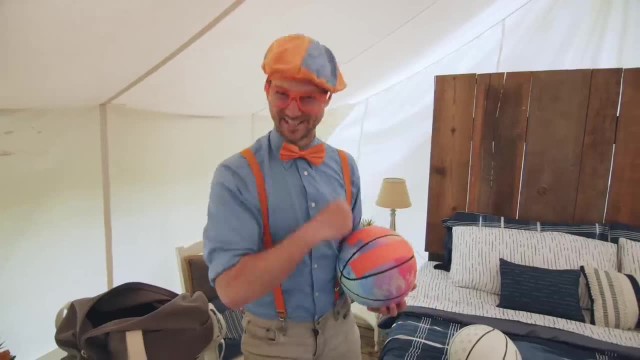 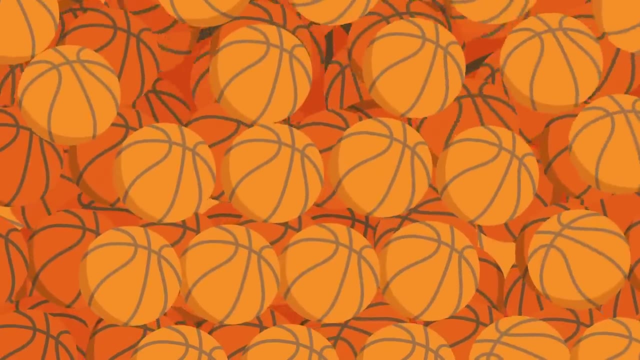 Whoa, two basketballs. Have you ever played basketball before? Yeah, it's so much fun shooting it and scoring a point. Let's go to the court and learn some basketball. Oh, I probably need this. Come on, let's go. 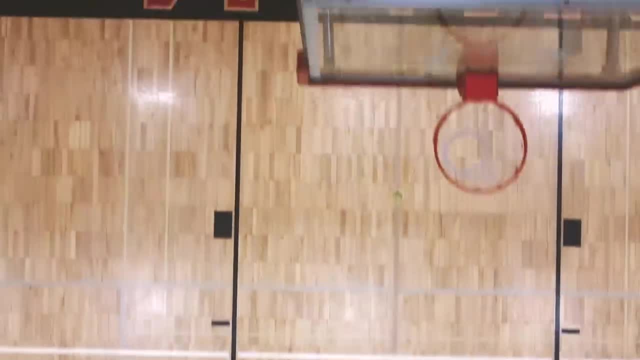 Come on, let's go. Come on, Let's go. Woo-hoo-hoo, What is this? Ooh, look, It's a store that sells basketball. Yeah, let's go see. Oh, okay, Let's go. 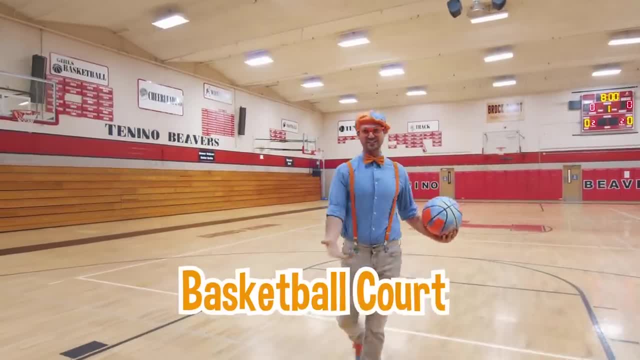 Let's go, Let's go. I'm excited, Let's go, let's go, let's go. Yeah, let's go, Let's go, let's go. Whoa, this is amazing. Wow, come on in. 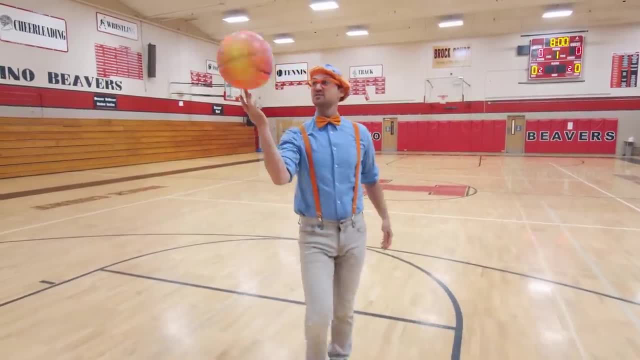 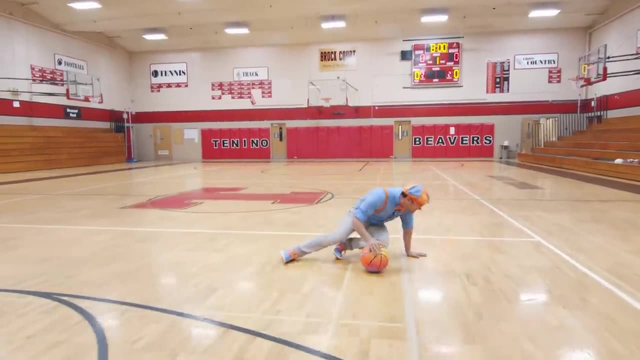 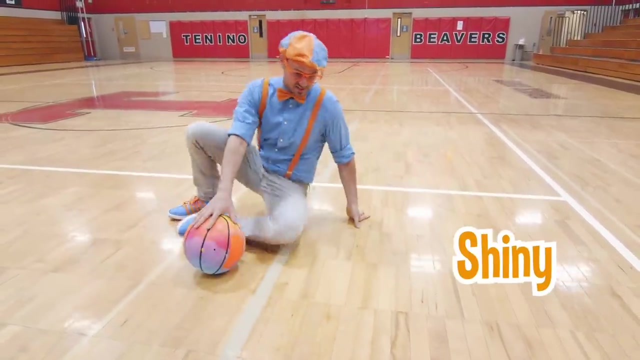 This is insane. Look at all the people here, And that's what I'm talking about: Whoa, Whoa, Wow, Wow of wow. do you see this? whoa? this is a really special wood and it's so shiny, yeah, so then? 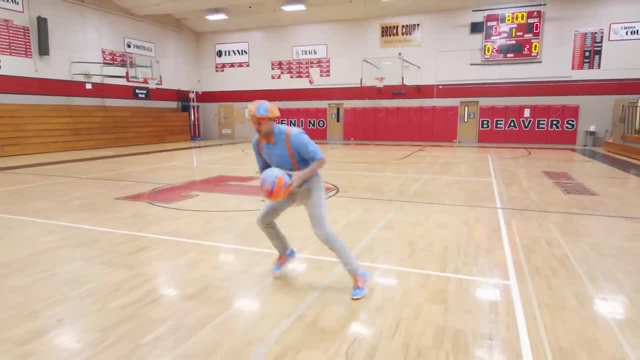 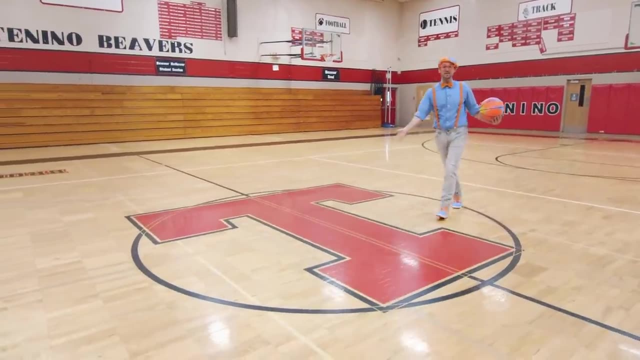 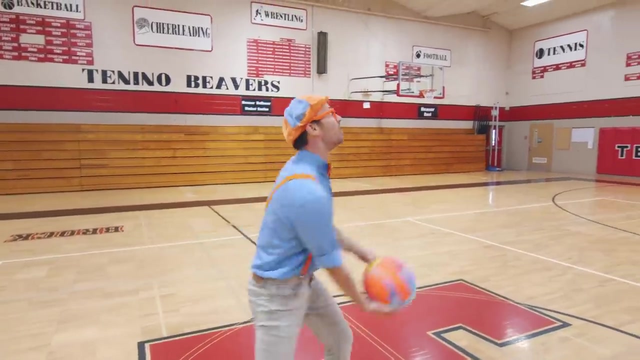 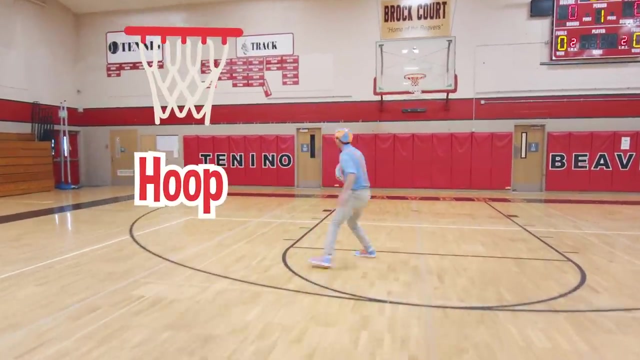 when you play some basketball, you don't slip and slide. whoa, hey, check this out. this is the center of the court. they call it center court. wow, how clever. yeah, this is where the game starts, and over here there's a basketball hoop. whoa, yeah, see that up there. that looks like a circle. 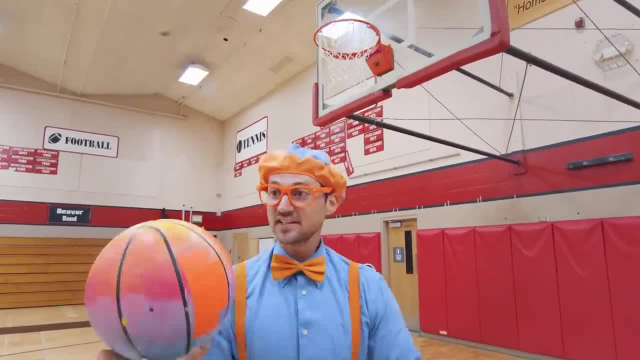 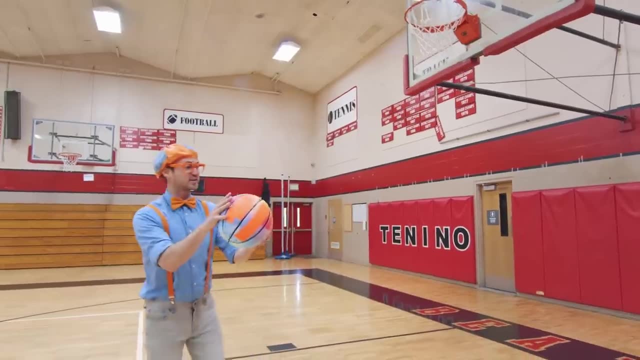 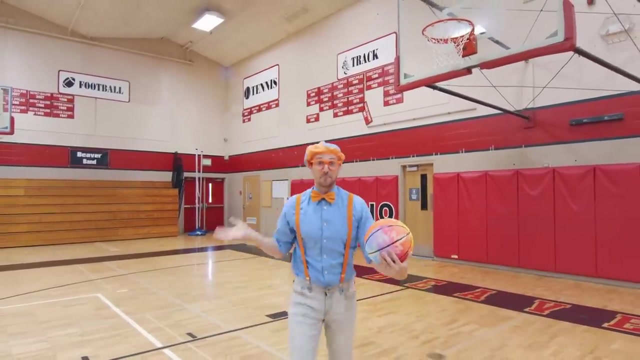 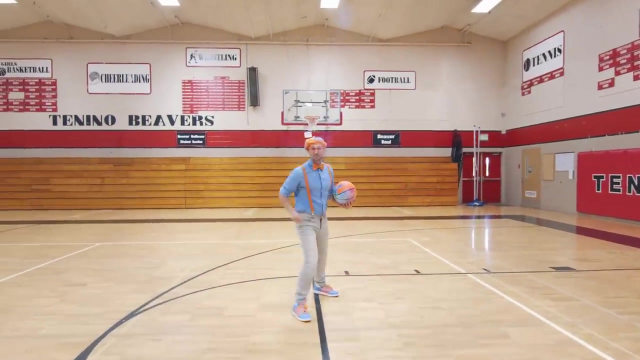 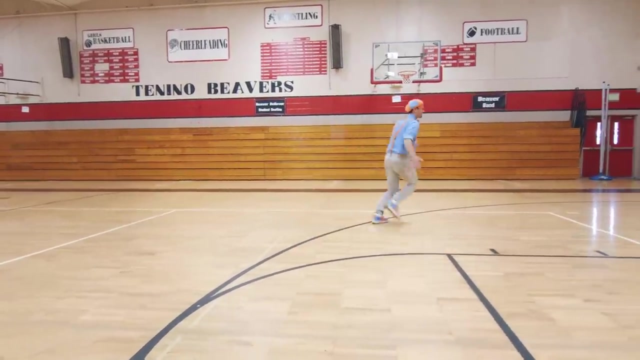 and you see what shape the basketball is. this is also a circle. yeah, the point of basketball is to put this circle inside that circle. that sounds like a fun game, but hey, how the points work. yeah, is anything in front and closer to that basketball hoop, from this line right here, and it goes all the way around over here. yeah, all the way to the other. 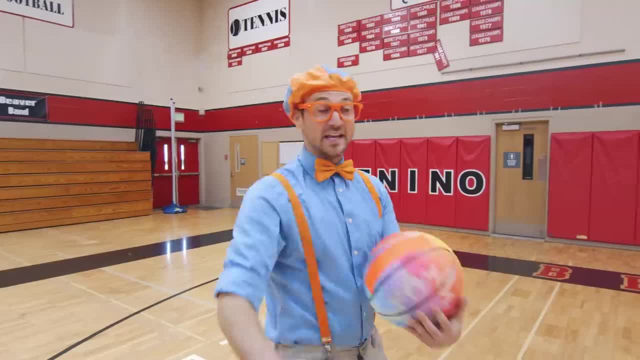 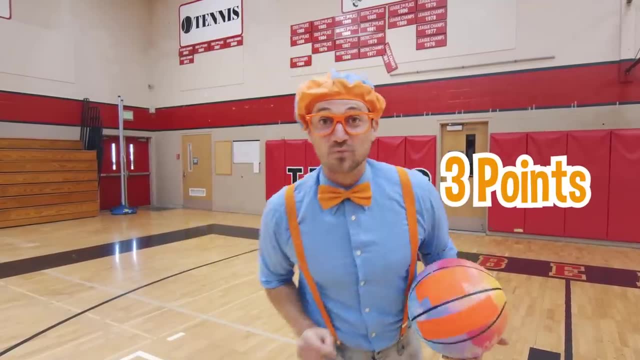 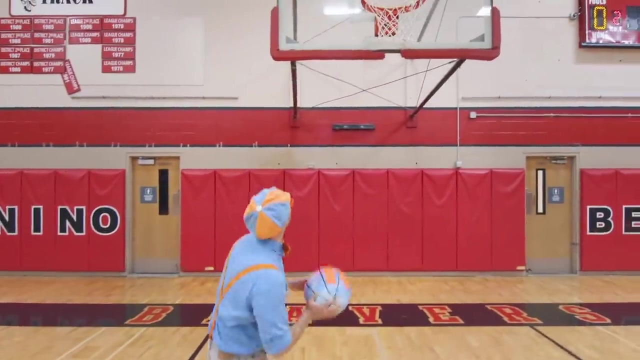 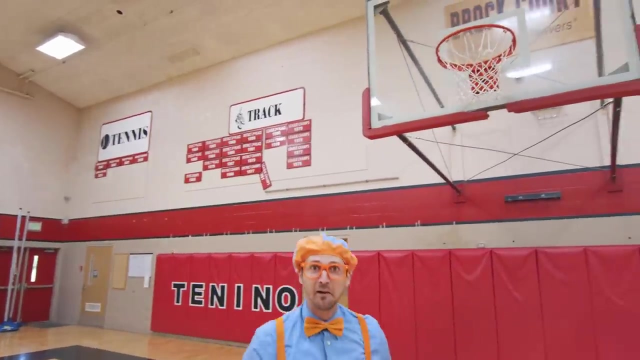 side, anything closer to the basketball hoop is two points. anything on the further side of it is three, and that's why they call that the three-point line. all right, let me show you how to do it. oh, i missed. oh, i missed again. this is really fun, though. 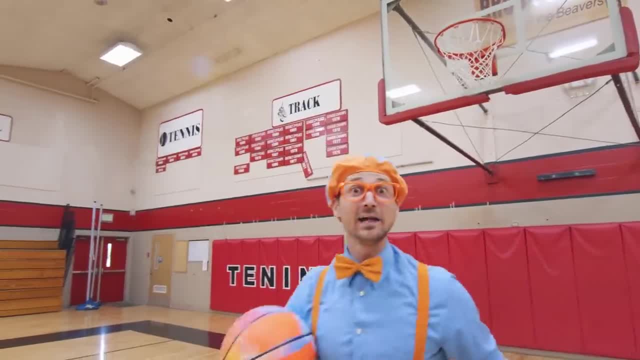 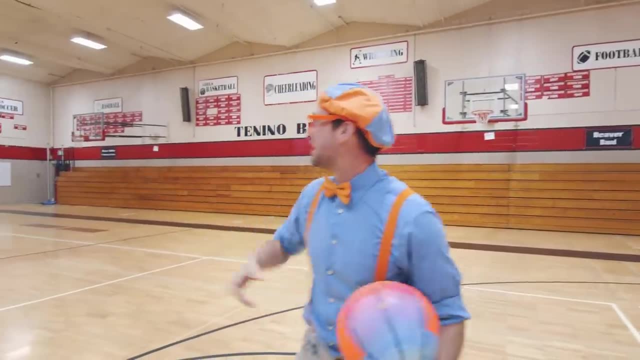 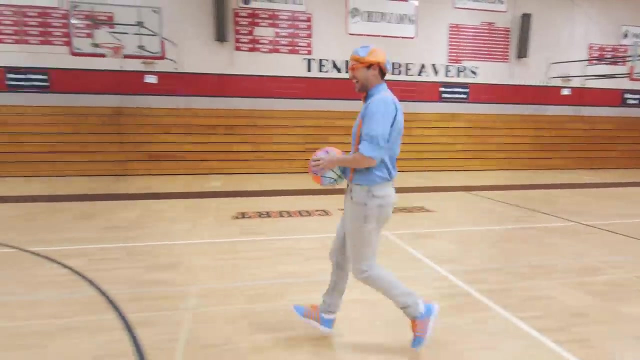 i'm not very good. whoa, that's crazy. well, since i'm not very good, maybe i should take some lessons. hey, look, that's coach joe over there, let's take some lessons. hey, coach joe, how are you good, blippy, how are you? oh, pretty good. hey, will you teach us some? 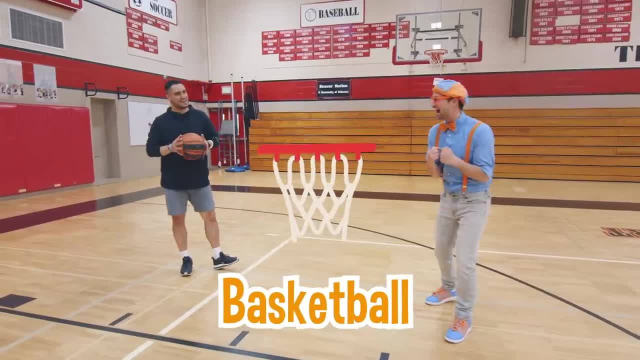 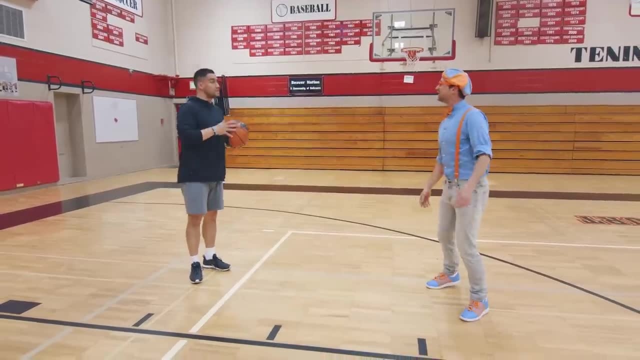 basketball skills today, of course. yeah, what are we going to learn? i think today we probably should start with dribbling. oh, that sounds like fun. how do you do it? well, dribbling is really bouncing the ball, but being in control of it okay. so we want to make sure, when you're dribbling, you're using 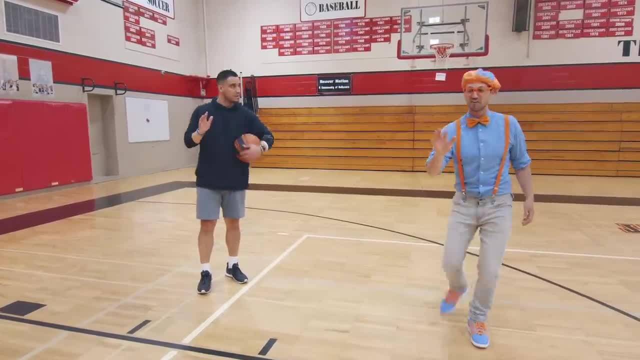 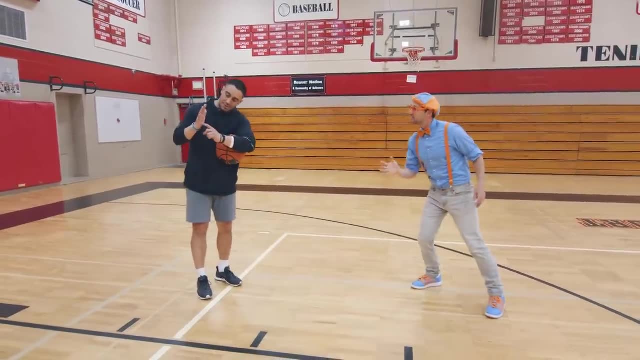 your fingertips and the pads of your fingers. good job, right there, you're doing it. well, what do you do? Oh, okay, so we use our fingertips and the pads of our fingers? That sounds like fun, Yep, and then you want to make sure that you're not using the palm. 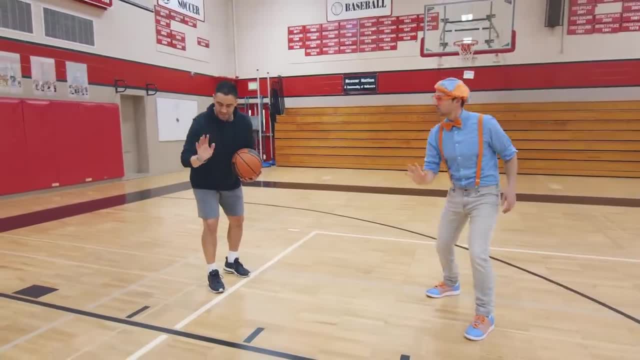 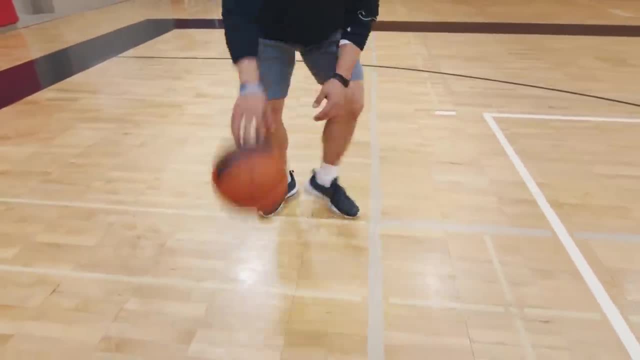 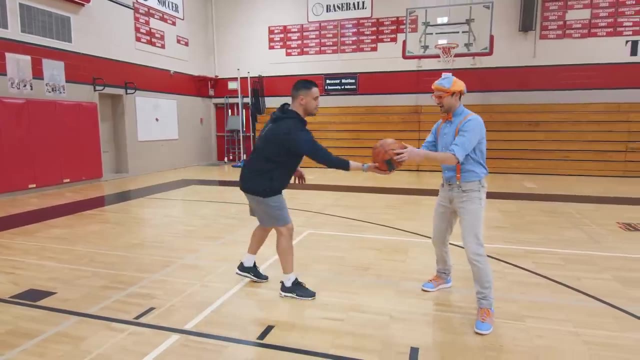 only the fingertips: Perfect, awesome. And then you get a little bit of flexibility in your wrist and you bounce the ball. Whoa, You want to try? Yeah, let's try it out. Here we go, Here we go. 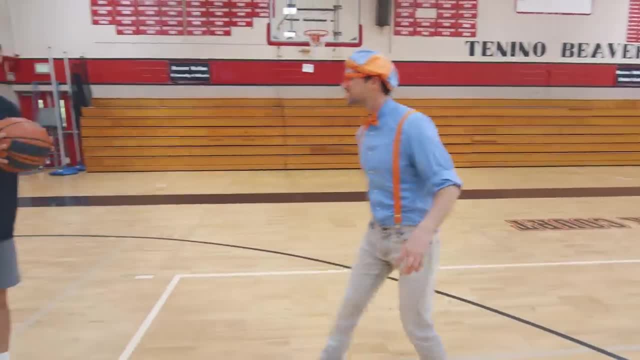 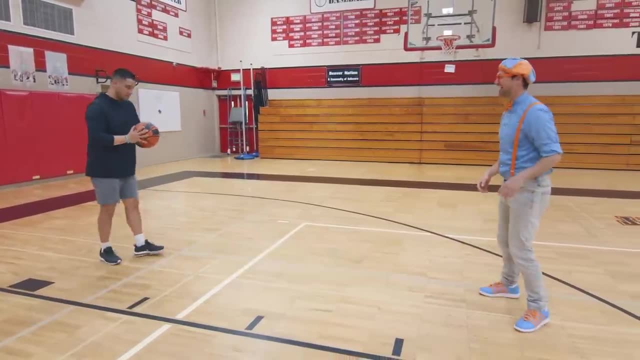 Wow, that was awesome. Nice, There you go. Nice. After dribbling, we probably should go into passing. Okay, Basketball is a teamwork sport, so we got to make sure we have good passes. Yeah, all right. so how do you do it? 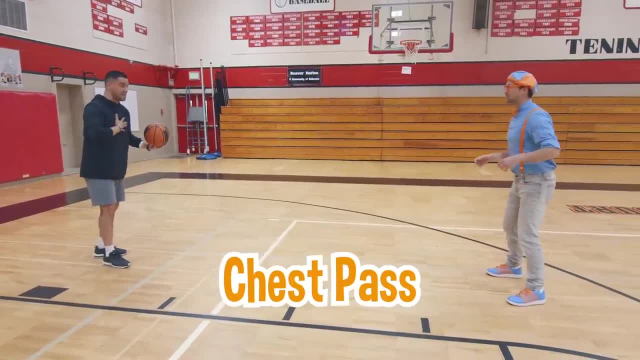 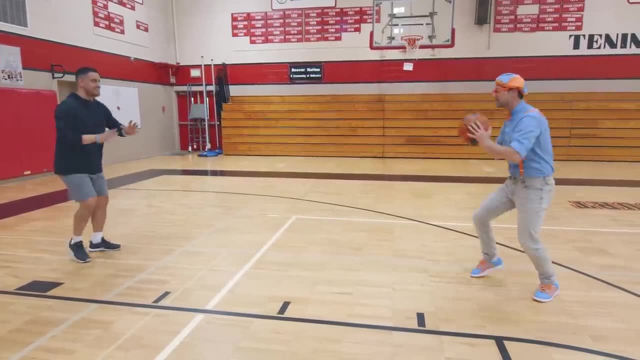 So there's two types of passes. The first one is a chest pass, and I'm going to aim to hit you right in the middle of the chest. All right, Ready, Yep. Oh, did you see that? All right, my turn. 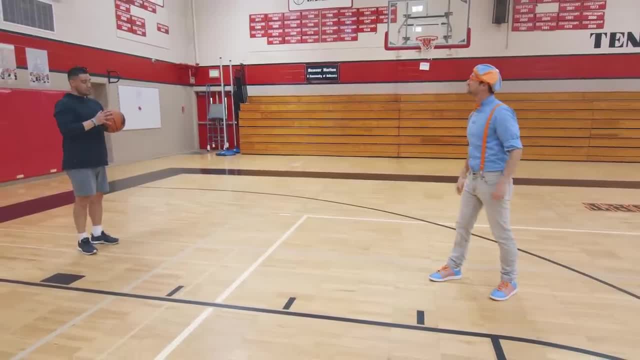 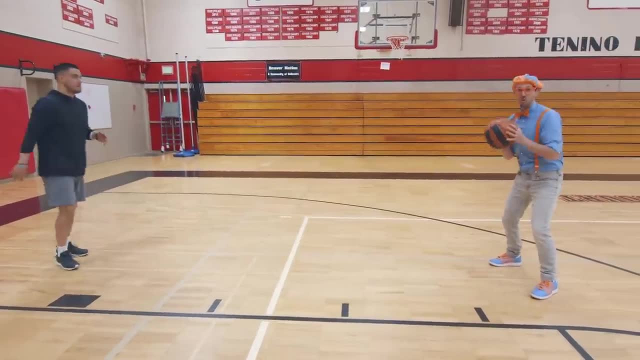 Nice pass, Thank you. The next one we want to work on is a bounce pass. Okay, Same thing, I want to bounce it. so it bounces right up to your chest, Okay, Wow, nice work. All right, here we go. 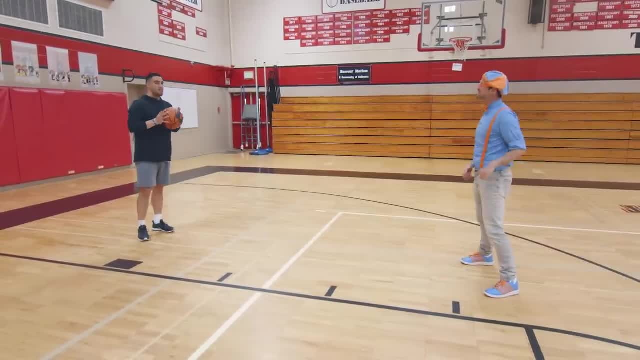 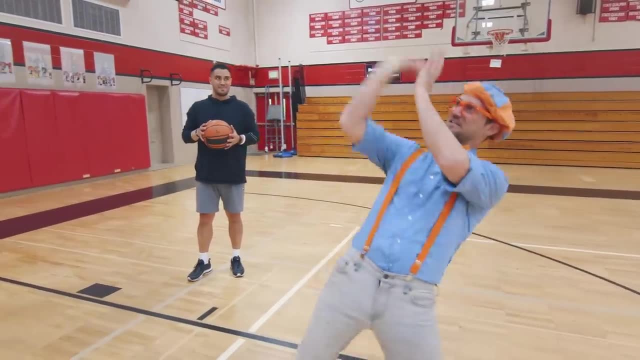 Nice pass. Yeah, thank you. All right. what's next, Then? the next thing that's really important is making sure we know how to shoot. Oh, that's the fun part. Score and points. Yeah, Score and points. To start, we want to probably get as close as we can to the hoop. 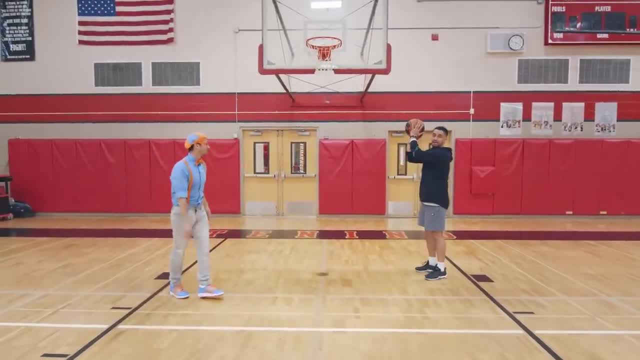 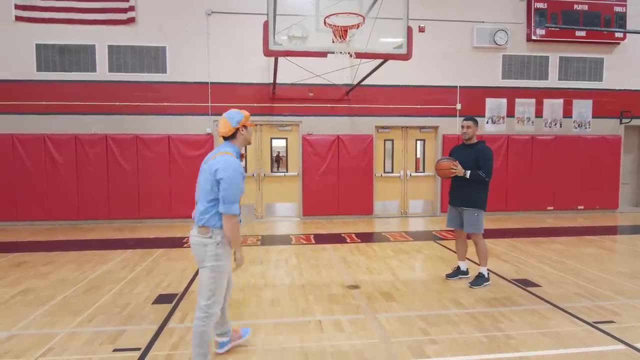 Okay, And when we shoot it, we want to make sure we have a guide hand. Uh-huh, And then your shooting hand And the guide hand helps you control the ball while you're shooting. All right, Just like that, All right. 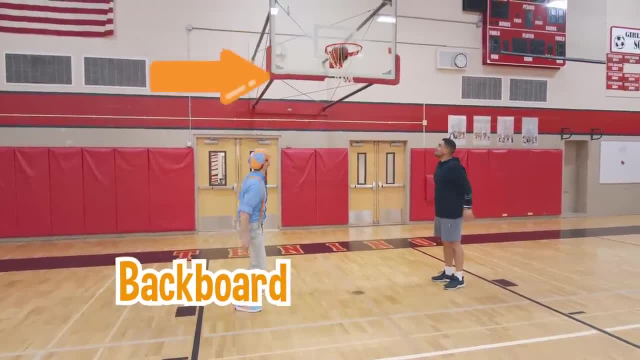 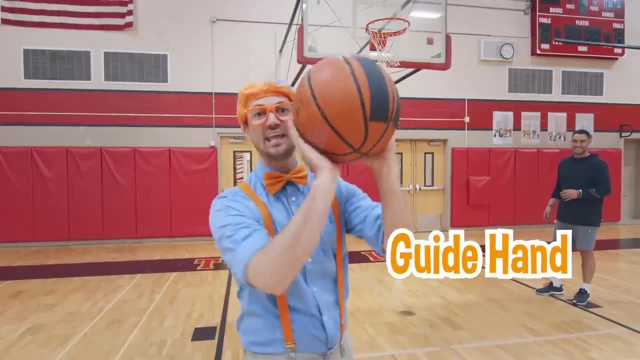 When you shoot it off the glass or the backboard, you want to do it nice and gently, so it falls right in the hoop. Perfect, You try it. All. right, here we go. I'm going to use my guide hand and my shooting hand to score a point. 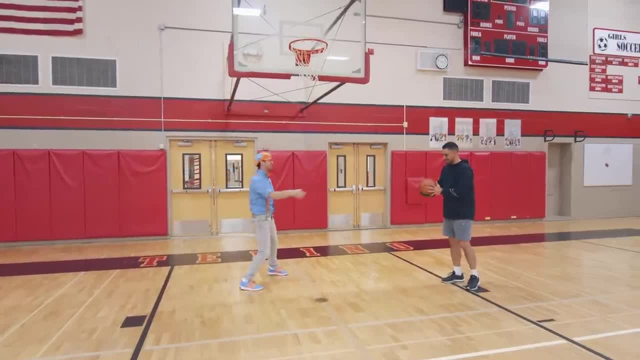 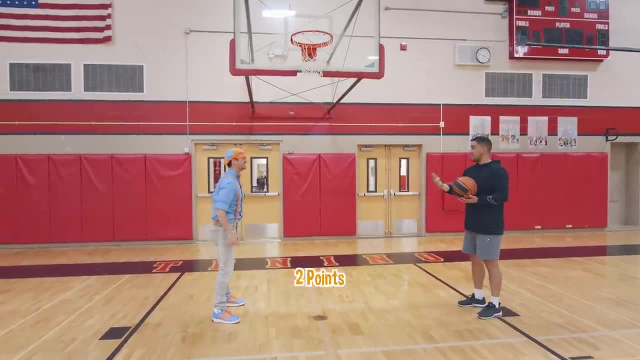 Yeah, Nice shot. Blippi, Nice shot. Thank you, All right, So now what do you do? So when you shoot a layup, it's worth two points. Okay, Part of us having good teamwork is I can pass you the ball. 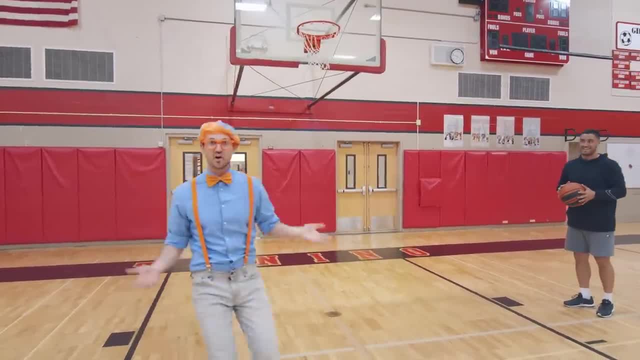 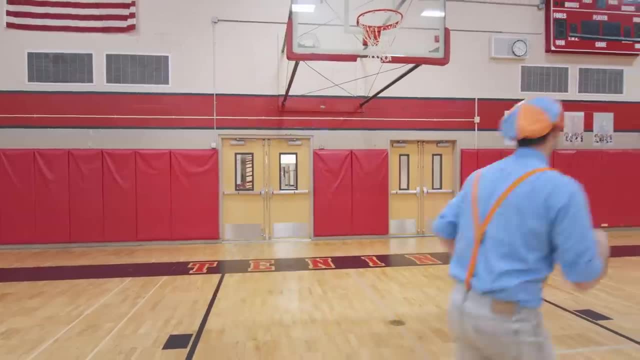 and you can shoot a layup. You want to try it? Yeah. So since I know how to receive a pass and shoot, maybe he and I can use some teamwork to score a point. Let's do it, Okay, All right. 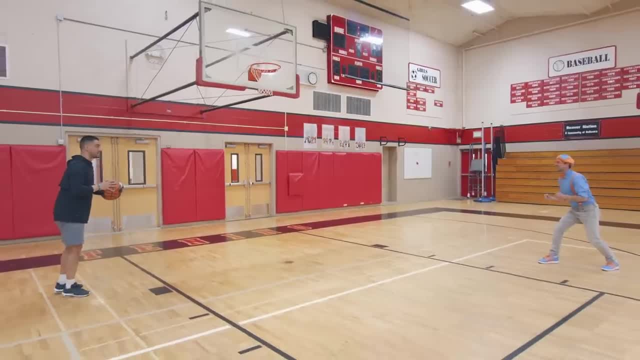 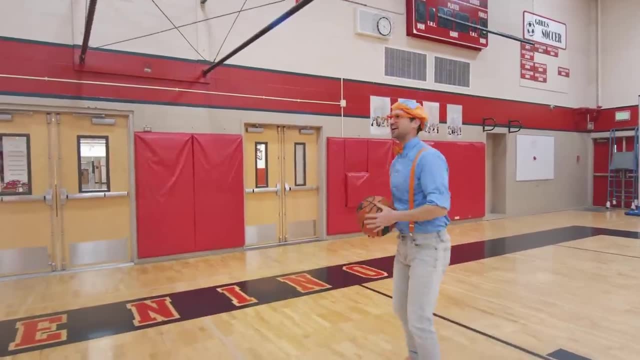 I'm going to give you a bounce pass. You take your layup off the glass. All right, Are you ready Go Woo-hoo. Yeah, We did it. Nice shot. Do you want to try? I'll try it too sure. 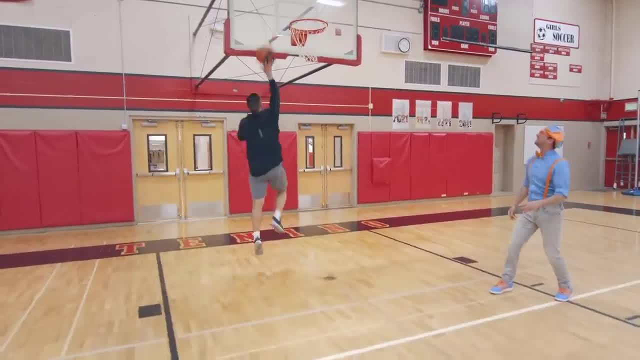 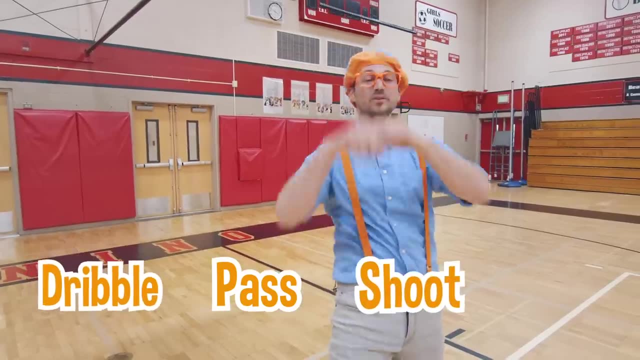 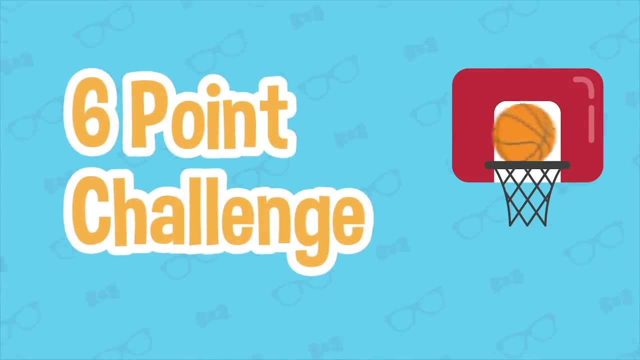 Ready, Here we go. Yeah, We did it. Wow, We just learned how to dribble, pass, shoot and do a layup. Now it's time for a challenge. Help, It's time for the six-point challenge. 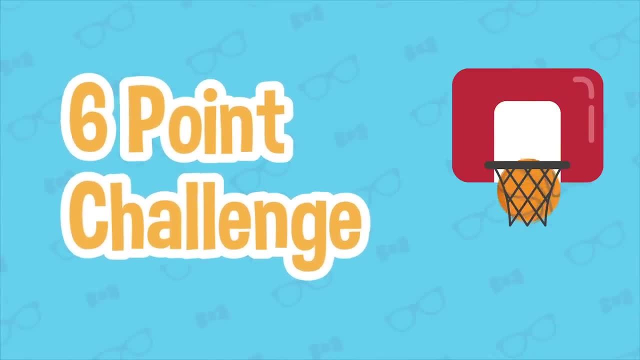 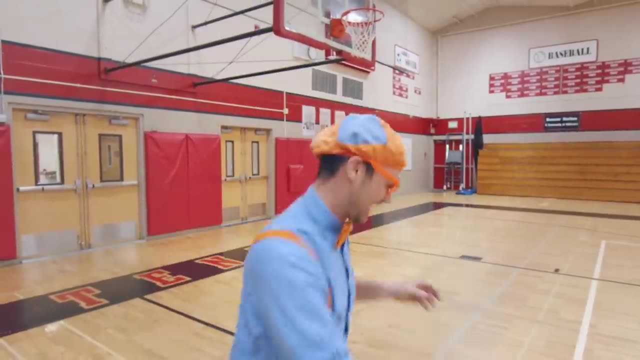 Will Blippi score six points for the basketball medal. Count along? All right, Here's the challenge. Let's do this. Are you ready? I'm ready, All right, Here we go. Yeah, Good shot. Thanks, Blippi. 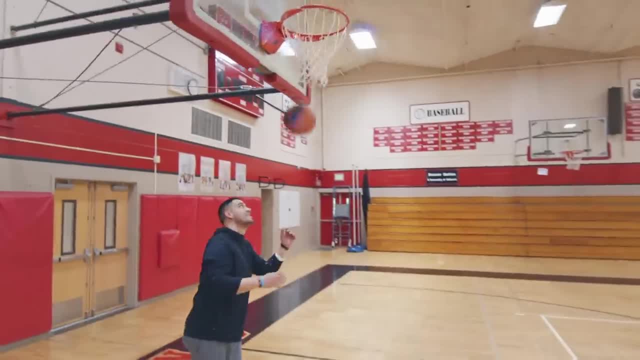 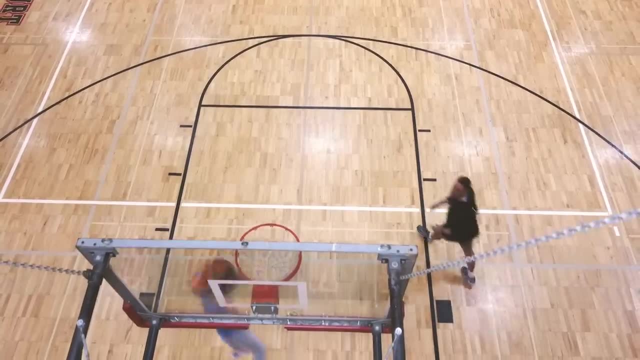 That was awesome. All right, My turn Ready. Yep, Here we go. Woo-hoo. Nice shot, Blippi. Did you see that? Whoa, All right, Here's for a mid-shot. Here you go. Nice shot, Blippi. 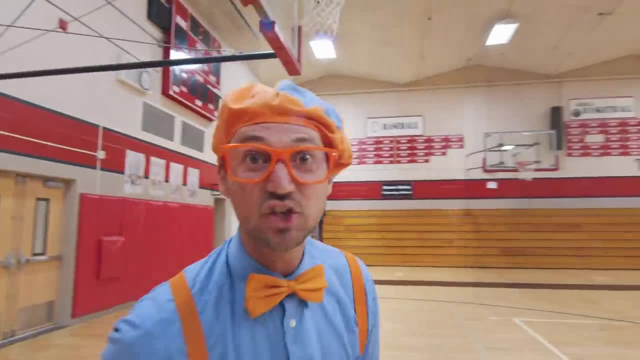 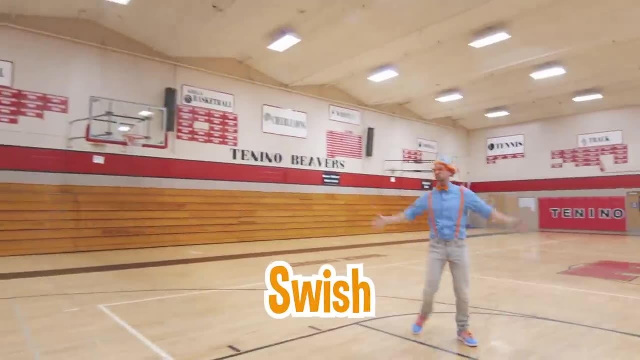 Did you see that? Whoa, All right, Here's for a mid-shot. Here you go. All right, Here we go. Here we go. Whoa, That was a perfect swish. All right, You ready, Yep. 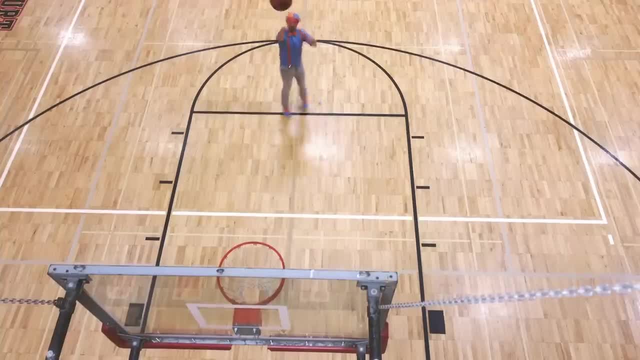 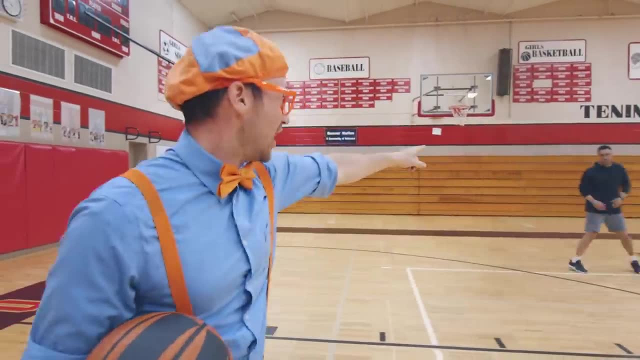 I'm ready, Your turn. Here it comes. Yeah, Nice shot, Blippi, Woo-hoo. All right, Now for a three-pointer. Here he goes. Ha-ha, Whoa, That was amazing. Your turn, Blippi. 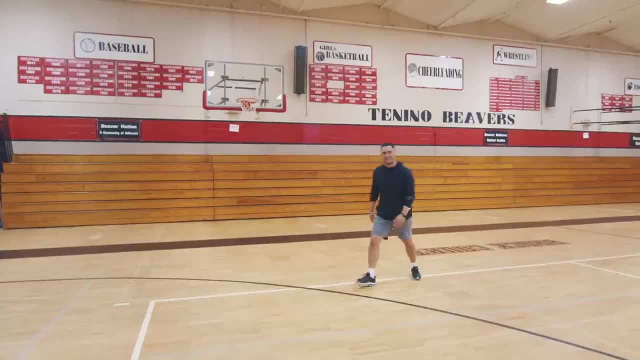 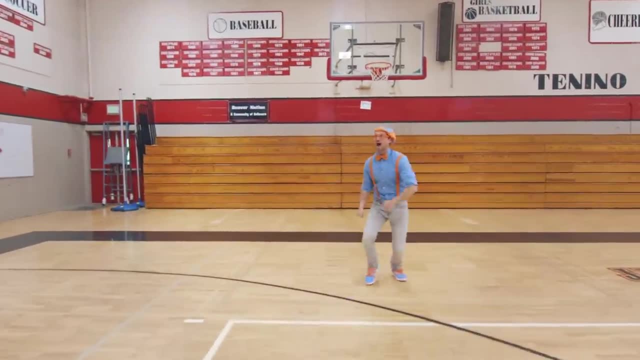 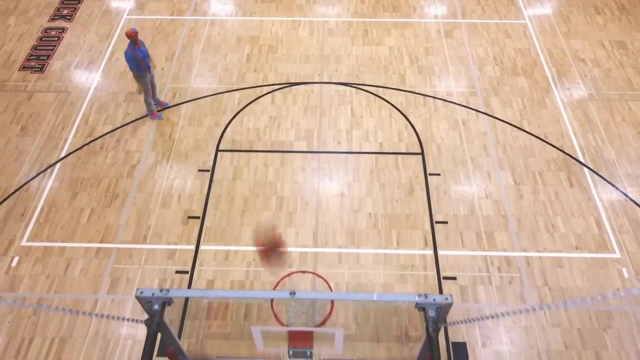 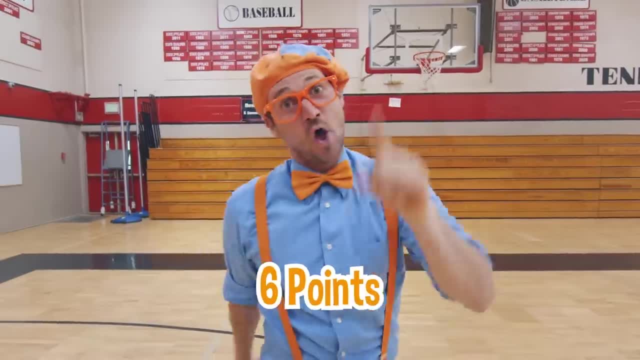 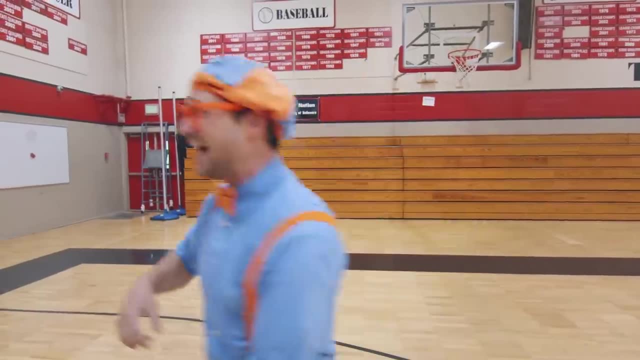 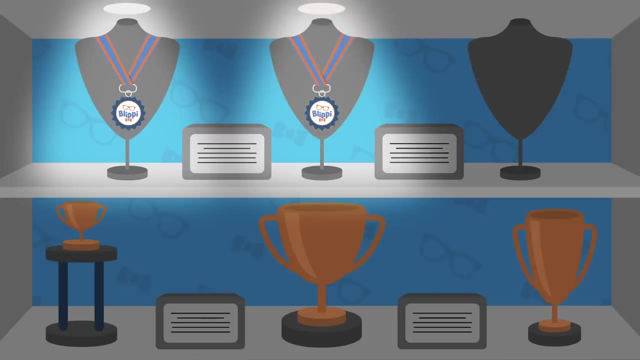 Nice shot. Thank you so much. That was six points: One, two, three, four, five, six. Whoa, That was so many High five. He did it. Basketball takes a lot of teamwork, All right, With some training and a whole lot of practice. 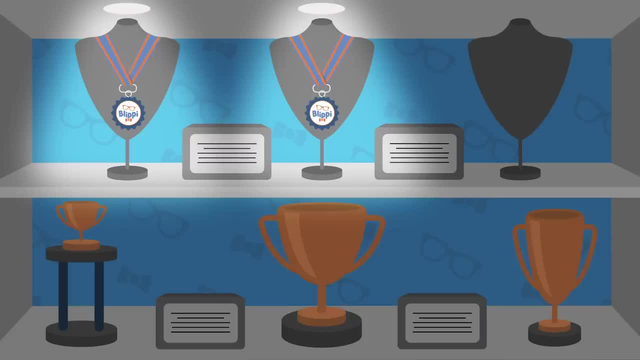 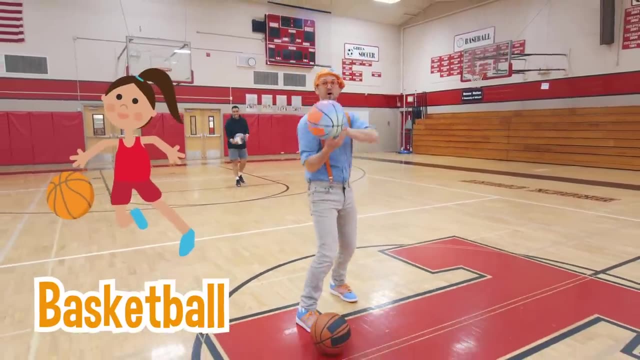 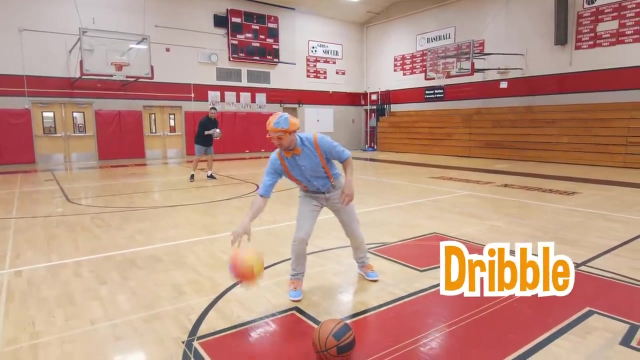 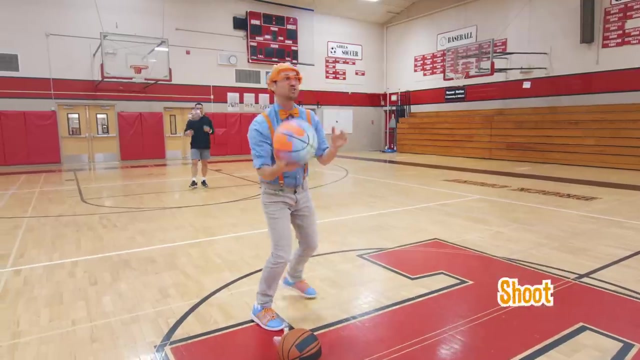 you can become a champion. Way to go, Blippi. Wow, That was so much fun learning how to play basketball together. Whoa, Do you like basketball? Yeah, I do too. Whoa, It was so much fun learning how to dribble, how to pass and how to shoot. 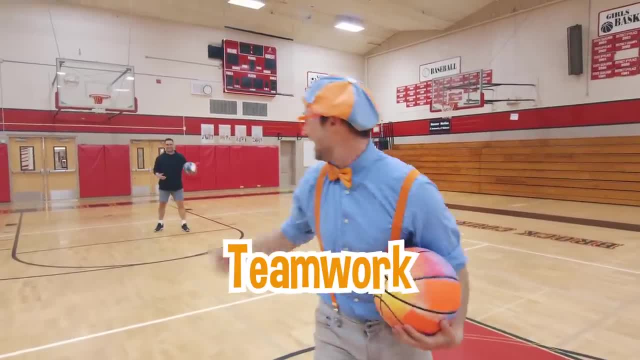 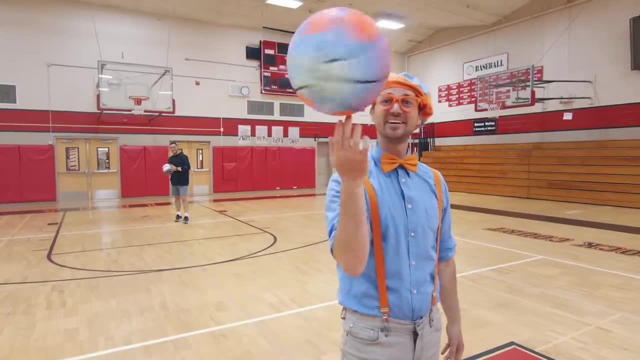 And all of that We learned with a lot of teamwork. Yeah, Thank you so much. Coach Joe, Thanks for coming. Blippi, Yeah, Wow, Do you like basketball? I do too. It's great, But before I go, I probably don't need this basketball anymore. 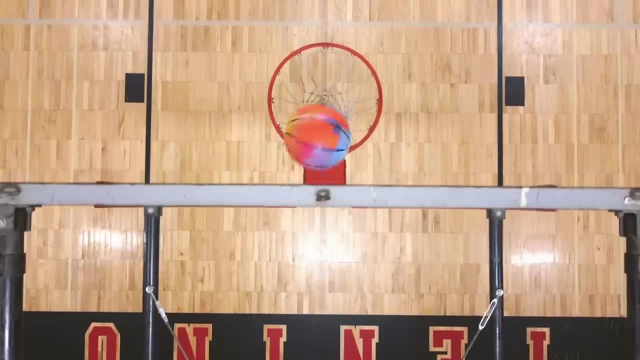 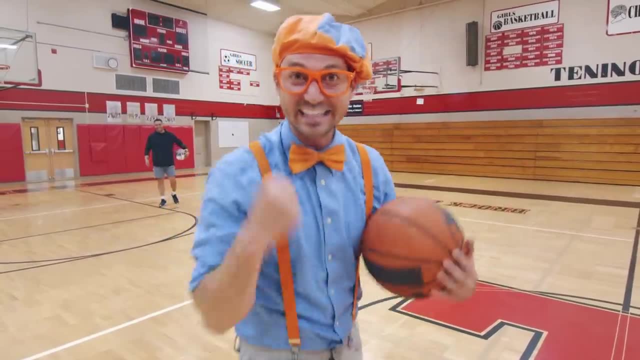 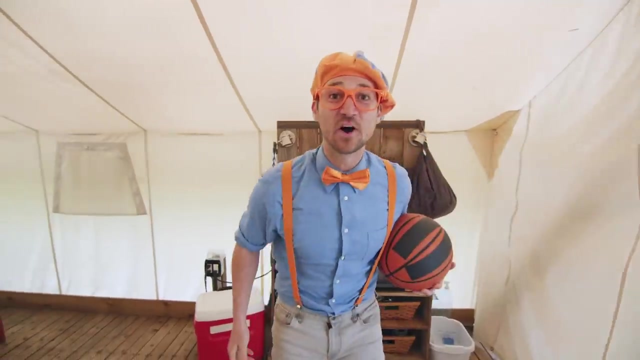 See you later. basketball: Yay, Yeah, That was awesome. All right, Let's head back to the Summer Games tent. Let's go. Ha-ha, Woo-hoo, Ha-ha. Wasn't that so much fun playing basketball together? 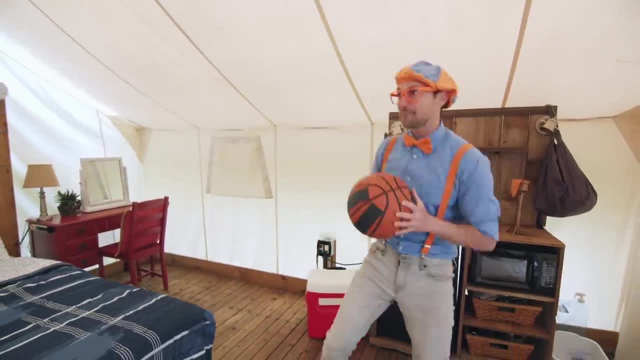 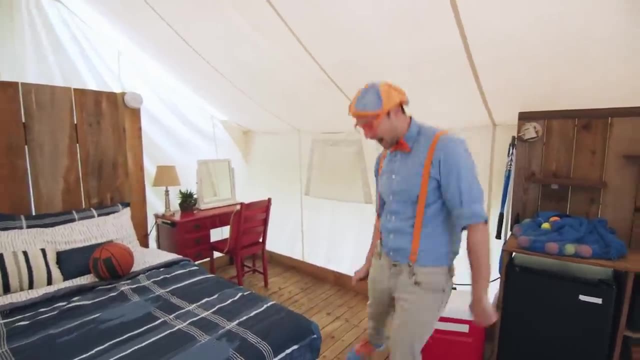 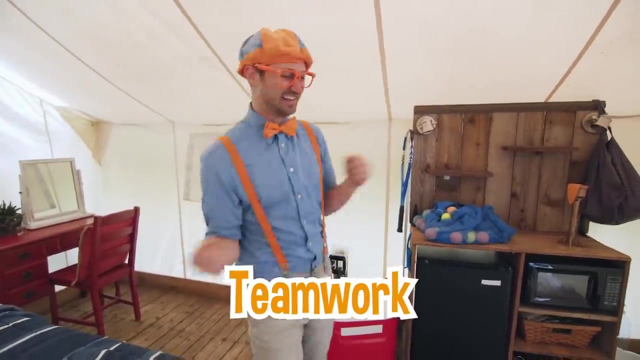 Yeah, It was awesome dribbling the ball together, passing it to a teammate- Yeah. And swishing some threes- Yeah. My favorite part about basketball is working with a teammate- Yeah, Teamwork, It's so much fun, Ha-ha. 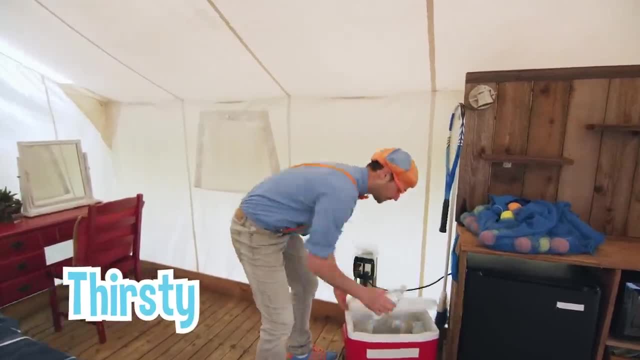 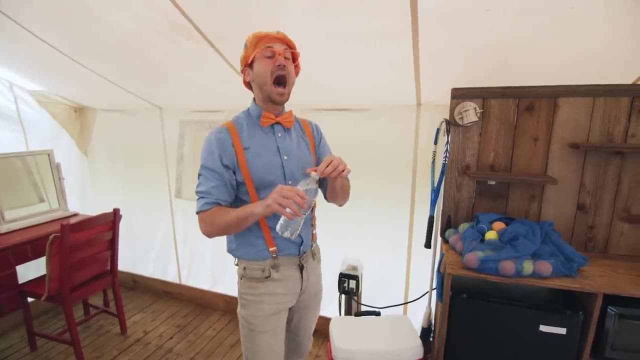 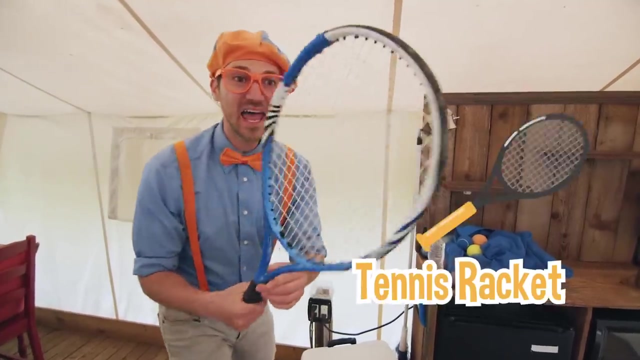 Oh, I am sure thirsty. I should probably get some water. It's really important to stay hydrated while you're playing sports And being active. Ha-ha, Whoa, Look at what it is. Yeah, A tennis racket. Wow. 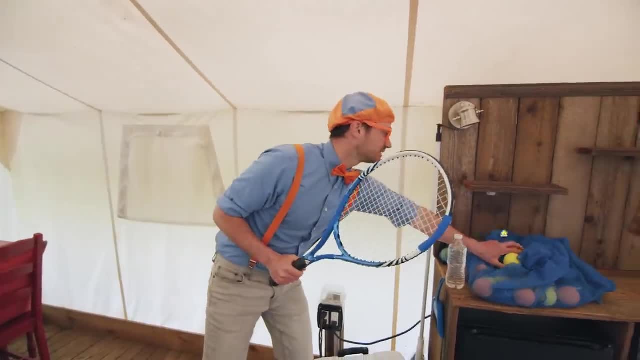 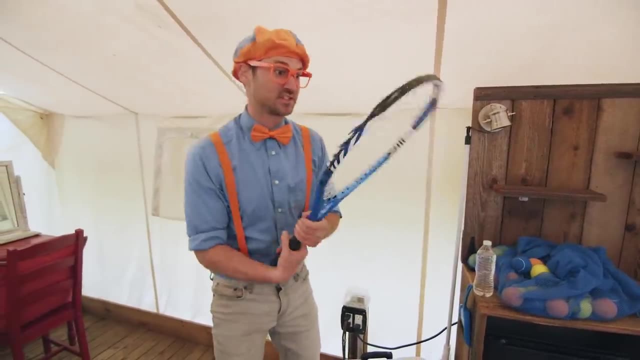 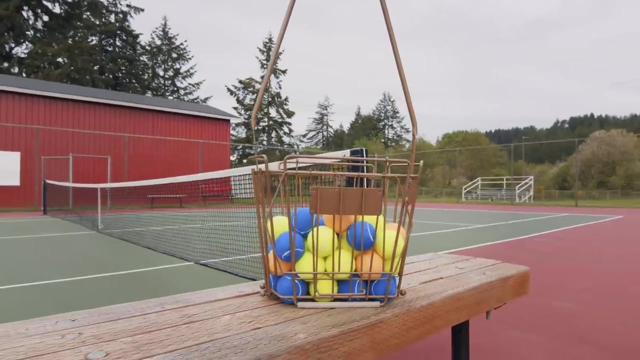 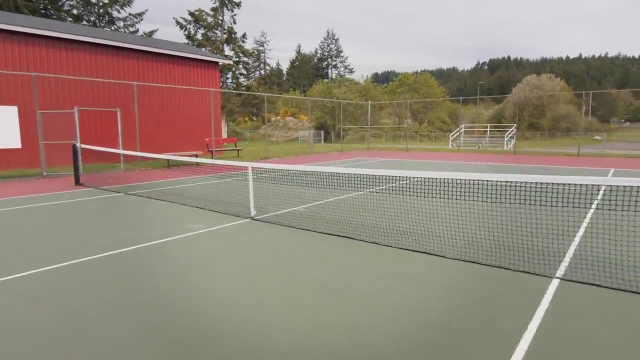 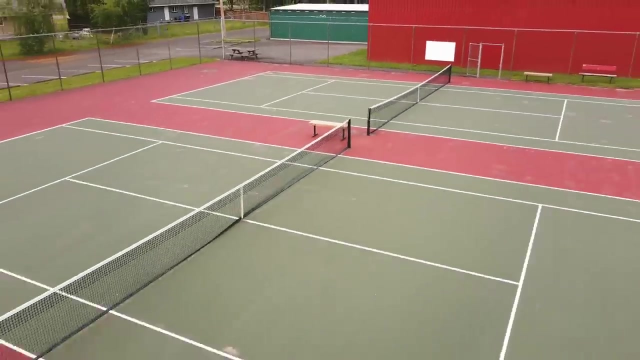 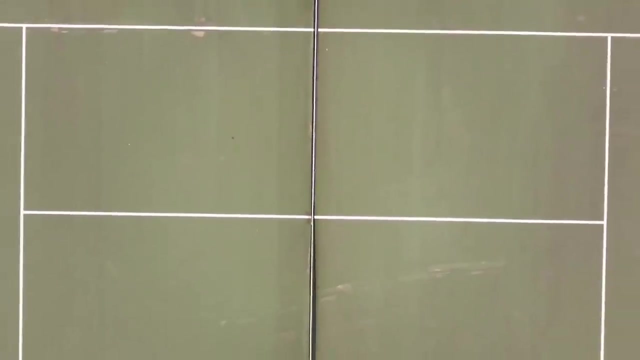 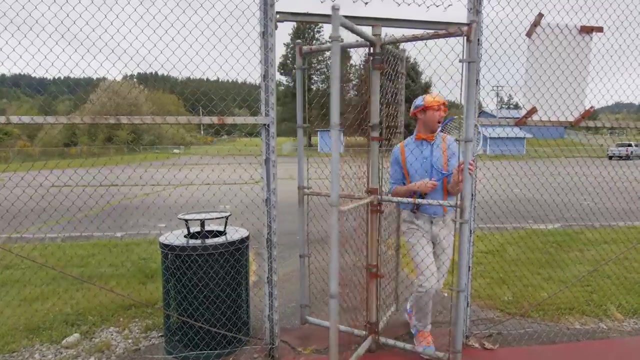 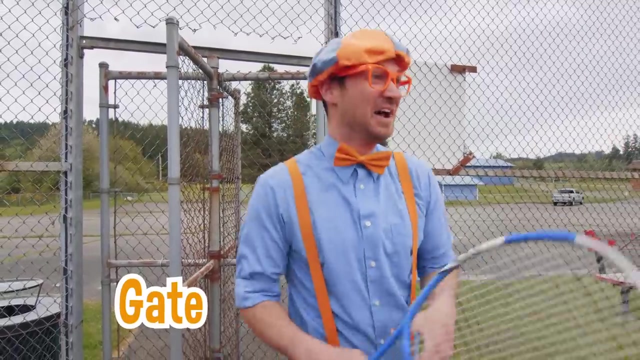 Tennis is also played on a court. And look Some tennis balls, So colorful, Ha-ha. Hey, Maybe we should go to a tennis court And play and learn some tennis. Yeah, Ha-ha, Ha-ha, That's one squeaky tennis gate. 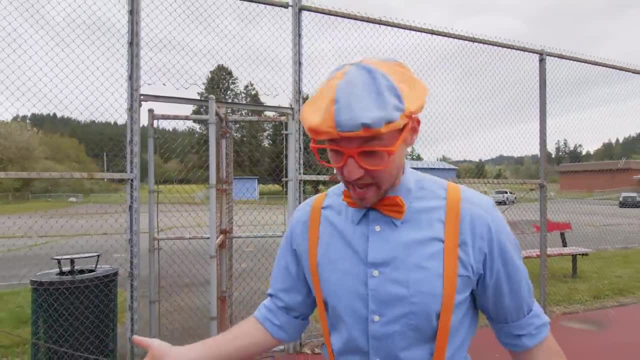 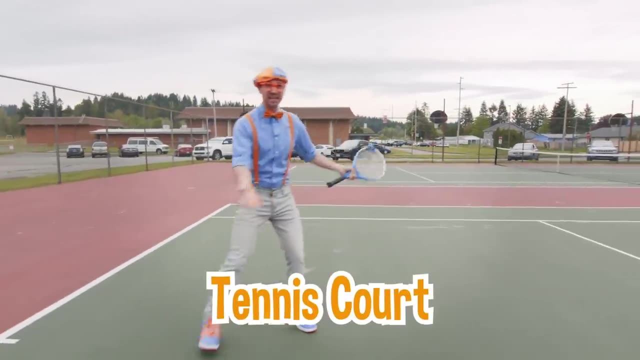 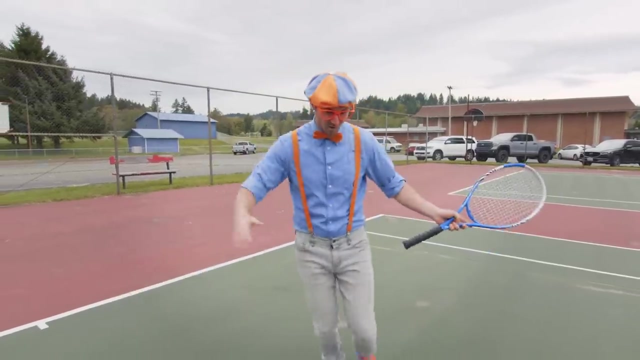 Well, hey, check it out. Right now we are at the tennis court and this is awesome. I love tennis, and check it out this tennis court. yeah, it's just like basketball: Basketball and tennis are both played on a court. whoa, look, my feet grip to the ground. 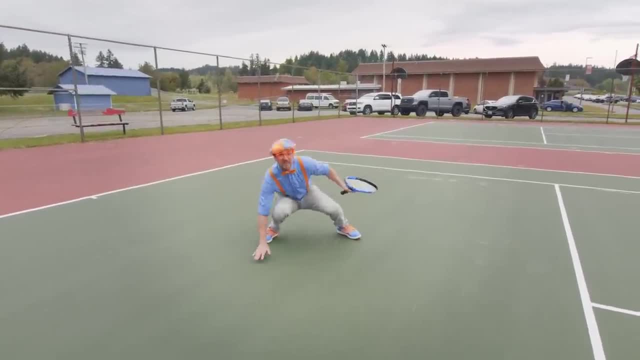 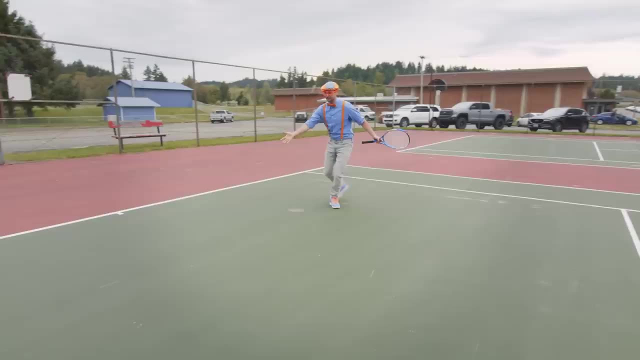 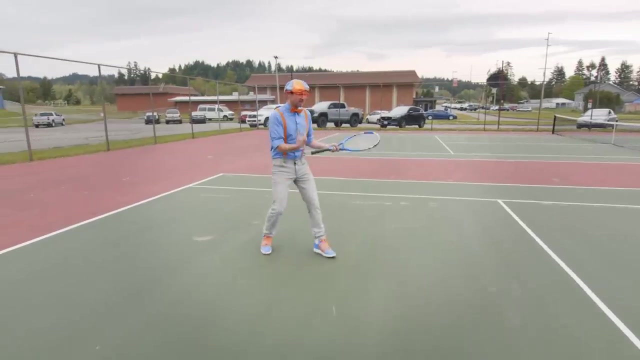 super good, because this tennis court is made with special material, so then you don't slip and slide. Whoa, look at this. do you see what shape this is? whoa, this is a rectangle. This is part of my side of the tennis court. oh, and here's another rectangle over here. 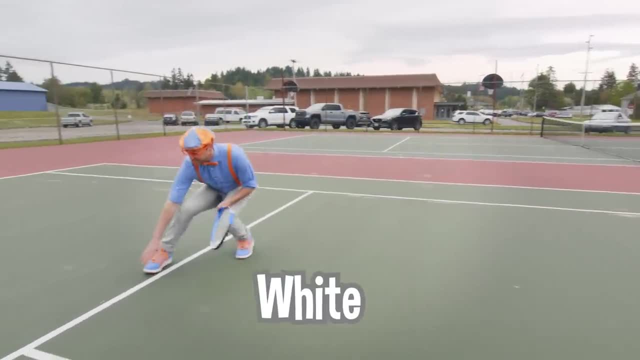 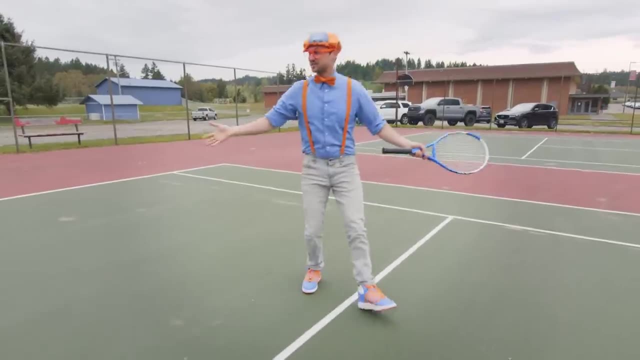 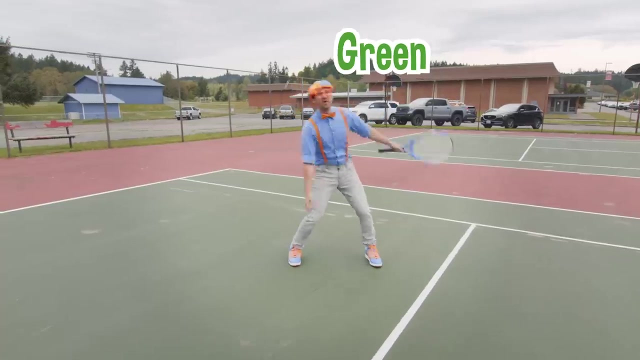 whoa, And do you see these white lines right here? This is what separates the boxes of the tennis court. whoa, do you see what color the main part of the tennis court is? yeah, it's the color green. oh, and outside of the tennis court, 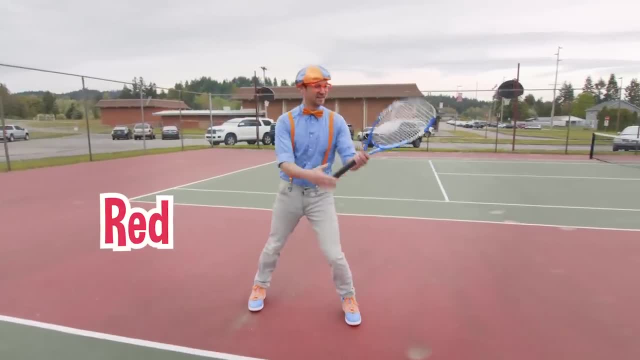 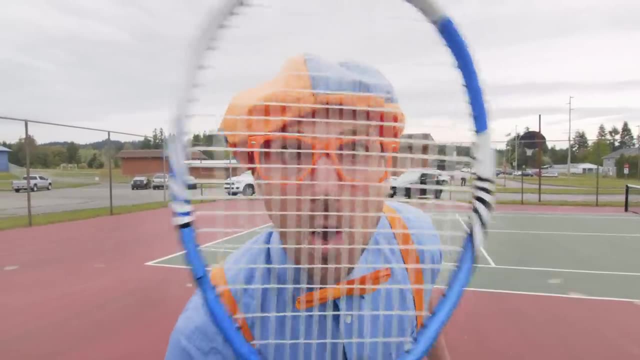 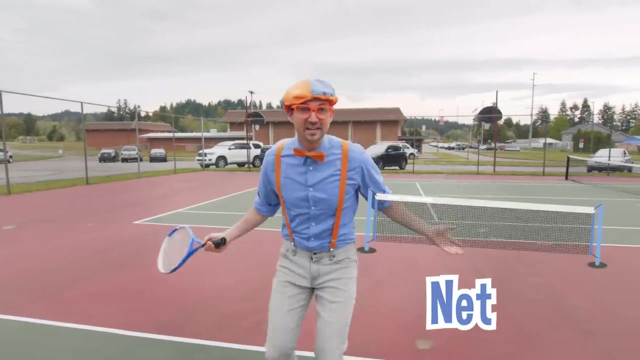 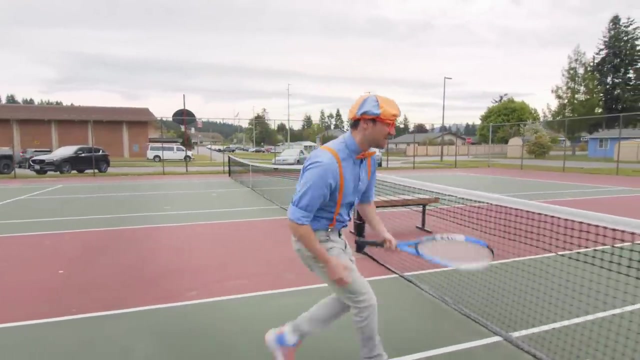 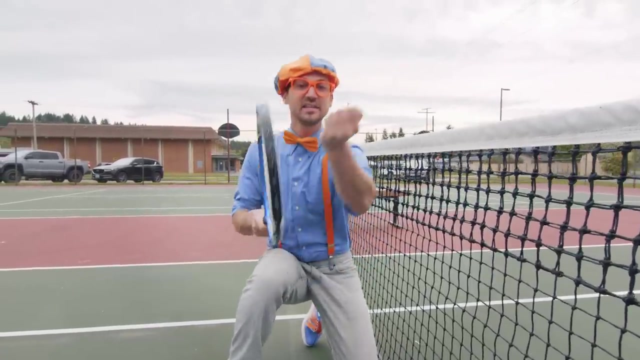 yeah, it's the color red. do you see what I'm holding? do you know what this is? yeah, this is a tennis racket. Hello, yeah, this is what you use to hit the ball over the net. oh, speaking of the net, come on, wow, check it out. whoa, this is the net and this, like I said, you hit the tennis ball. 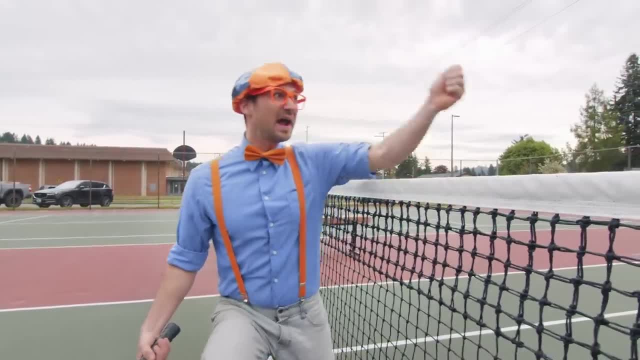 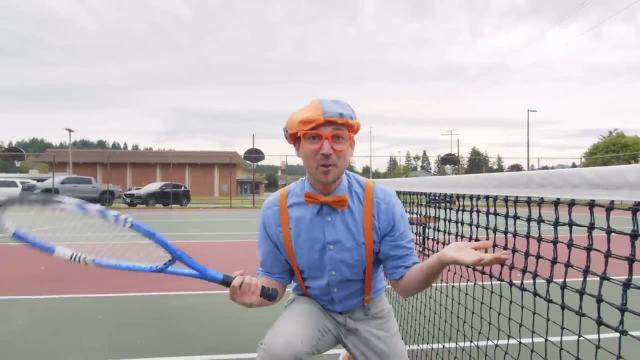 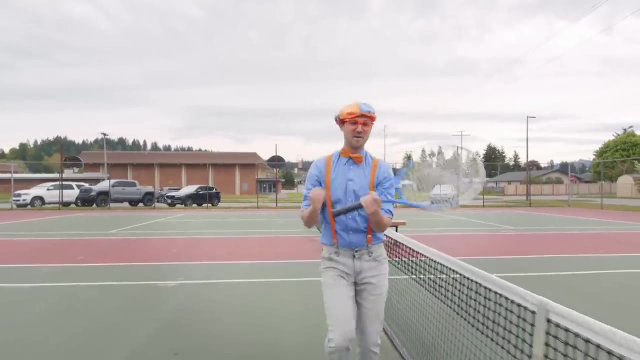 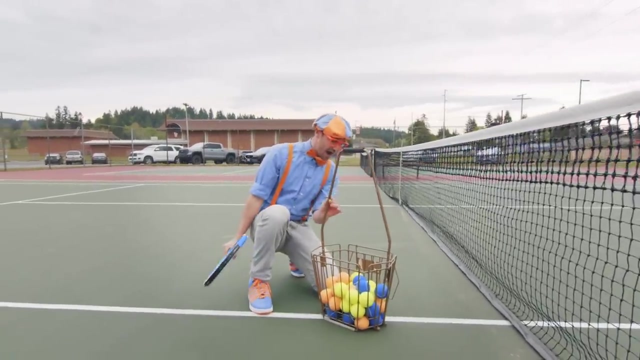 over the net and then your opponent hits it back, and then you hit it back, They hit it, They hit it back, you hit it back, and that is called a rally. oh, I am so excited to play some tennis, but I think we need a ball. whoa, speaking of tennis balls? wow, look at this. 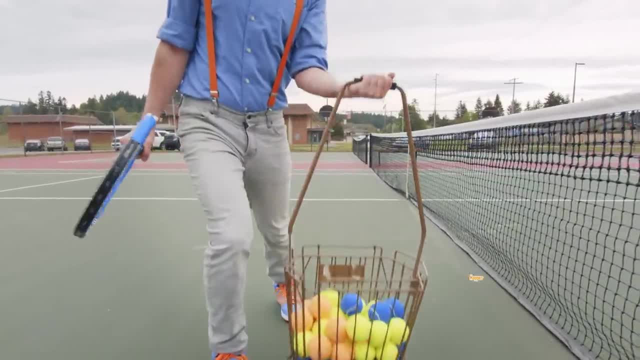 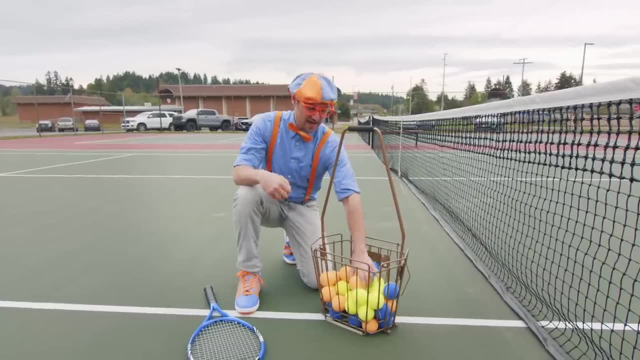 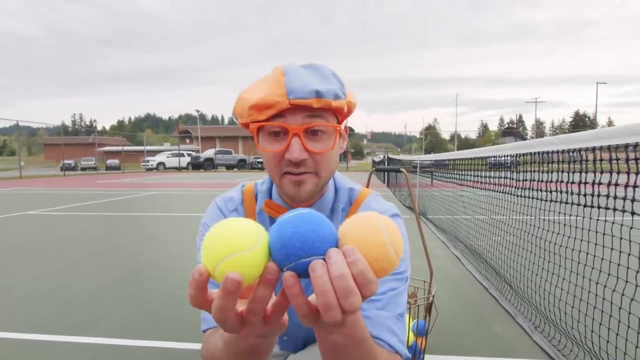 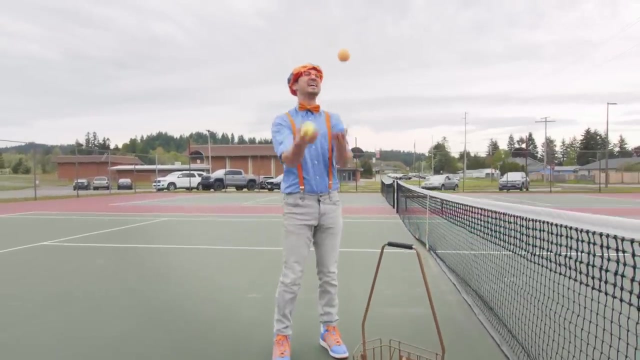 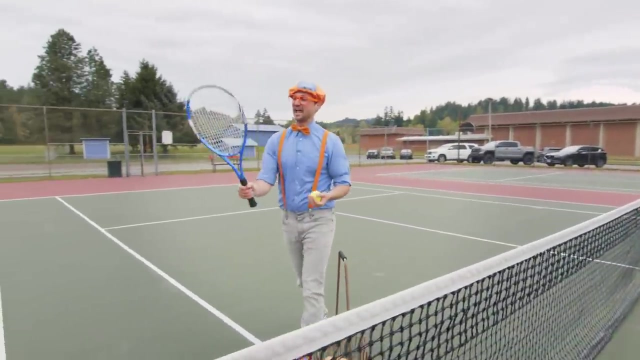 this is called a hopper. whoa, it is so heavy. look at how many tennis balls are in here. wow, Wow, We have so many. but hey, we have 3 colors of tennis balls. what colors are these? yeah, we have yellow, blue and orange. yeah, I love tennis. all right, let me take the yellow ball. 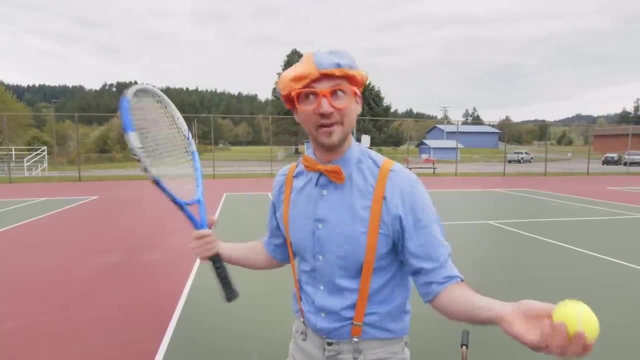 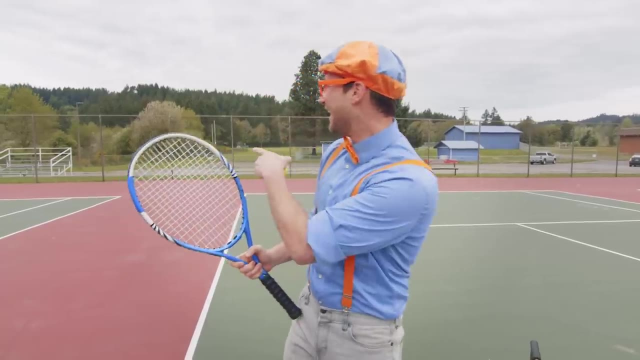 and I should probably play some tennis. wait a second. even though I'm one of the best tennis players in the whole wide world, I love tennis. That doesn't mean I don't need lessons. Oh, hey, look, It's my coach. 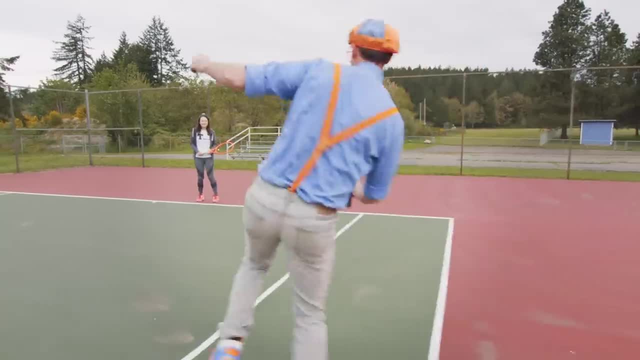 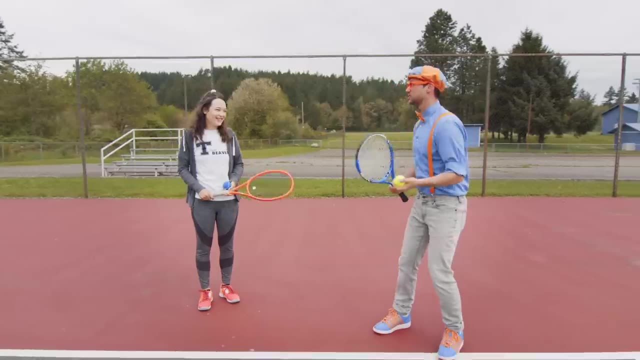 We should go say: hi, Hey, Coach Whitney, Hi Blippi, How are you, I'm doing well, How are you, I'm good? Well, hey, I was thinking you and I could play a game, But first I think we should have some tennis lessons. 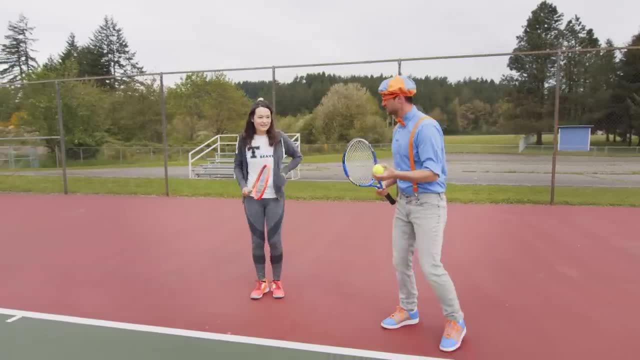 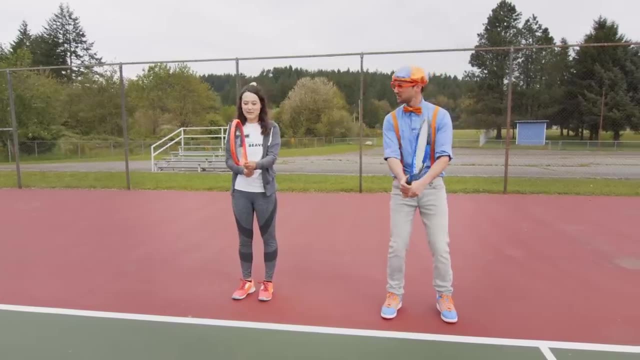 Will you teach us some Absolutely Okay? All right, let's start with a forehand. Okay, So there's two types of hits in tennis. The first is a forehand, And you want to hold the racket with your hand that you write or draw with. 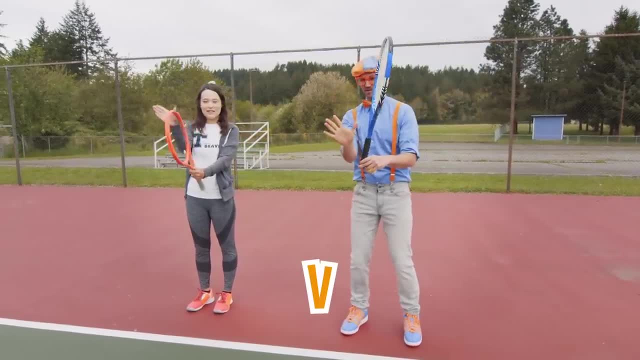 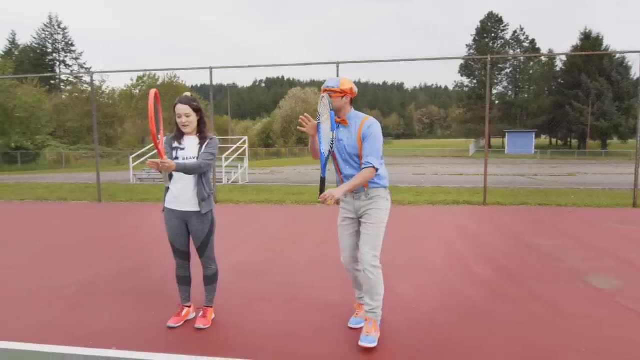 Oh, that's this hand, So I like to make a V first. Okay, And I start up here at the top of my racket. All right, a V, And I'll start at the top of the racket And work your way all the way down to the bottom. 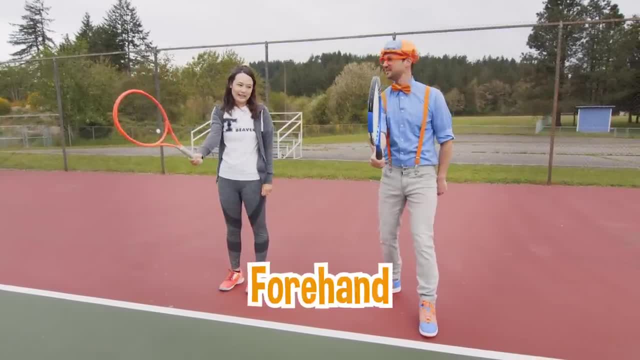 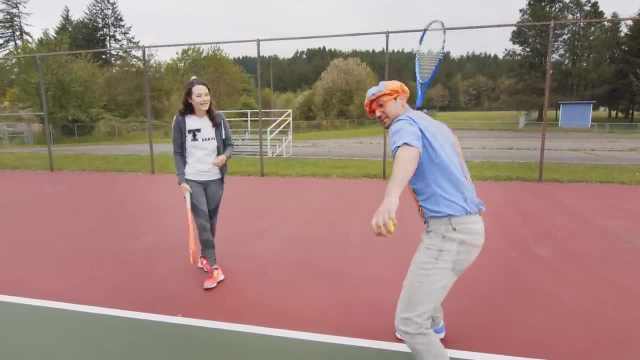 And then grip it like a handshake. All right, And that's your forehand grip. Perfect From there. when the ball comes to you, you swing back and forward. Oh Okay, Like this Pretty close, I'm so good. 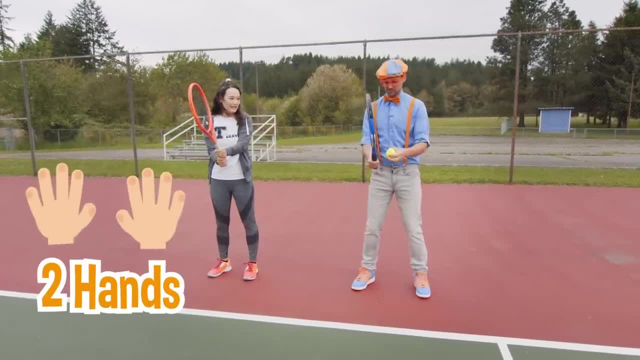 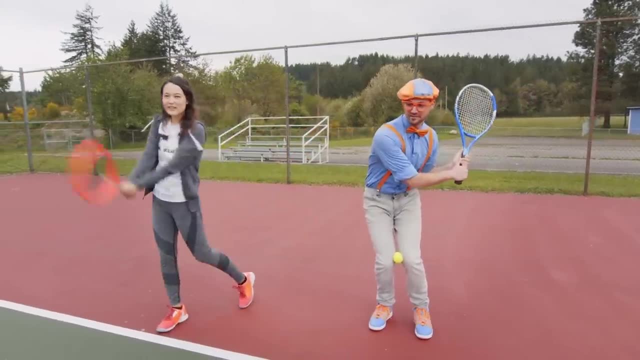 All right, And then a backhand. You want two hands on the racket this time, Okay, And you're going to go to this side of your body, the other side. Step forward and swing just like a forehand, Perfect, Okay. 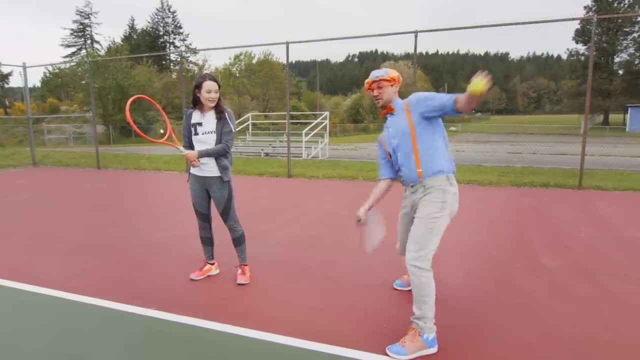 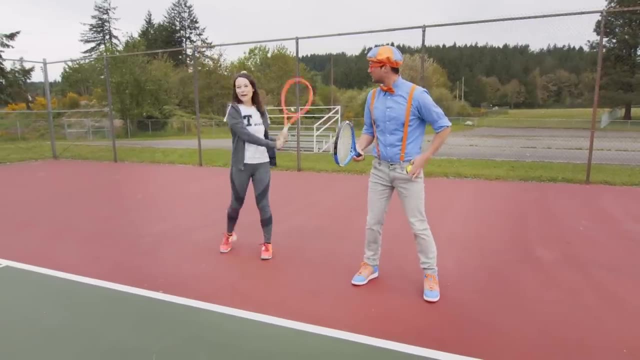 So this was a backhand And this was a forehand. So what do I do with my feet? Well, you always want to be ready for a forehand, A forehand or a backhand. So you want your feet nice and wide, like your shoulders. 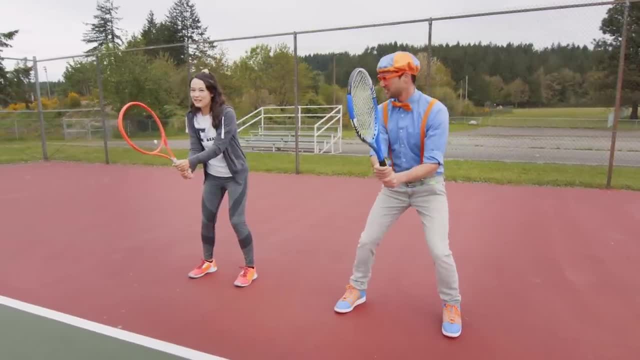 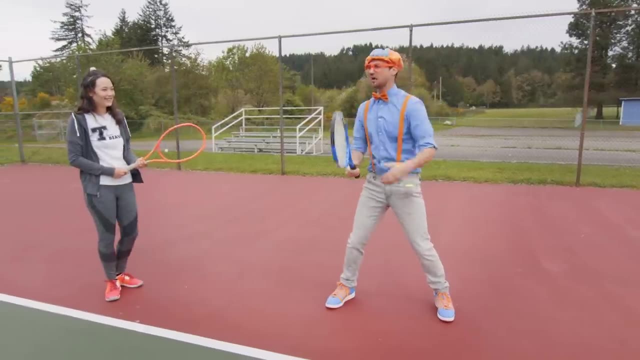 All right. And from here we hold the racket in the middle of our body. Okay, So we can go either way. Oh, how do I look Perfect, All right. Well, how do we start the rally? Well, we have to start with a serve. 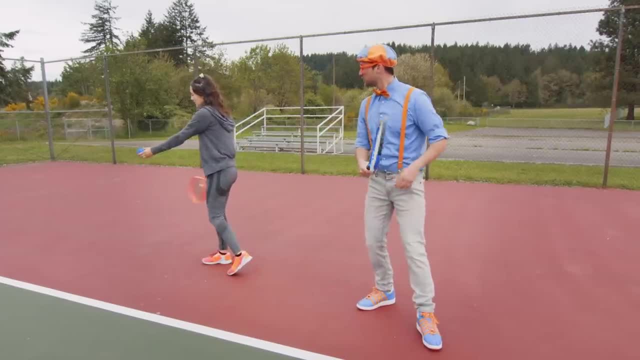 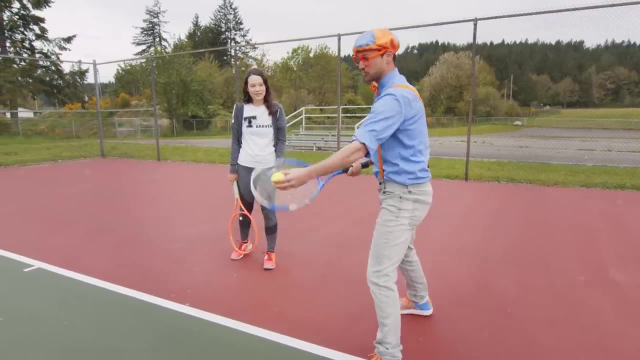 Okay, And you can do two types of serves. You can start with an underhand serve where you hit down here kind of like a forehand: Okay, This is an underhand serve. Okay, And what is this? The other type of serve? 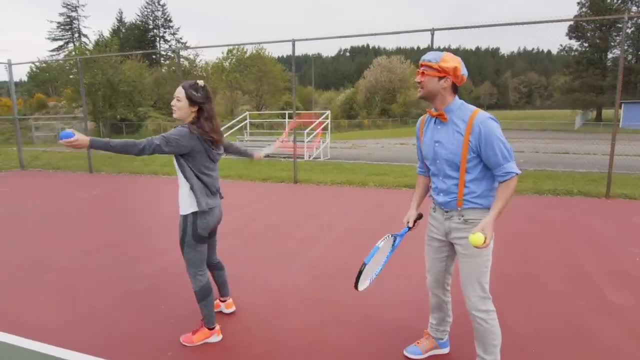 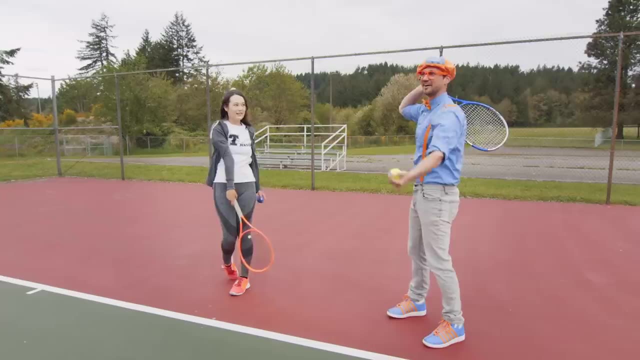 An overhand serve. In an overhand serve, you have to point your elbow to the sky up here behind your back, Okay, And you toss the ball high up in the sky and swing to hit. Oh, that sounds pretty fun. 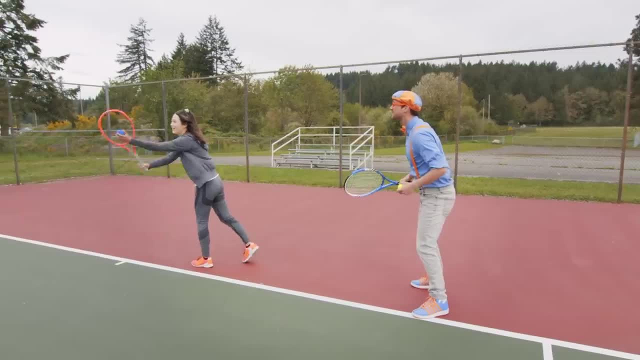 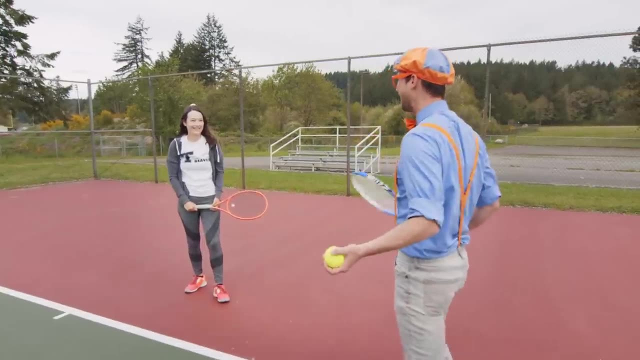 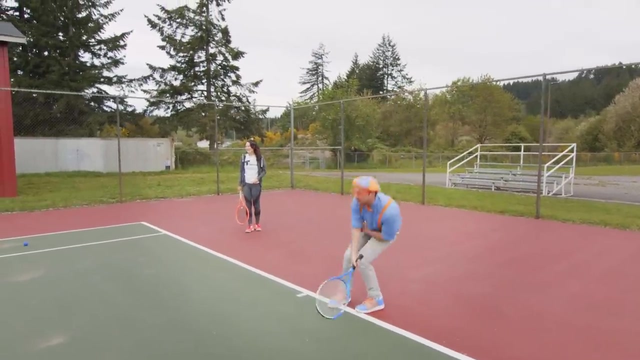 Will you show us Absolutely: Whoa, that was awesome. Can I try? Sure, All right, Here we go. Yeah, That was awesome. Well, hey, maybe you and I should do a challenge. Yeah, we should play a game. 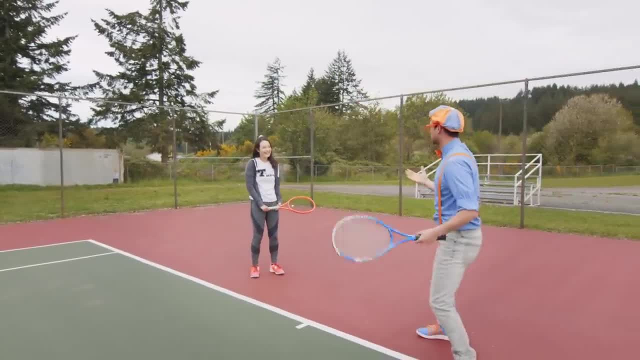 Are you up for it? I'm absolutely up for it. All right, Let's go. It's the five rally challenge. Can Blippi hit five shots back to his coach for the tennis medal? Let's count, Let's go, Let's go. 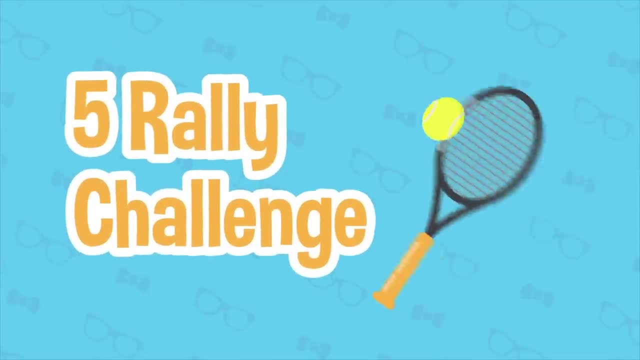 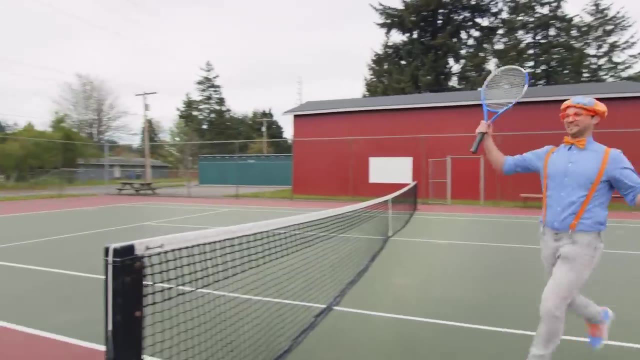 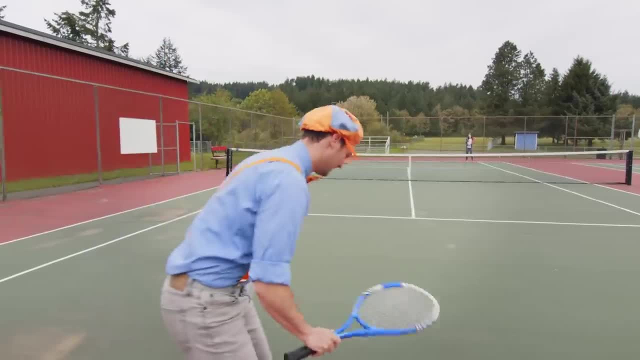 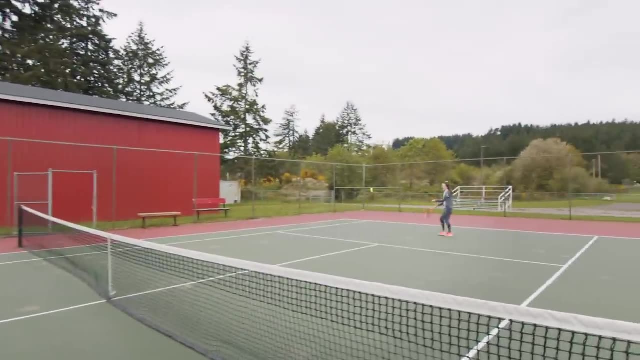 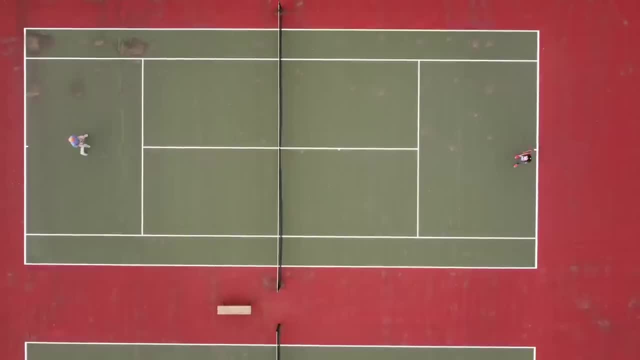 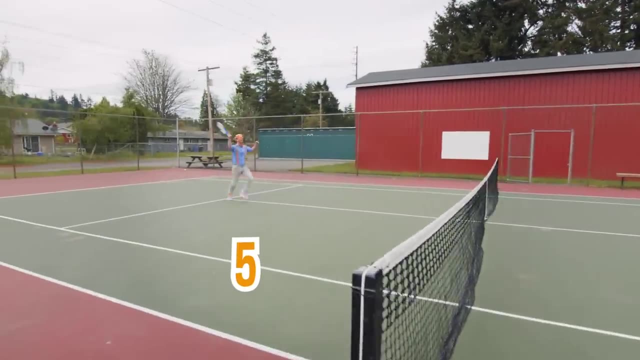 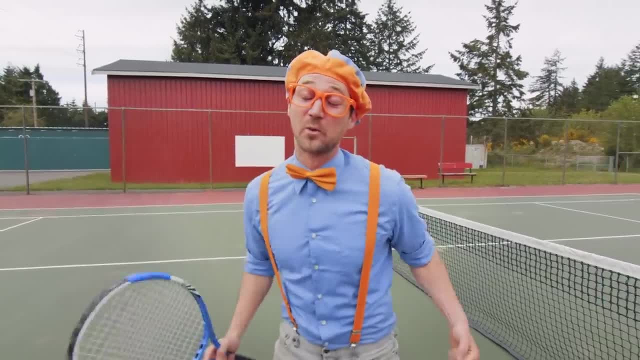 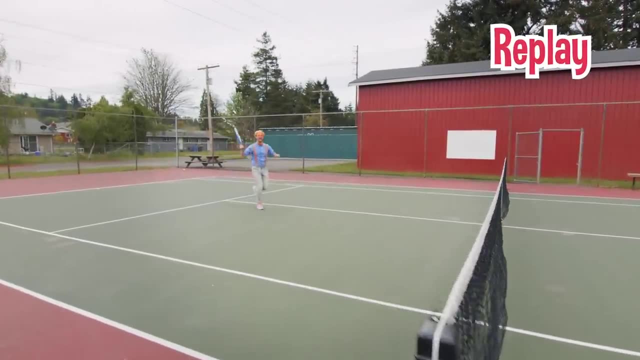 It was great. Let's see how many they hit. All right, let's keep going. Let's do all of them. Ooh, Ooh, Ooh. What a great rally Blippi had with his coach. Check out that forehand. 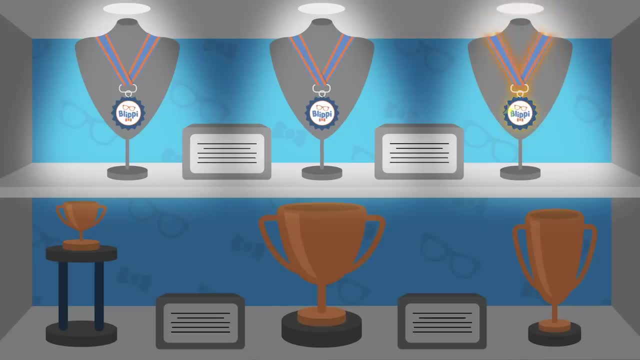 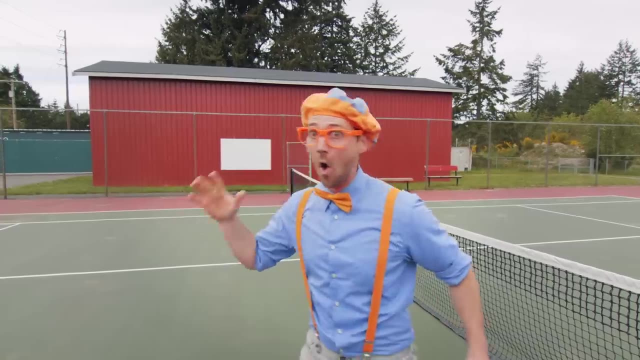 Blippi earns his third medal. Tennis takes a lot of hard work, but with some training and a whole lot of practice you can become a champion. Oh, do you hear that? Yeah, sounds like the closing ceremony is going off. I think we should go. 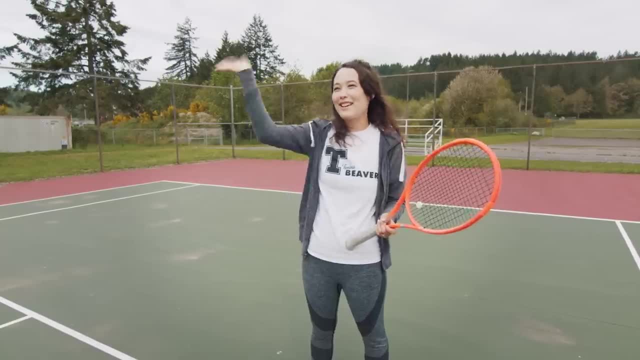 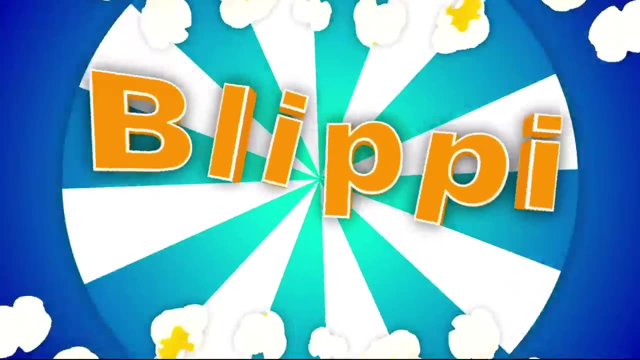 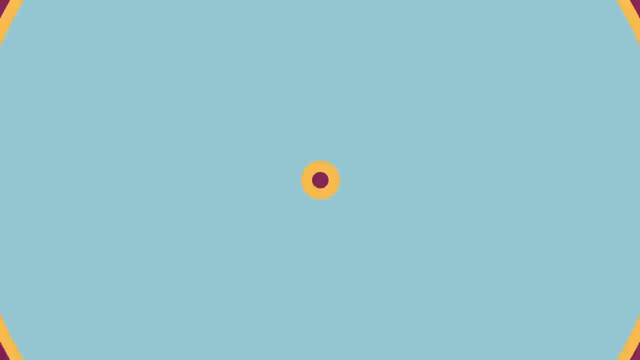 Well, hey, I gotta go Nice playing with ya. See you later, Blippi. See you later. So much to learn about. it'll make you want to shout: Blippi. Teamwork is dreamwork. We play together. 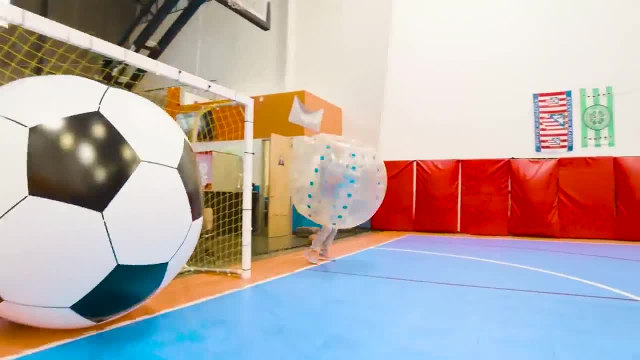 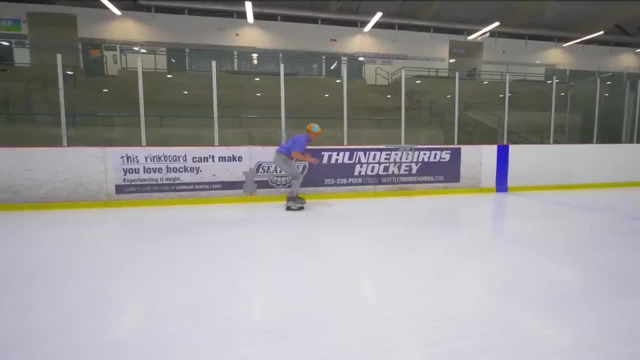 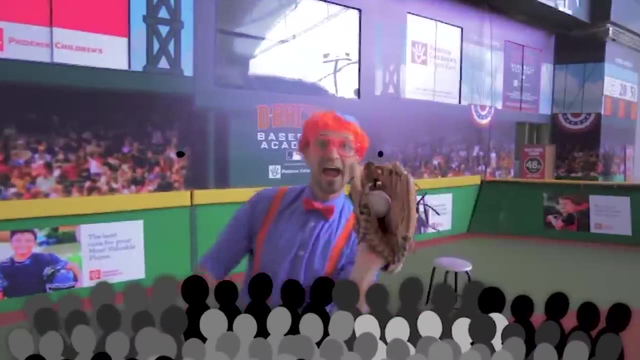 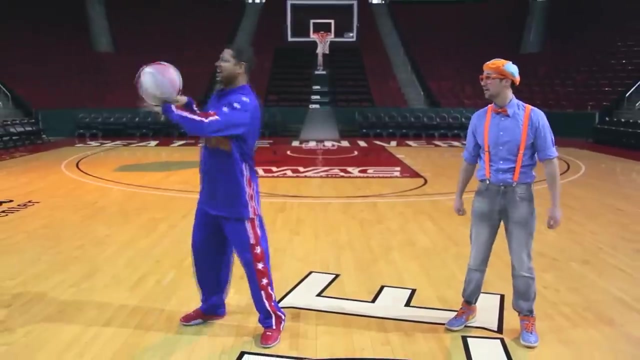 Run, pass and score. Make friends forever. Teamwork is dreamwork. We play together. We play together, Run, pass and score. Make friends forever. All for one And one for all. Together, we can win it all. 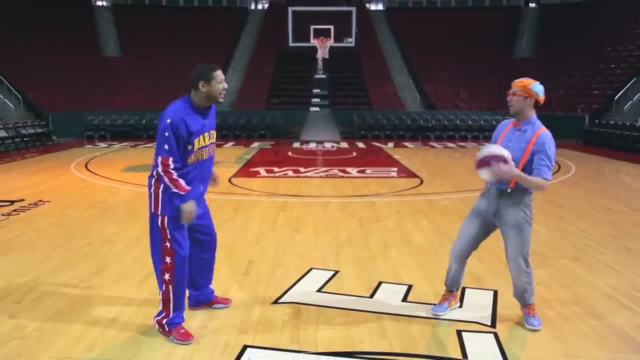 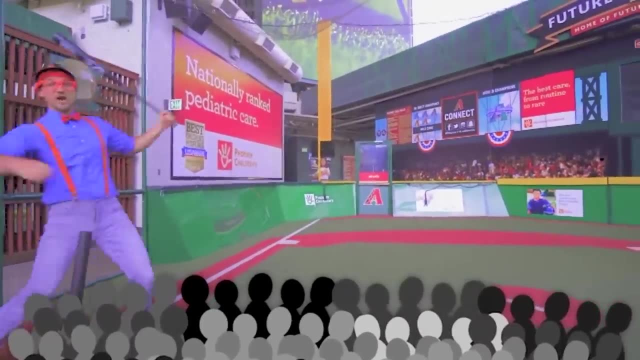 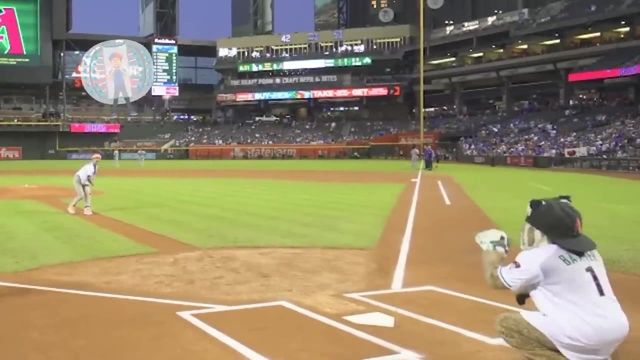 Dribble the ball and pass some more Kick and score. that's what we got in store. Up to bat. it's time to swing. It's a home run. We all win. Are you a team player? Let me hear you cheer. 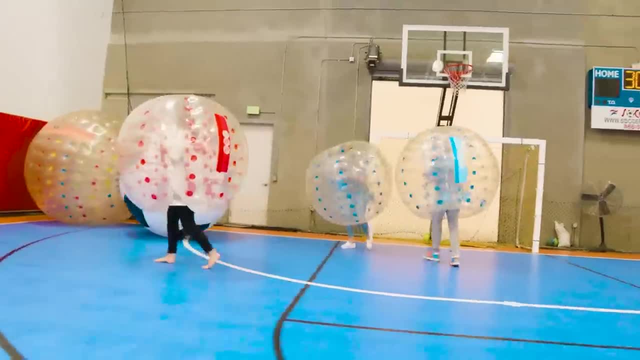 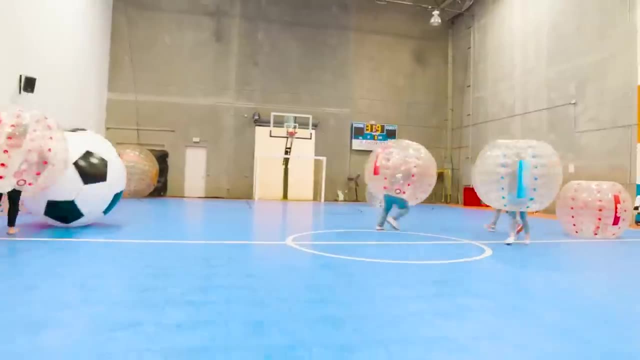 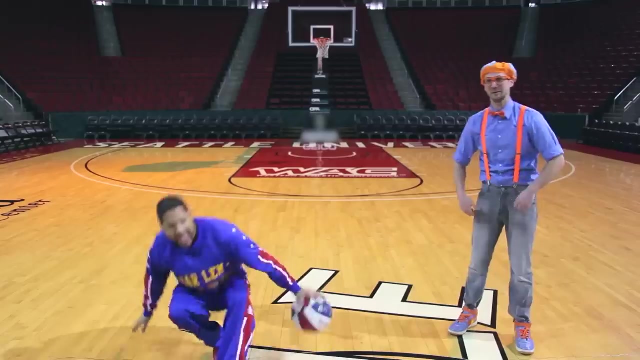 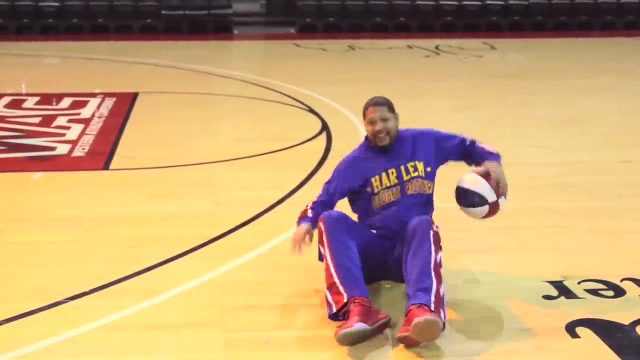 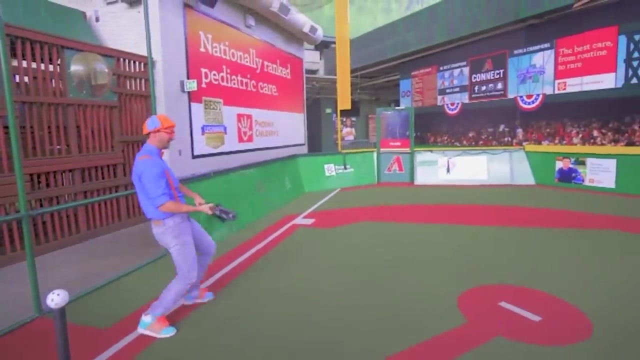 Are you a team player? Let your friends take the wheel. Teamwork is dreamwork. we play together, Run, pass and score. make friends forever. Teamwork is dreamwork. we play together, Run, pass and score. make friends forever. All for one and one for all. 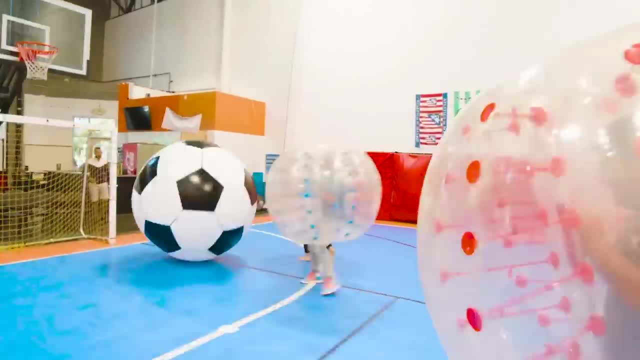 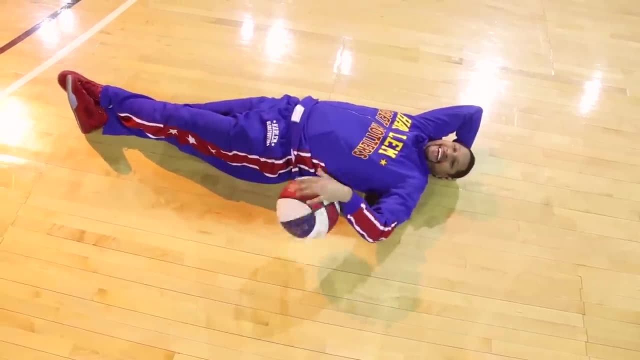 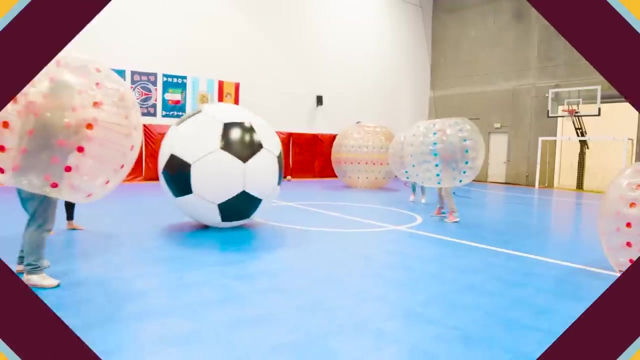 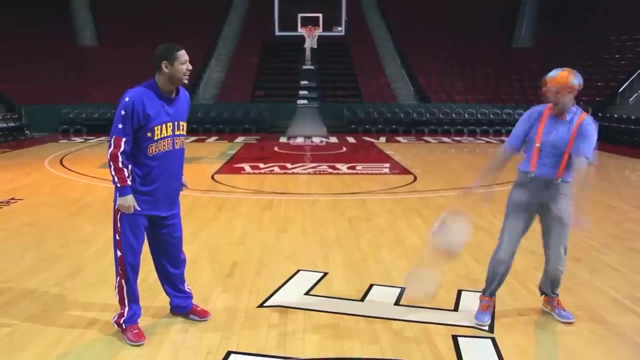 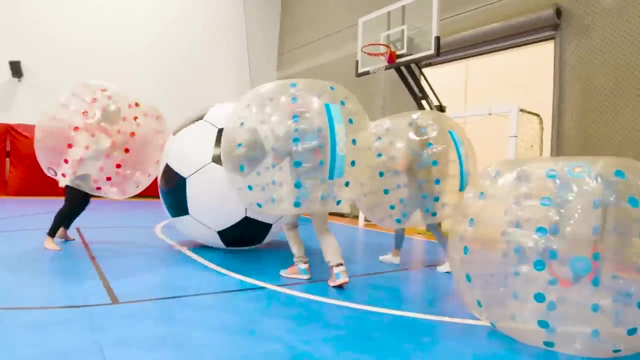 Together we can win it all. Sports take skills. you learn something new, Practice and practice is what you gotta do. Teamwork is dreamwork. we play together, Run, pass and score. make friends forever. Teamwork is dreamwork: we play together. Dreamwork is dreamwork: we play together. 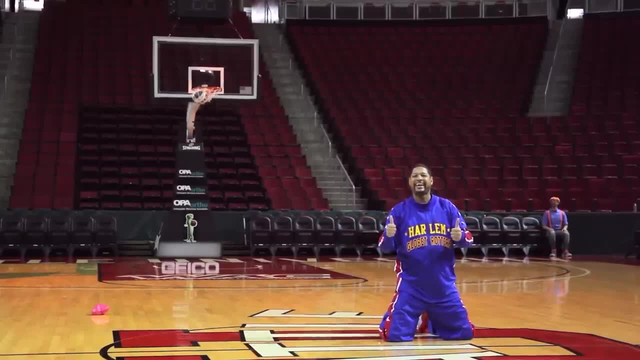 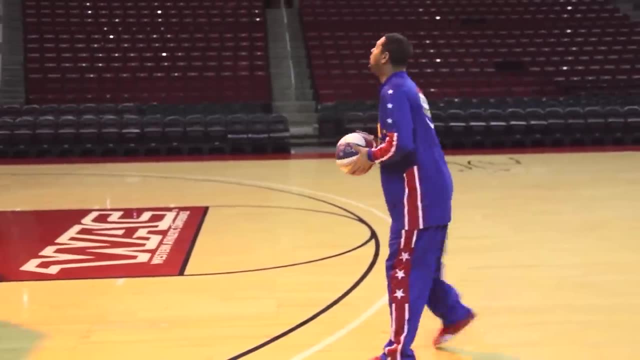 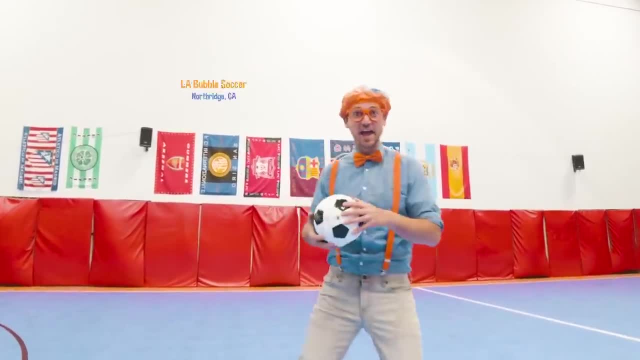 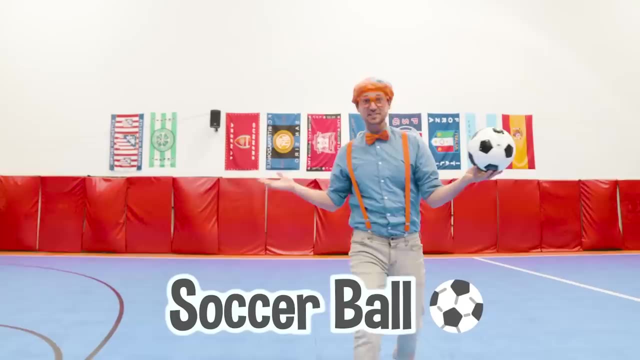 Hey, it's me Blippi, and today I'm at LA Bubble Soccer in Northridge California And check it out. This is a soccer ball. Some countries call it a football. Whoa, it's so fun to play with. 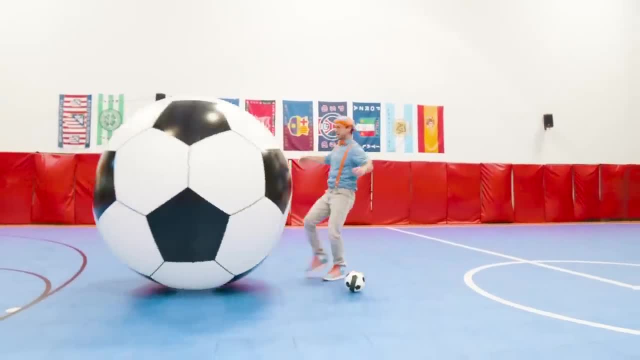 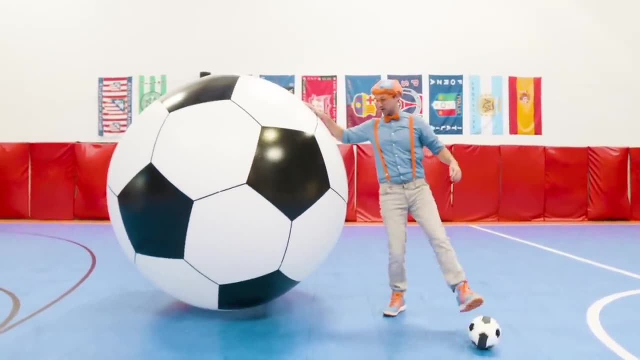 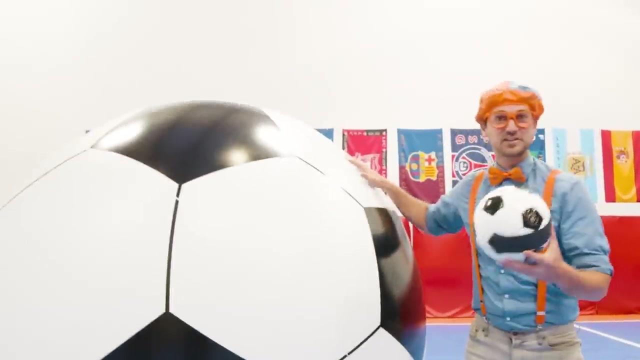 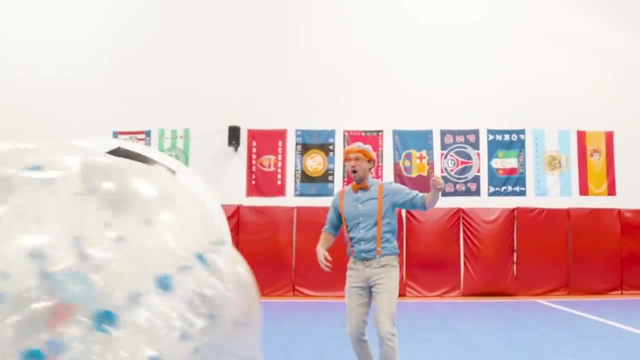 Whoa, whoa, Check this out. This is another soccer ball. Whoa, and this football soccer ball is really big and This one is small. I Love playing with soccer balls. Whoa, What's this? whoa, it looks like a bubble. yeah. 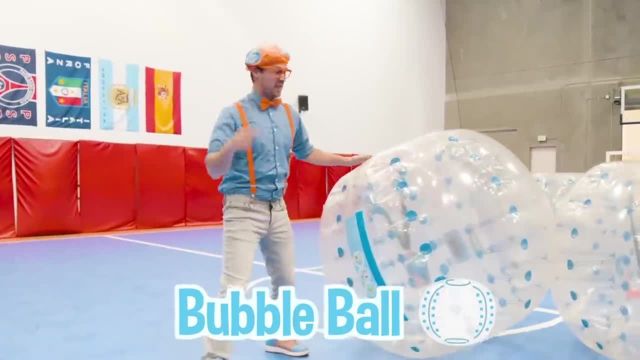 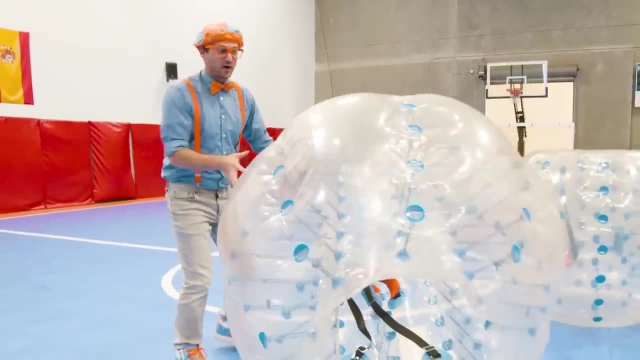 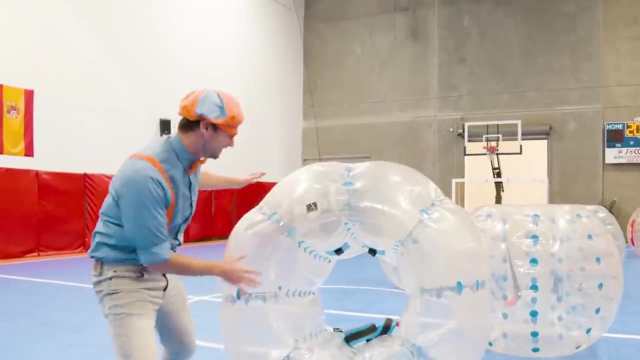 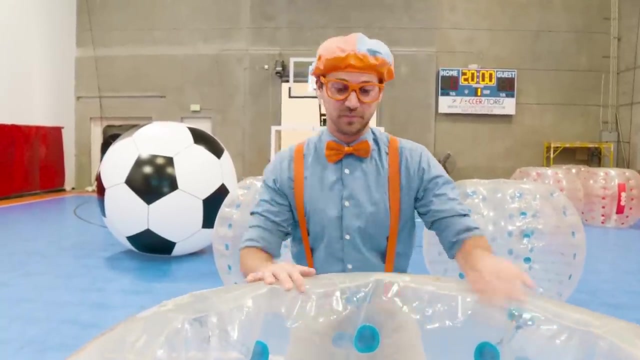 bubble, Bubble ball. this sport is called bubble ball. It's basically like soccer football, But you get inside these bubbles with your body and then you play soccer and football. Check it out. The first thing that you have to do before you play bubble ball is get inside the bubble ball. 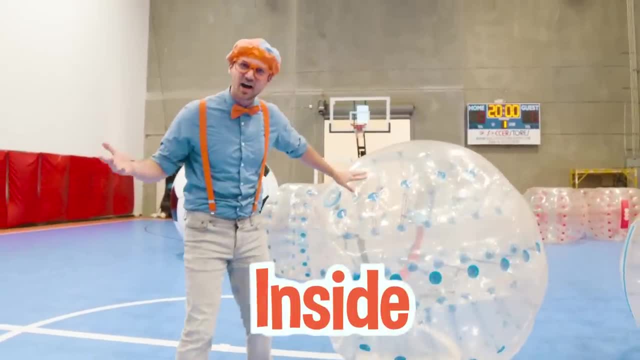 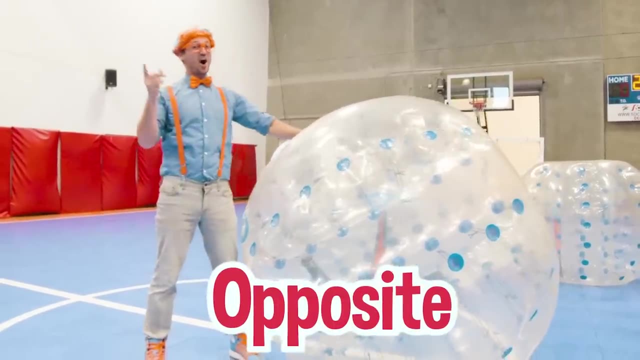 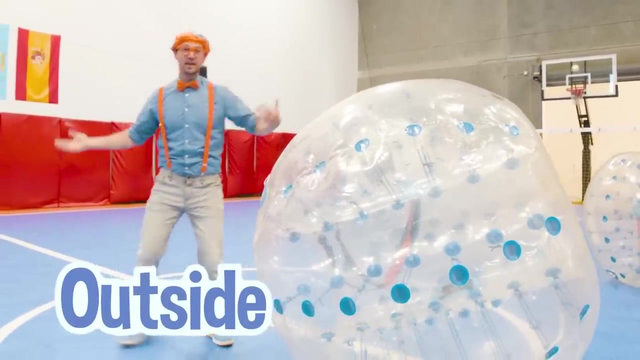 Okay, Hey, did you hear how I said inside? Yeah, that means I am outside the bubble ball. Do you know what an opposite is? an opposite is the exact reverse of something totally different. so if I'm outside and then I need to go inside, 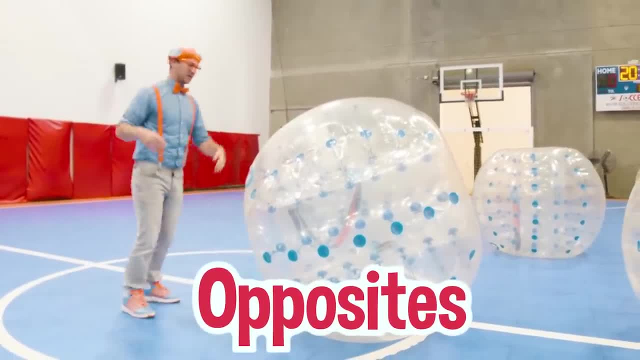 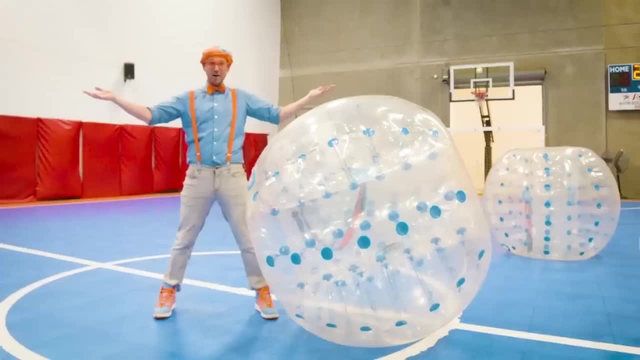 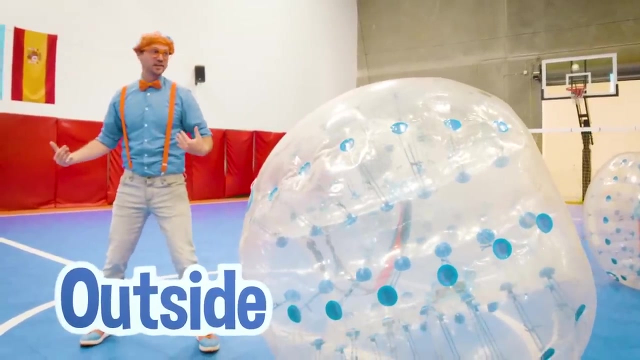 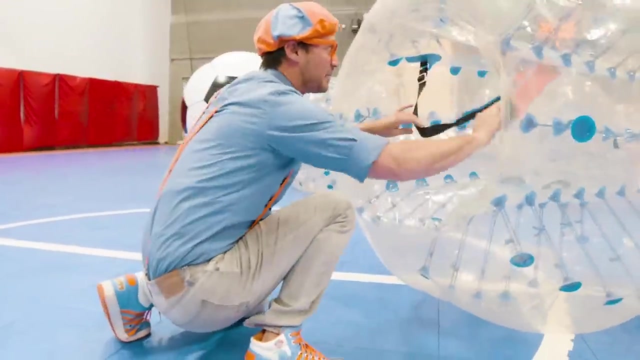 Inside and outside are opposites. So now that I'm outside, Let me get inside. What is the opposite? What is the opposite? What is the opposite of inside the ball, Outside the ball, Outside the ball, Outsides- the opposite of inside the ball. Okay, this is pretty tricky, but see these straps. you put it on like a backpack. 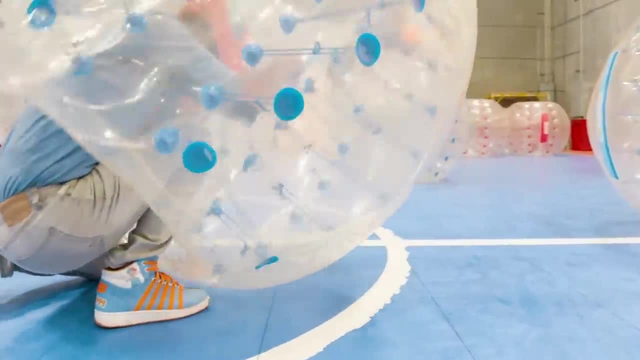 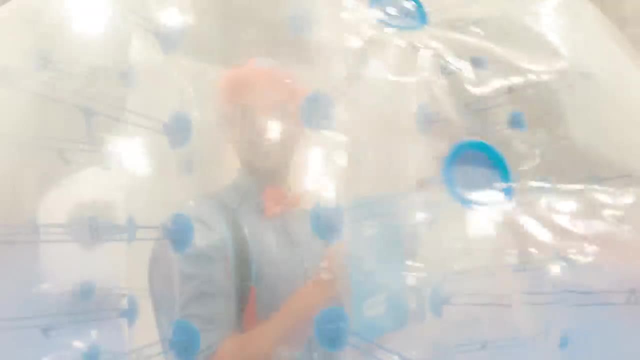 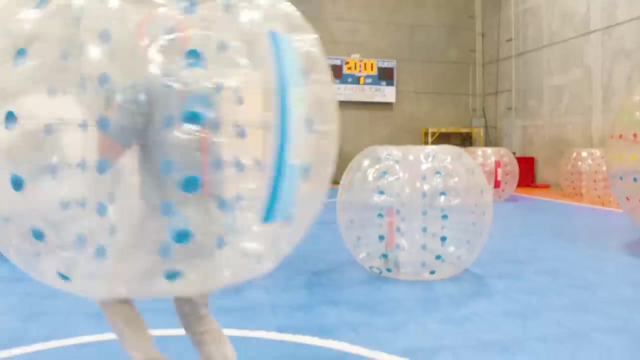 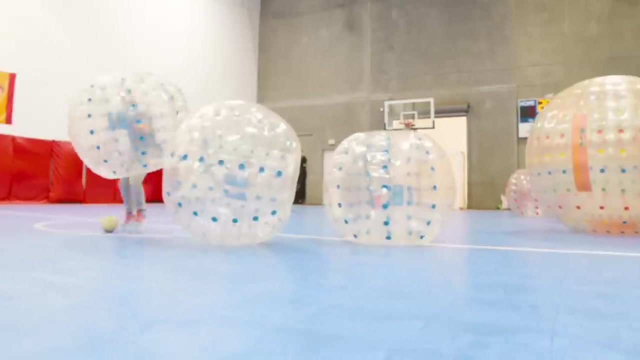 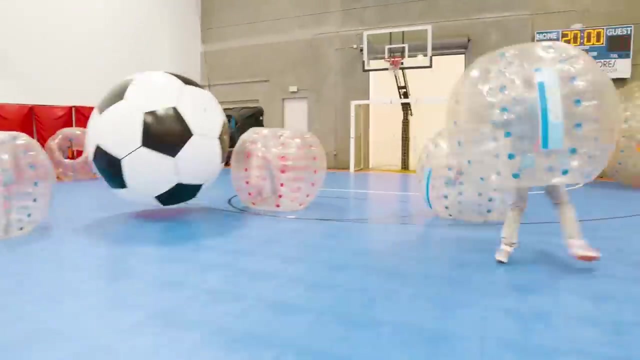 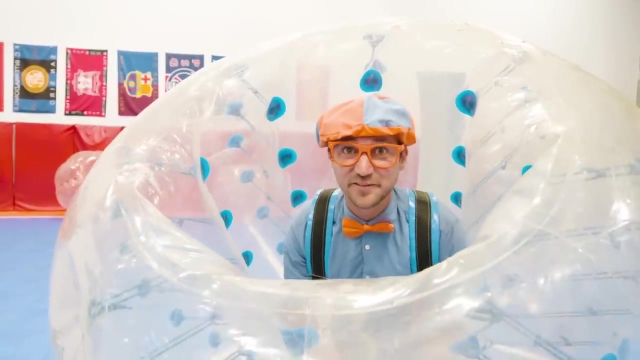 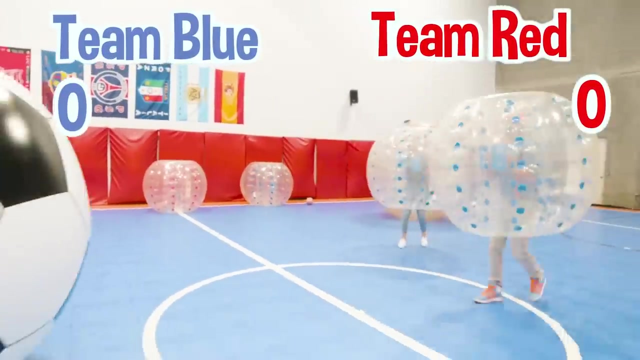 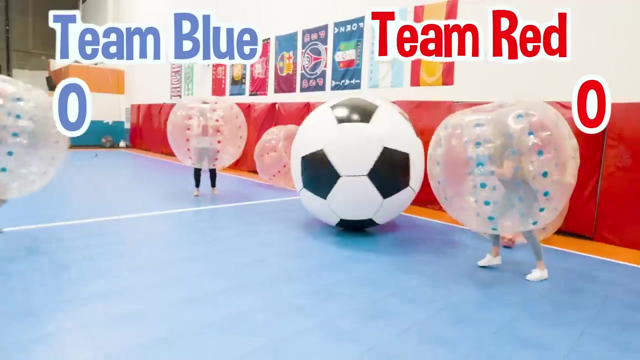 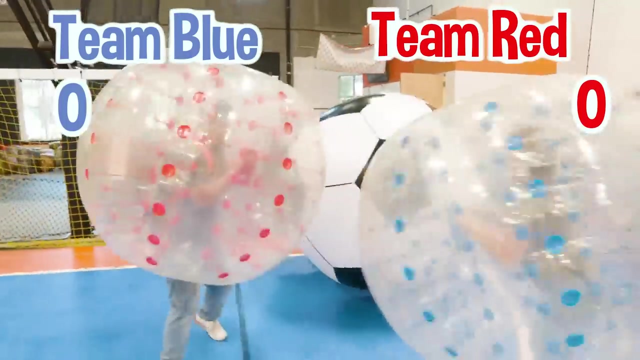 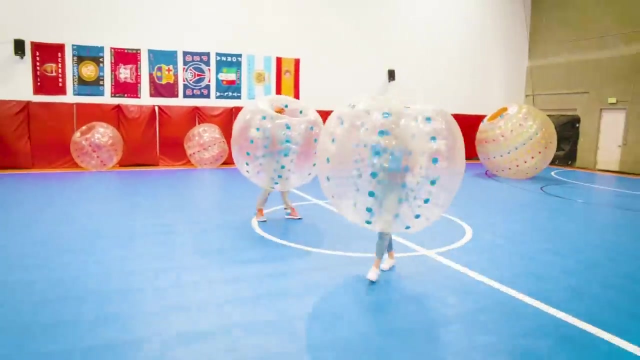 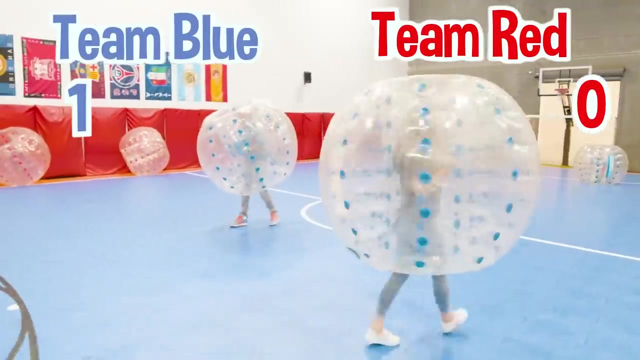 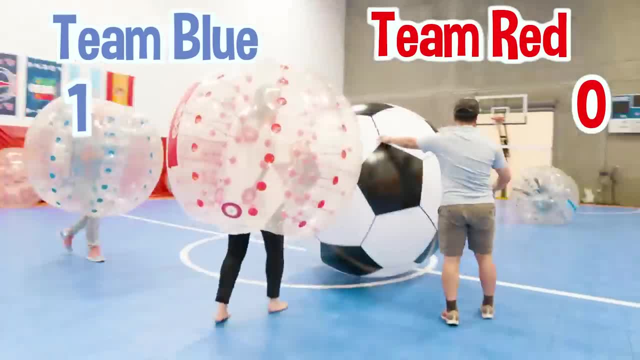 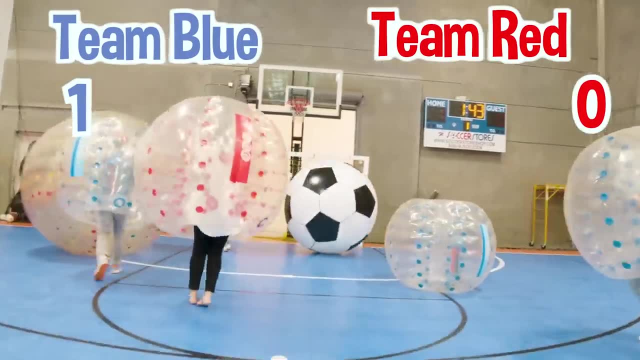 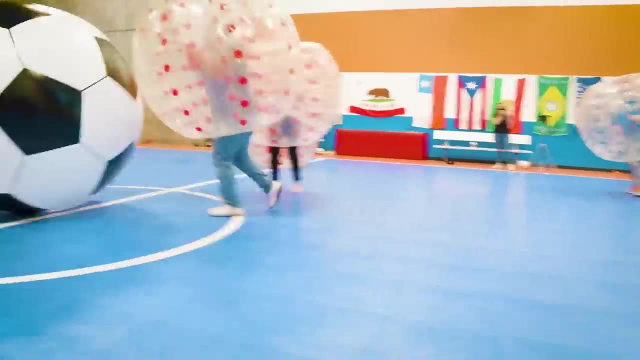 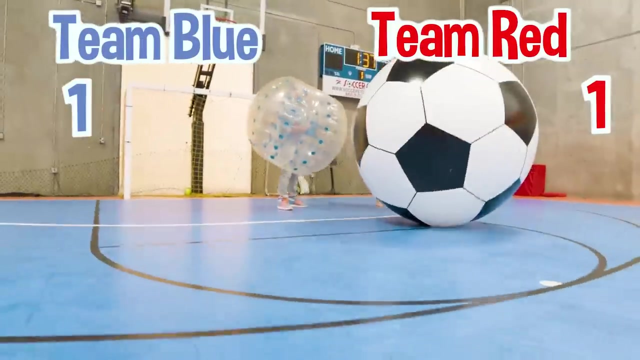 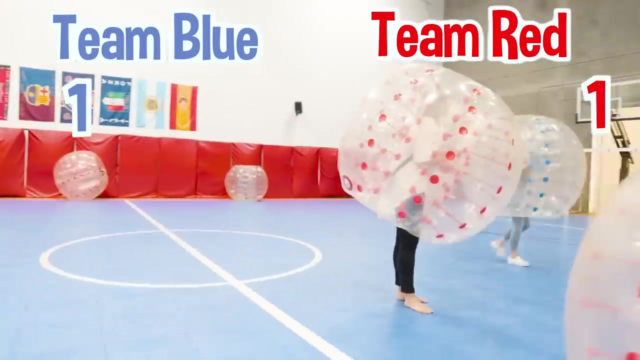 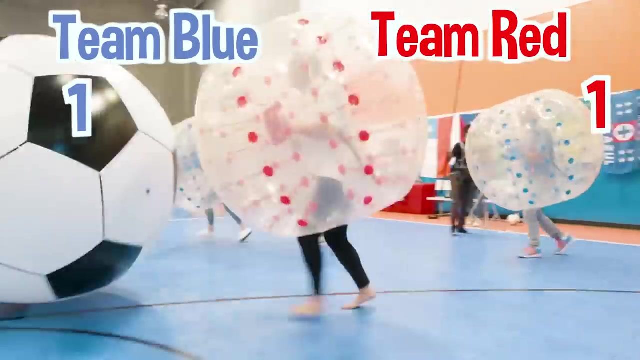 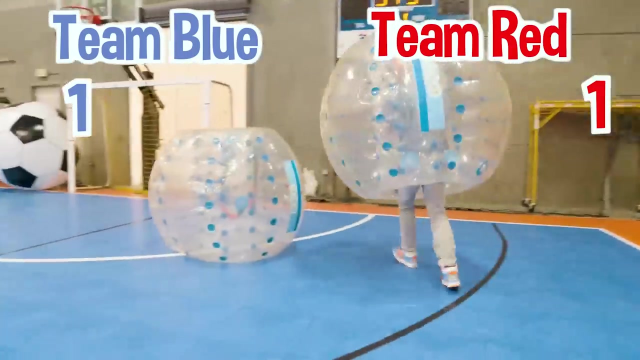 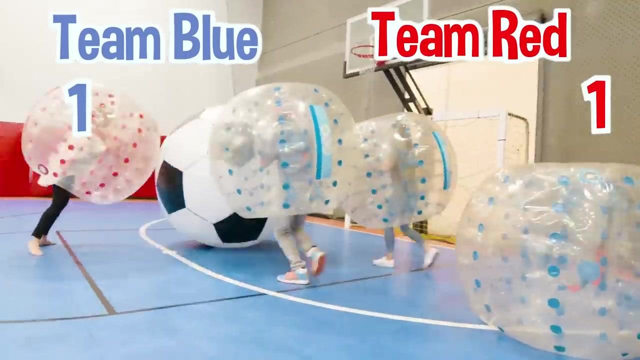 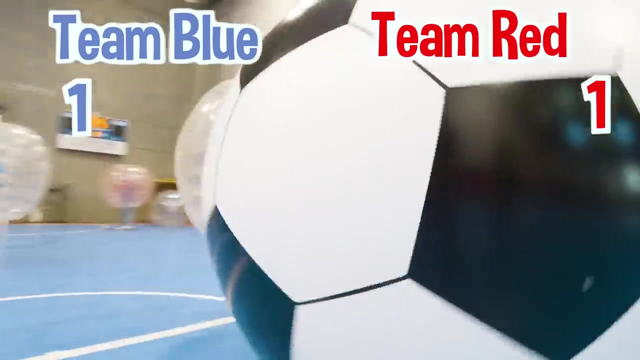 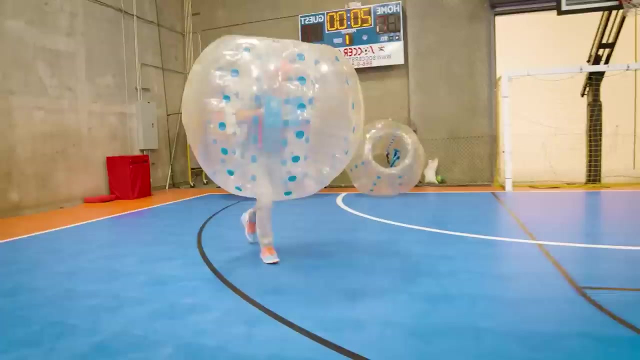 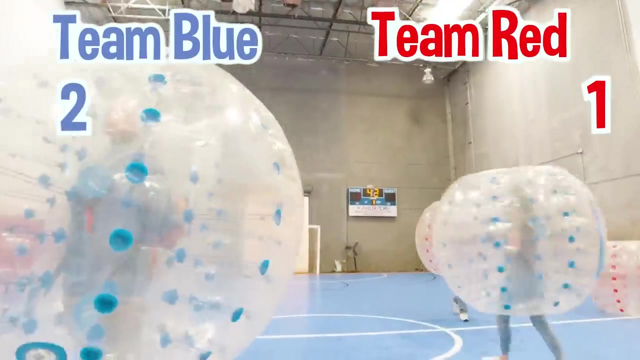 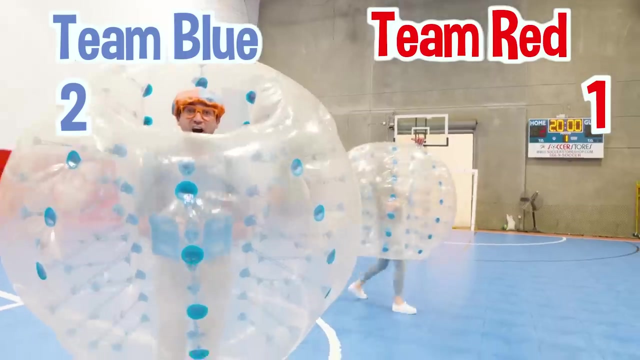 Oh, Oh, Oh, Oh Oh. Goal for the Reds. goal for the Reds. We're having so much fun. goal for the Reds. Goal for Blippi. goal for Blippi. He's got so much energy. goal for Blippi. I am so tired And Team Blue won. 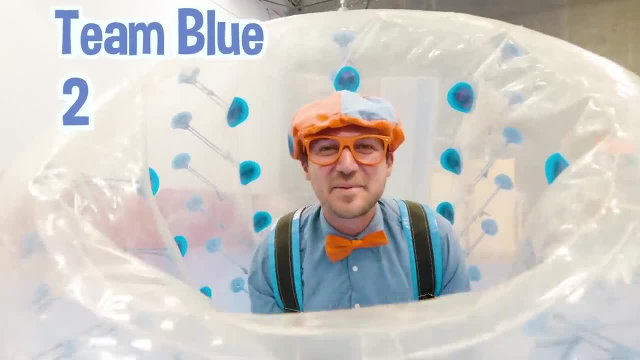 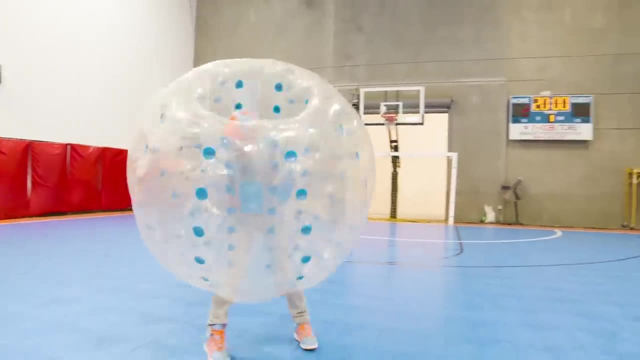 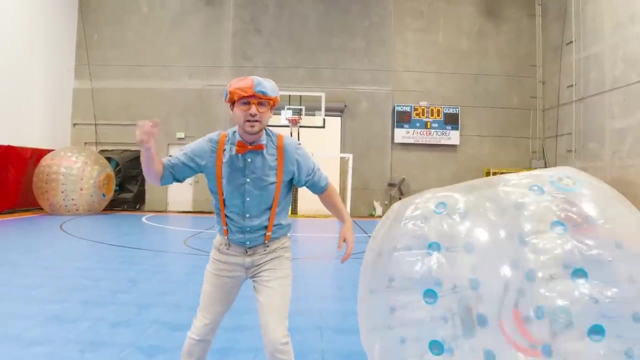 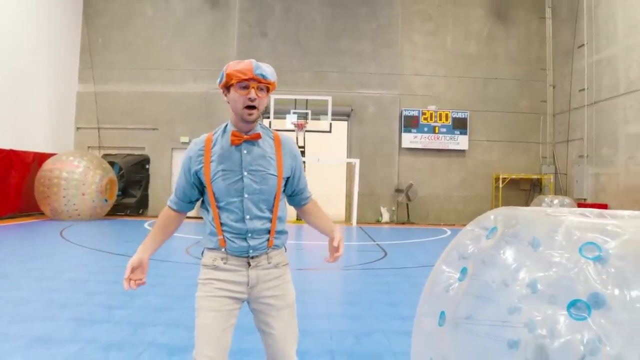 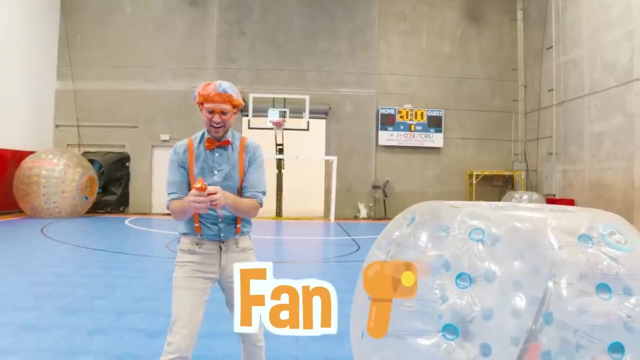 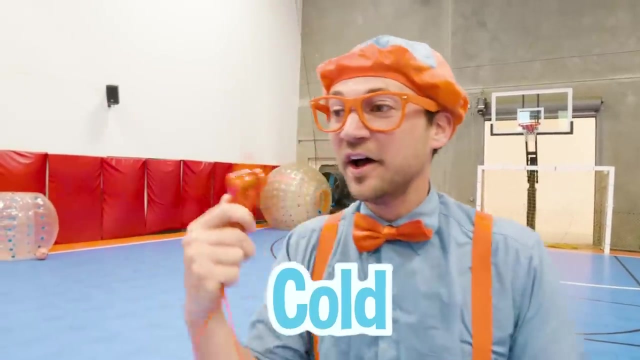 Everyone did a really good job at Bubble Ball today. I am so hot and sweaty right now. Do you see this? Hey, I have an idea: The opposite of hot is cold. I have a fan right here, See. Maybe if I put the fan I will become cold. 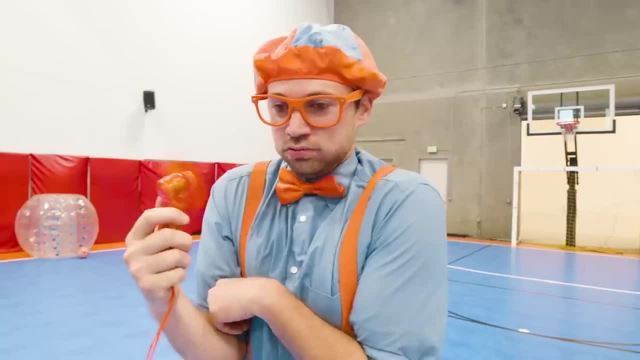 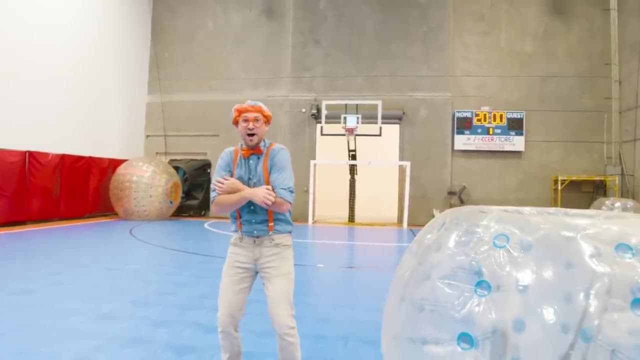 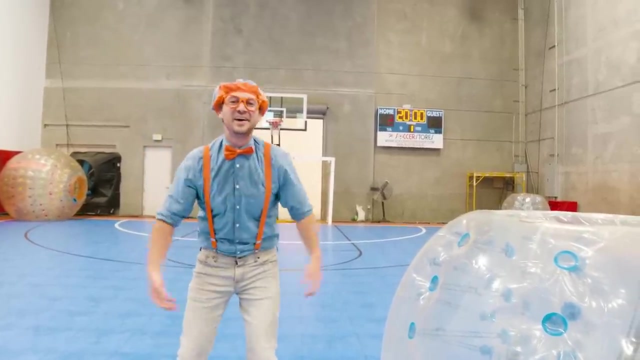 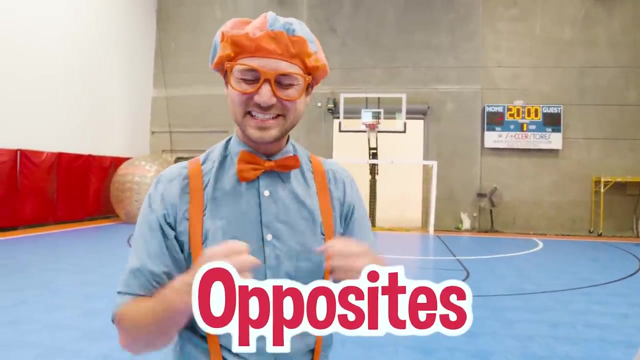 Yeah, it's working. Oh, brr. Oh, I'm so cold now. I used to be hot And then now I'm cold. Well, this was so much fun learning about Bubble Ball with you And opposites. Yeah, I love learning with you. But this is the end of this video. 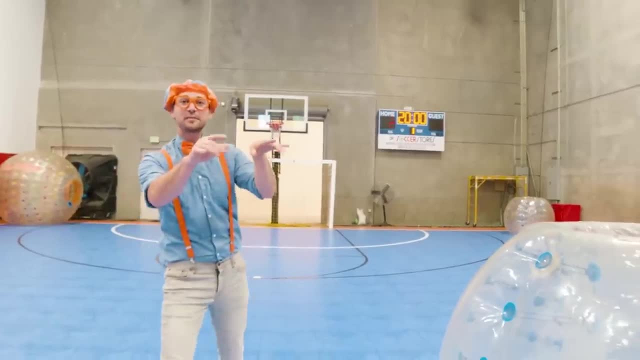 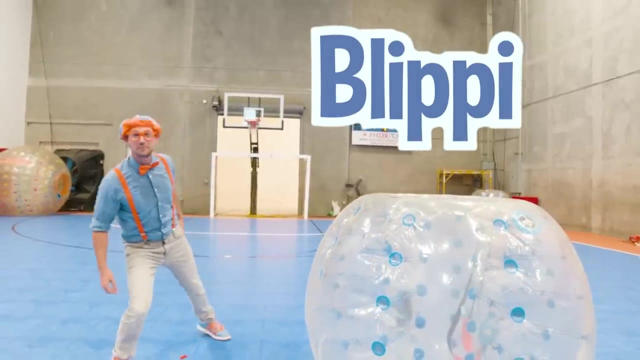 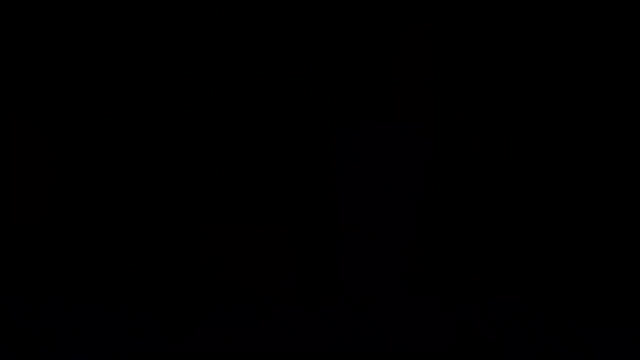 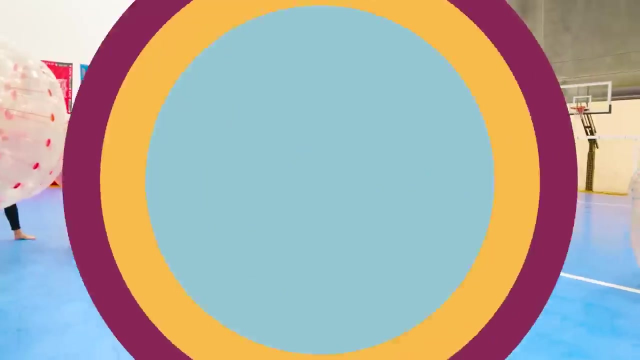 But if you want to see more of my videos, All you have to do is search for my name. Will you spell my name with me? B-L-I-P-P-I, Blippi. Good job, All right, see you later. Teamwork is dreamwork. We play together. 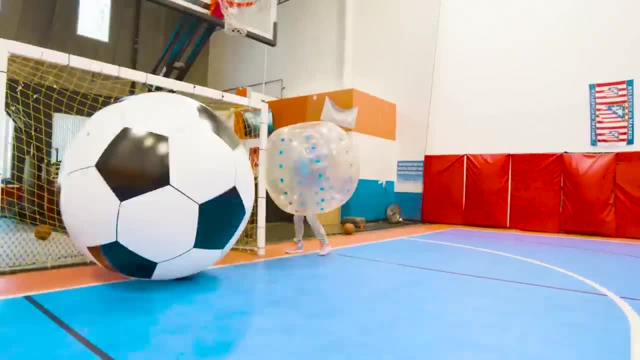 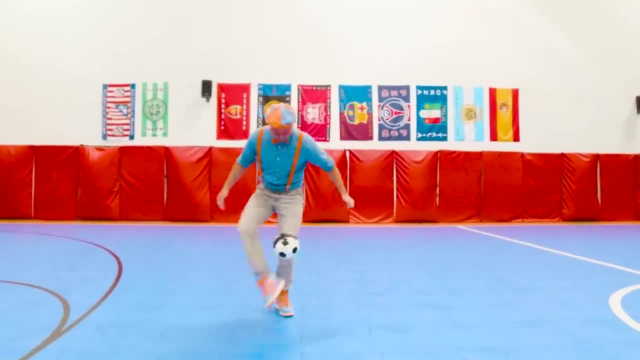 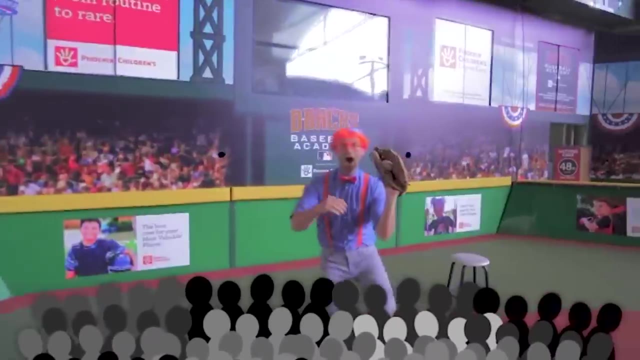 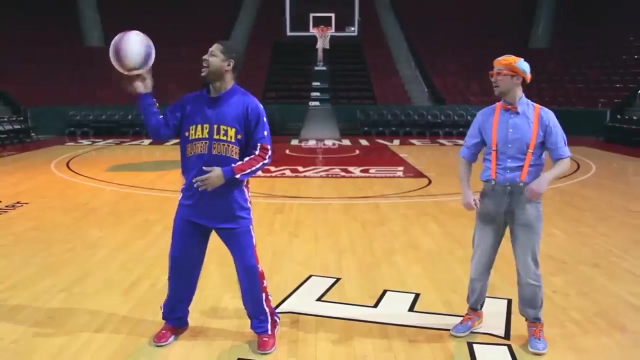 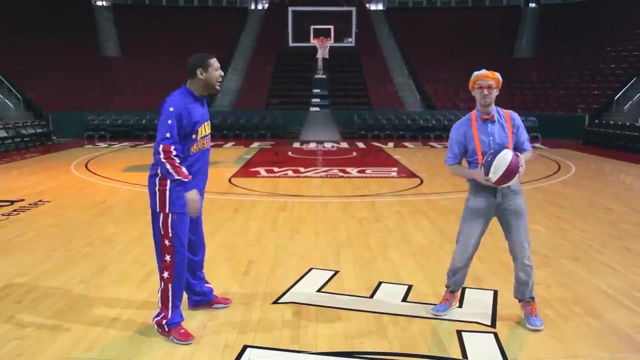 Run, pass and score. Make friends forever. Teamwork is dreamwork. We play together, Run, pass and score. Make friends forever. All for one And one for all. Together We can win it all. Dribble the ball and pass some more Kick and score. 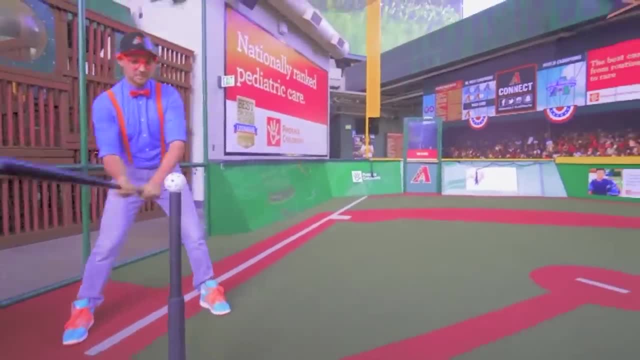 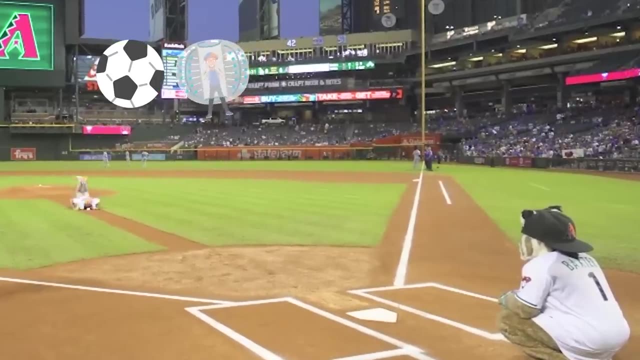 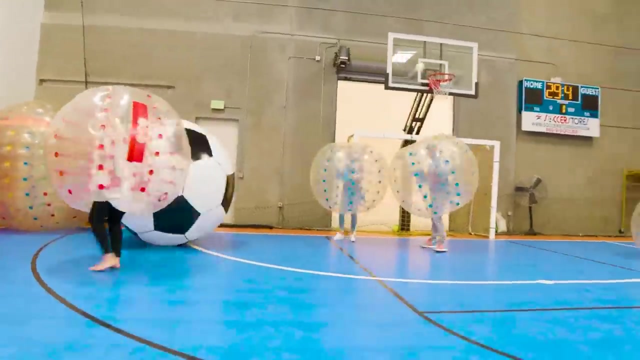 That's what we got in store Up to bat. It's all we got. It's time to swing. It's a home run. We all win. Are you a team player? Let me hear you cheer. Are you a team player? Let your friends take the wheel. 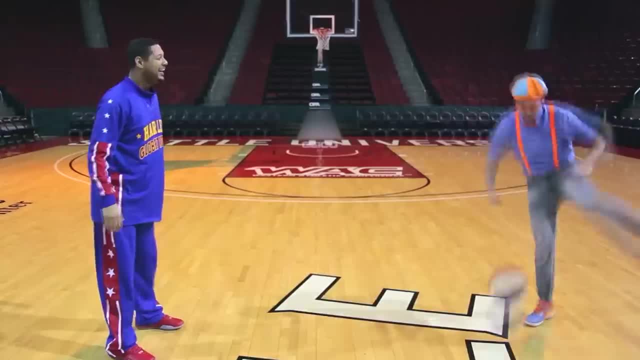 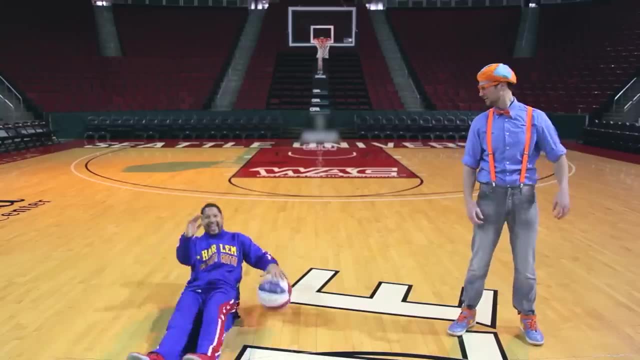 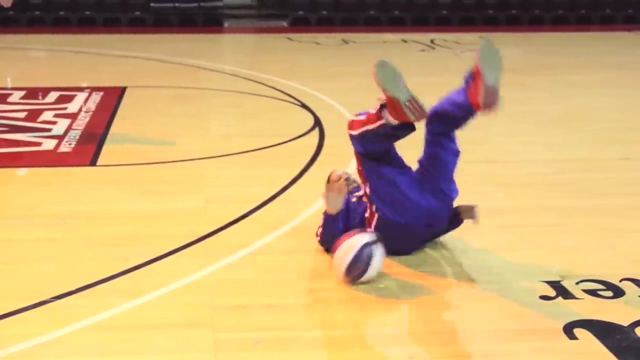 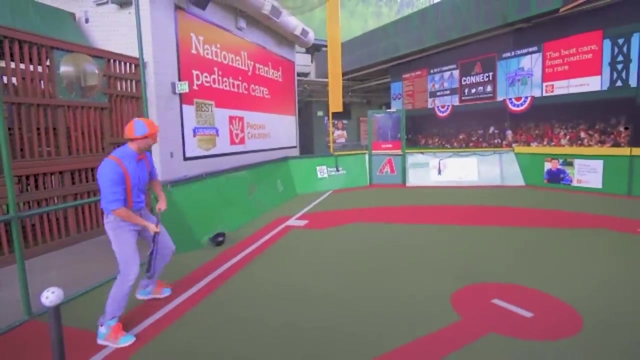 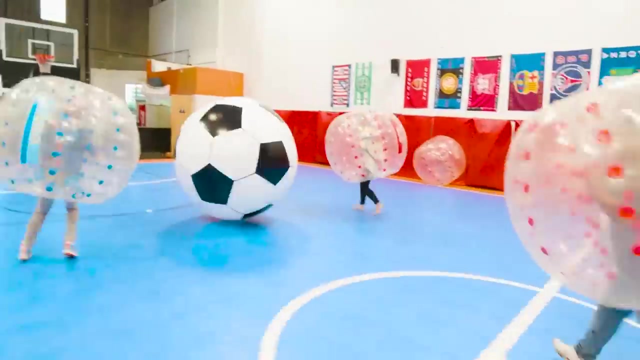 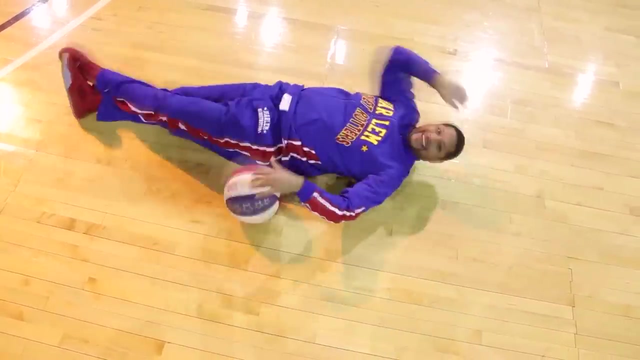 Teamwork is dreamwork. We play together, Run, pass and score. Make friends forever. Teamwork is dreamwork. We play together, Run, pass and score. Make friends forever. All for one And one for all. Together, We can win it all. Sports take skills. You learn something new. 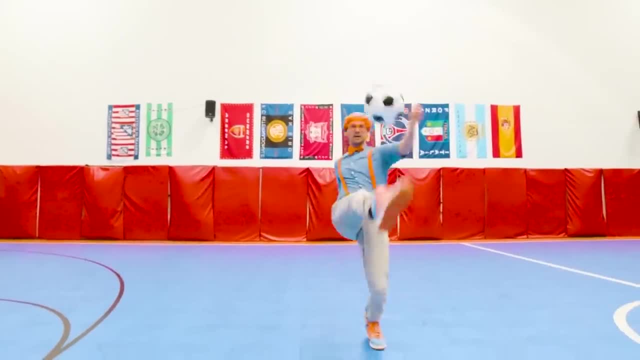 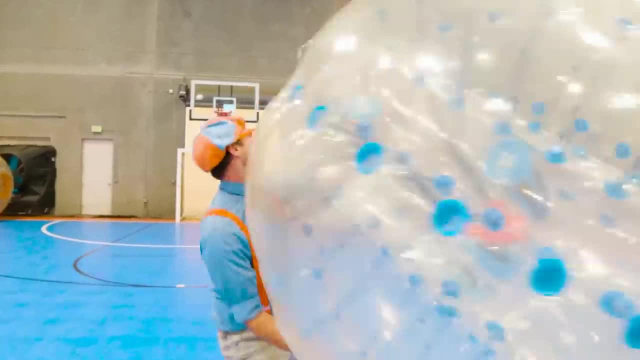 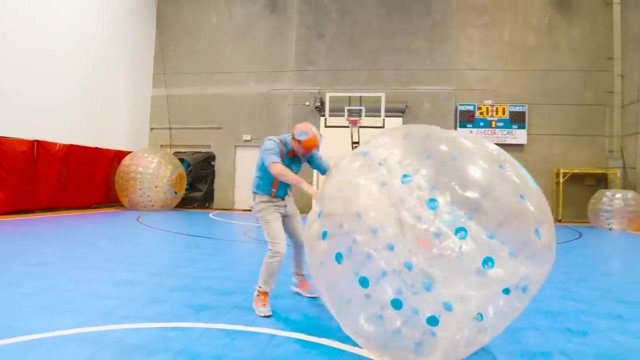 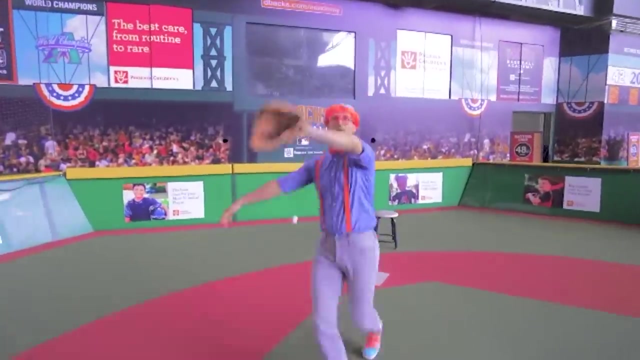 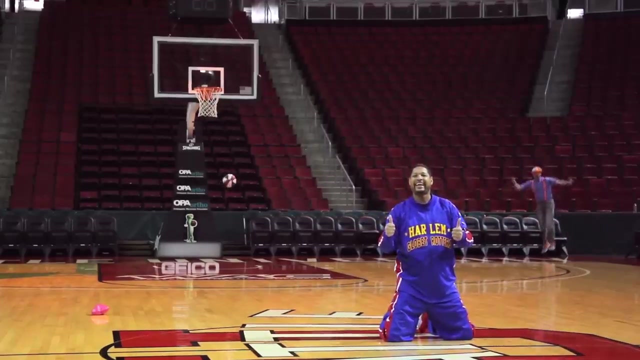 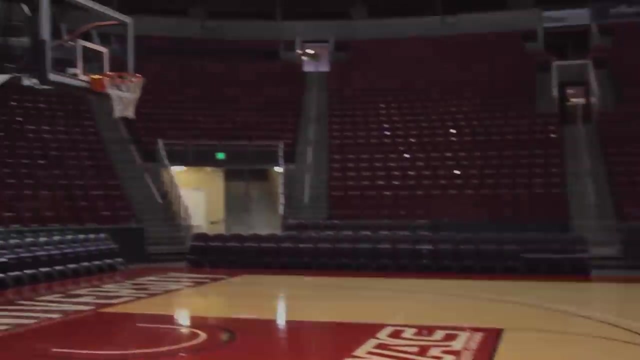 Practice And practice Is what you gotta do. Teamwork is dreamwork. We play together, Run, pass and score. Make friends forever. Teamwork is dreamwork. We play together, Dribble pass, score, Make friends forever. All for one And one for all. Together, we can win it all. 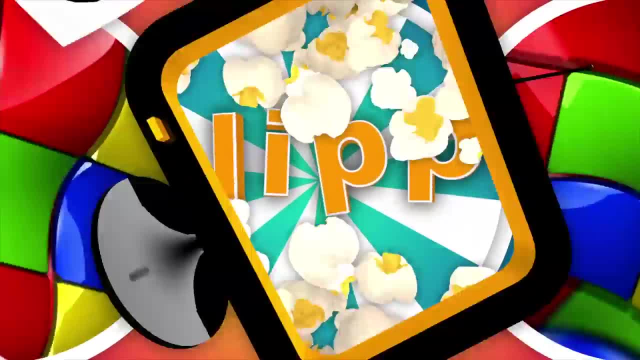 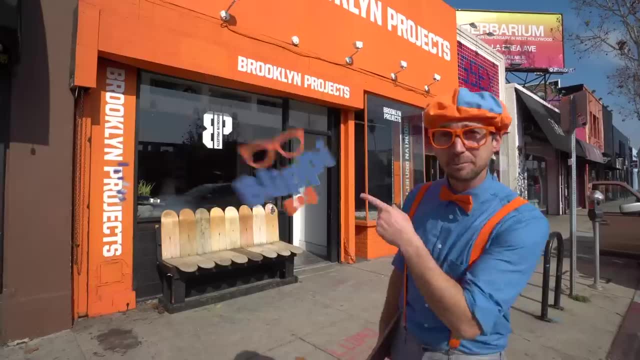 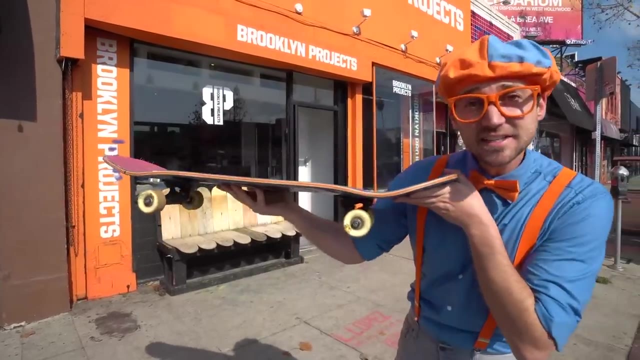 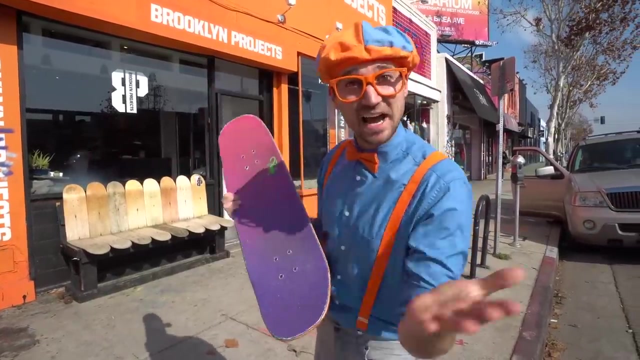 So much to learn about. It'll make you wanna shout: Blippi. Hey, it's me, Blippi, And look at what I have in my hand. Whoa, Do you know what this is? This is a skateboard, And I think you and I Should learn about skateboarding. 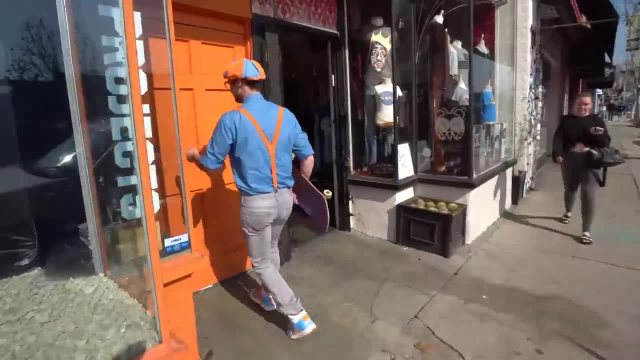 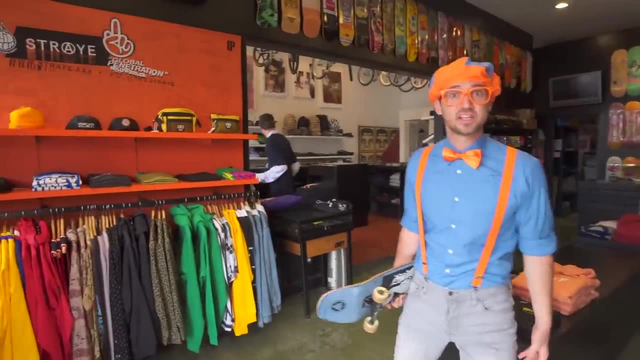 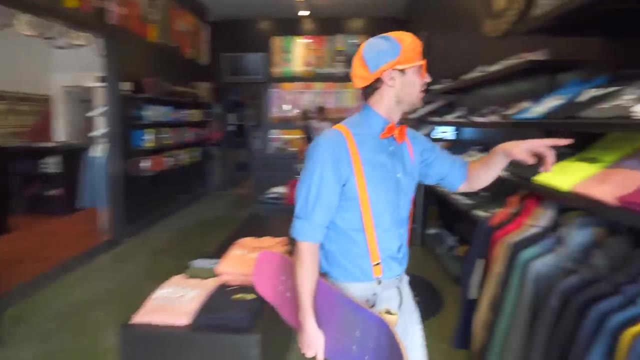 Come on, Blippi, Dribble, Dribble, pass and score. Whoa, Look at this store. This is the Brooklyn Projects In Los Angeles, California. Whoa, this place is so cool. Whoa, check this out over here. Whoa, Cool apparel. 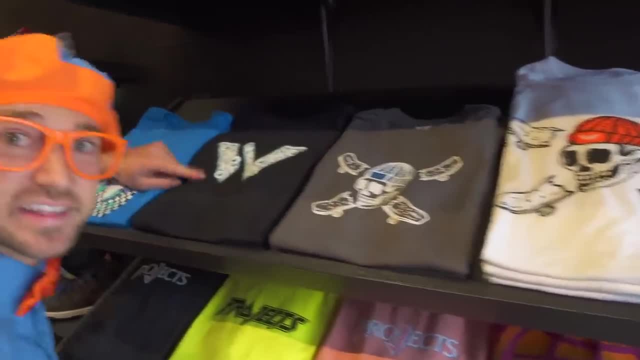 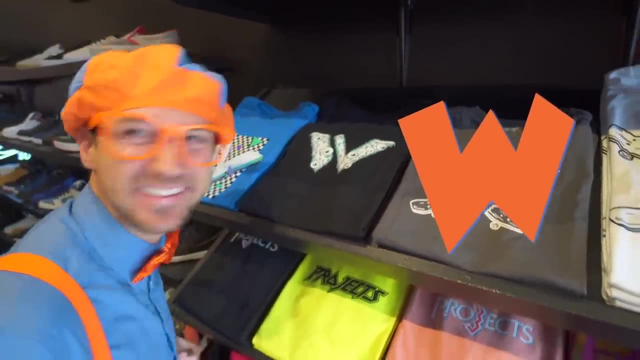 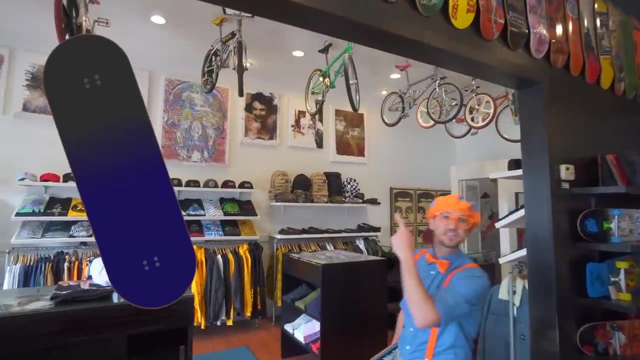 Whoa, look at these designs up here. Ooh, look at this. It's all fuzzy like a monster. Blippi, Dribble, pass and score and it's the letter W- pretty cool. whoa, come check it out. haha. skateboard decks up there, even BMX bikes. oh, this store owner must really 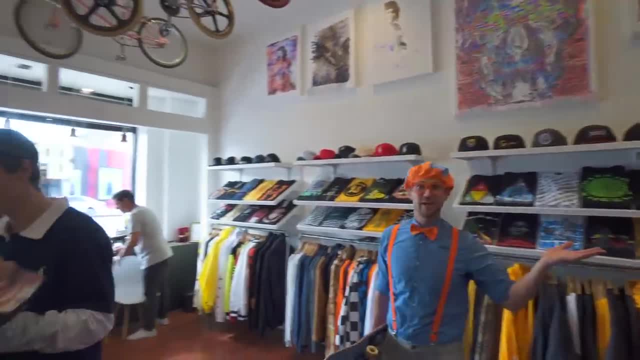 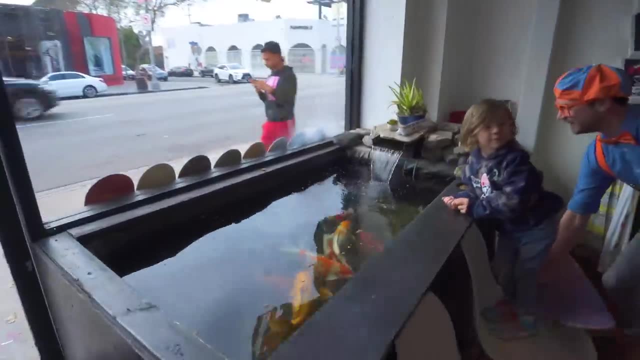 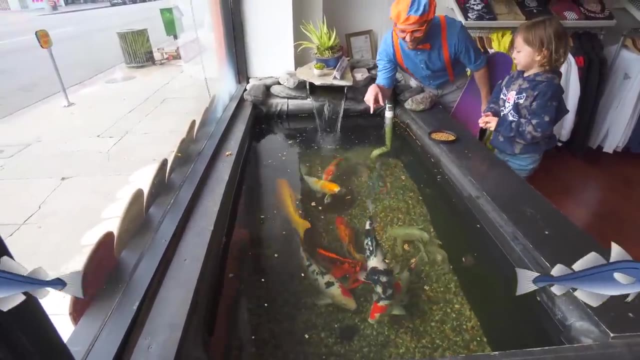 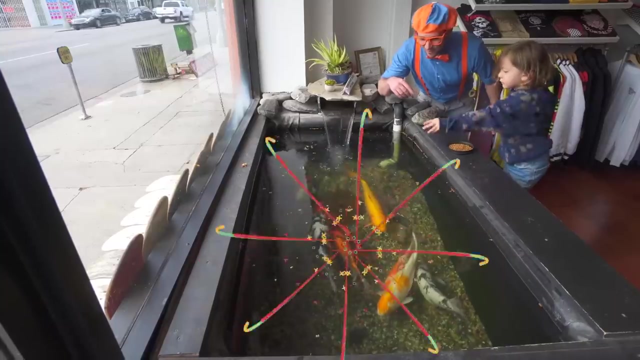 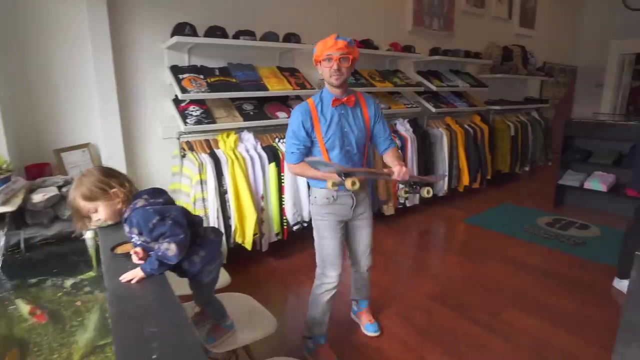 love skateboarding and BMX bikes. whoa, what's over here feeding the fish? the shop has a bunch of fish here you go. all right, throw it in there. all right. bye-bye fish. all right, see you soon. all right, hey, I think it's time to see if one of the workers will help me learn how to skateboard. come on. 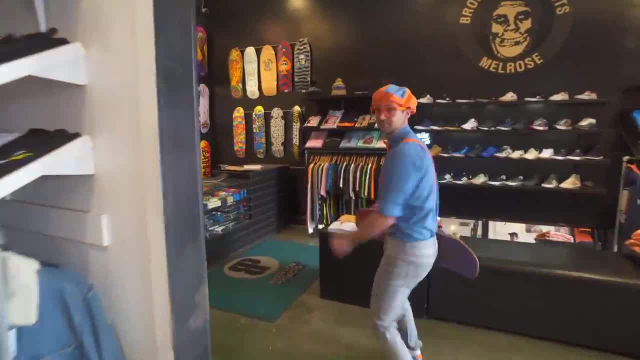 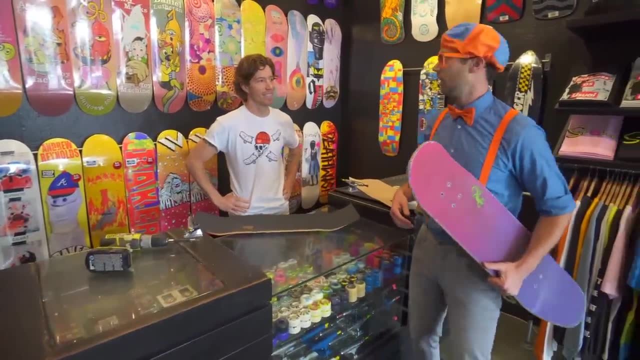 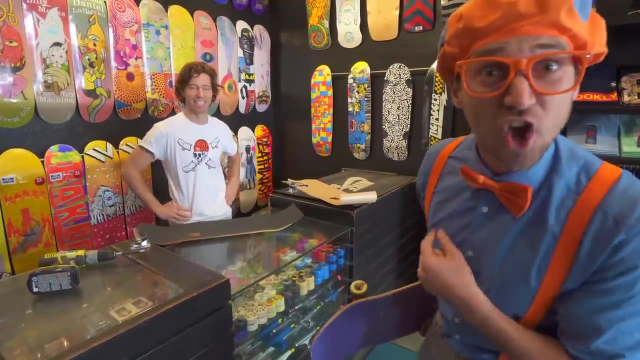 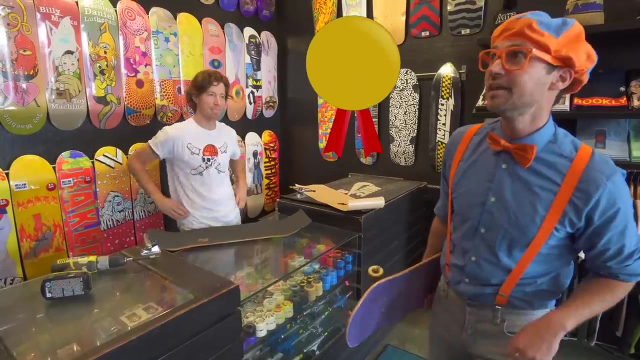 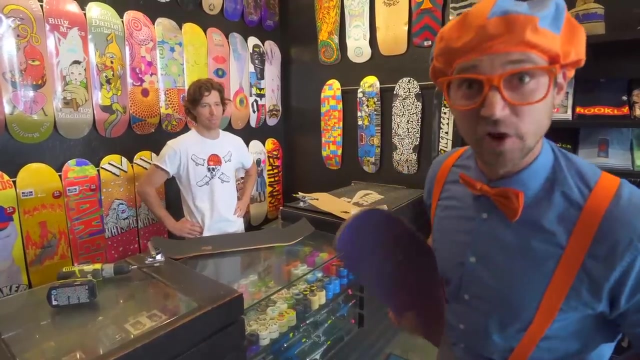 whoa, pretty cool. hey, good sir, carry me sit. do you know who that is? that's Shawn White. he's won three gold medals in the Olympics for snowboarding: one, two, three whoa- and he's a professional skateboarder. let's ask him for help. I'm gonna help you, I just uh. 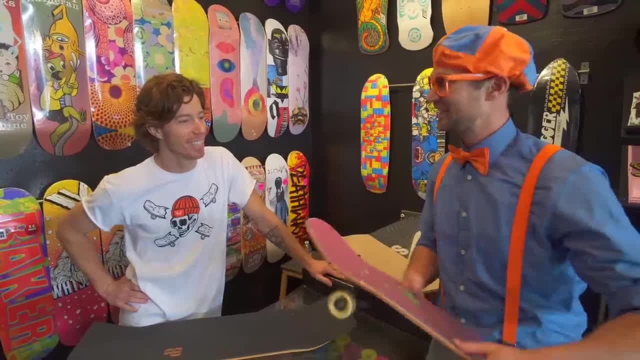 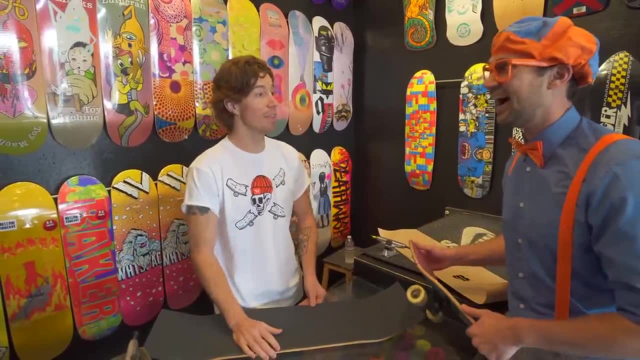 ahem, Just curious if you could help me learn the skateboard today. Oh yeah, you want to learn how to skateboard. you know, I've been skateboarding my whole life, love doing big airs and things. I'm just setting this board up and we'll take you out back, show you how to do it. 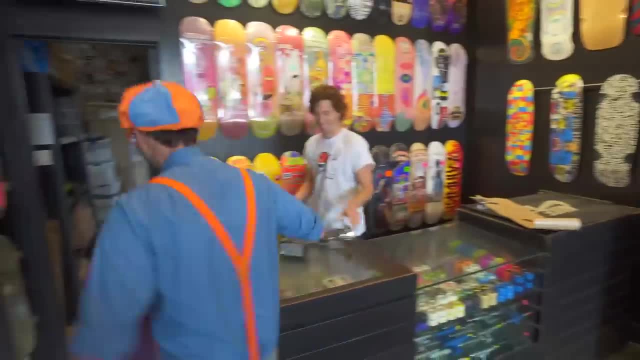 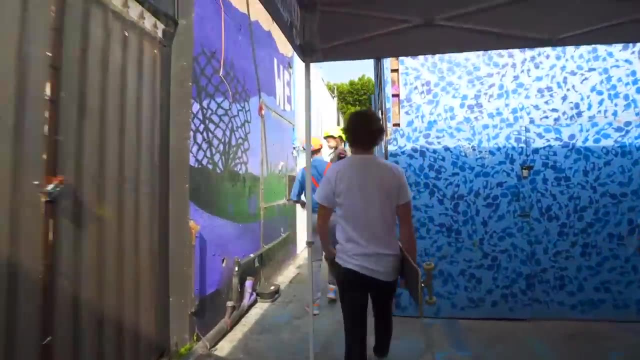 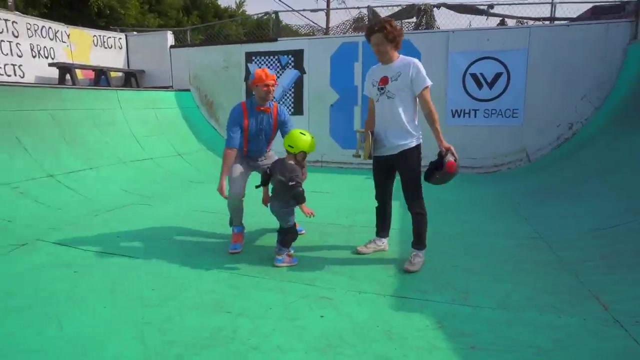 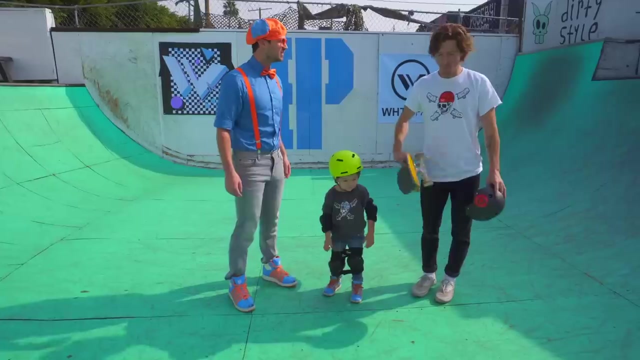 Okay, let's go. Yeah, awesome, Whoa, check it out. Whoa, this is a big ramp. is this where you skateboard at? This is Pretty cool, Alright. well, will you show us? Well, hold on, you know you're going to need some protective gear first. 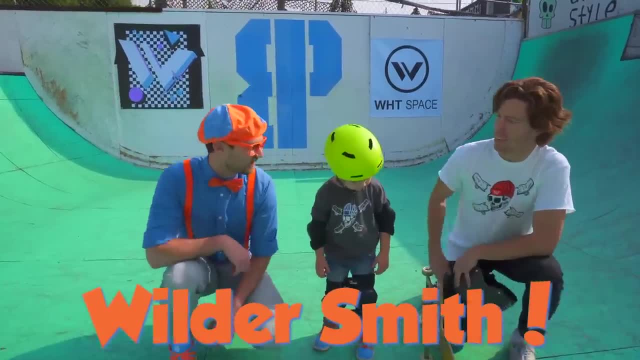 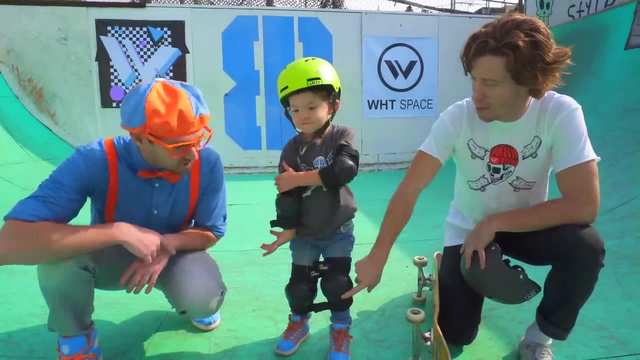 Alright, what's that? Check out my buddy Wilder here- Whoa, He's got a helmet, Wow, Yep. then he's got his elbow pads Right here, Yep. and then you've got your knee pads down here. 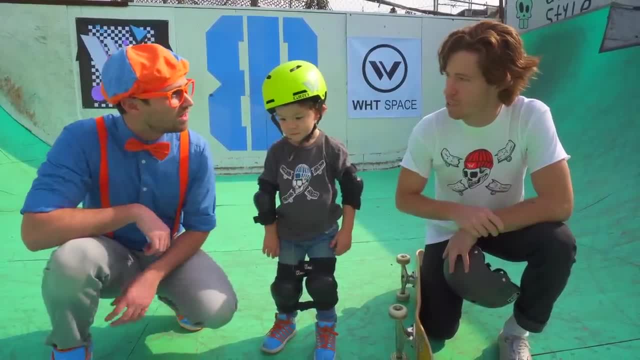 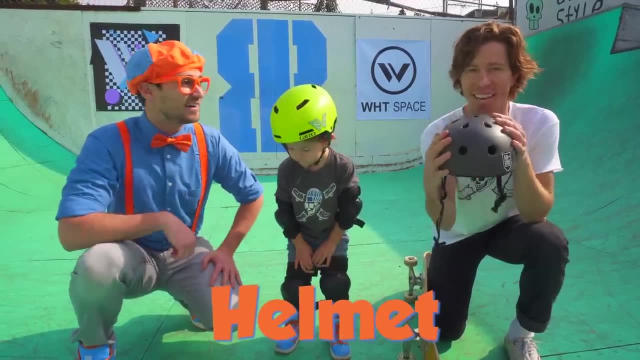 Ooh, and this is to help protect you for if you fall, Yep, just in case of a fall. Whoa, that's pretty cool. And what are you going to wear to be safe? I brought my lucky helmet. Okay, well, put it on and let's see a ride. 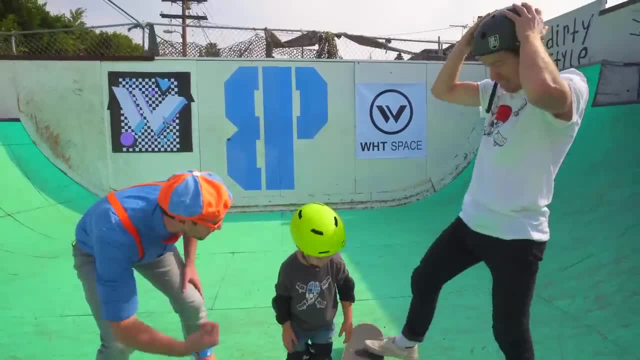 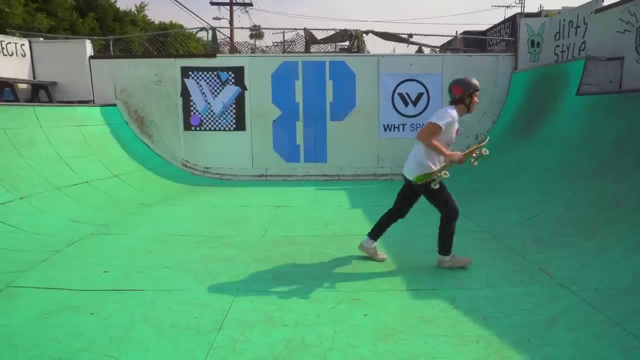 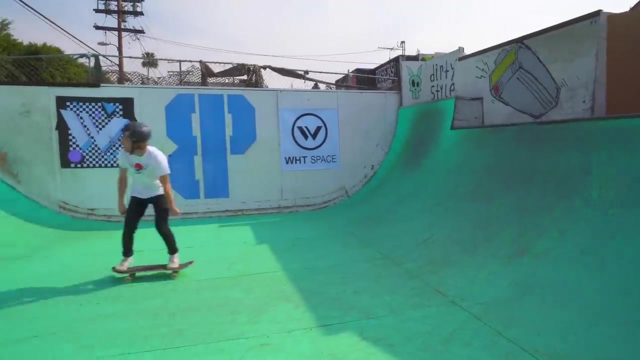 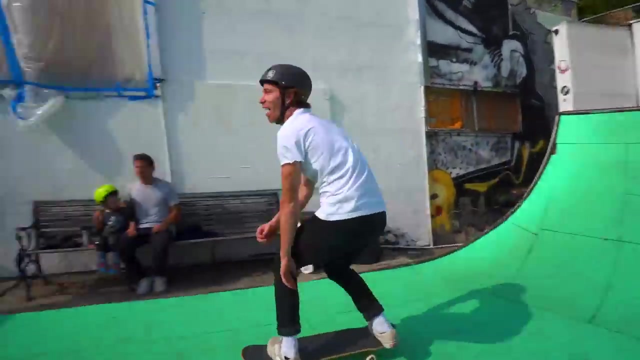 Alright, here we go, guys, Alright, here. you want to come this way, Let's go, Here we go, And this is where I'm going. Wow, Whoa, Whoa, Thank you, Thank you, Thank you. 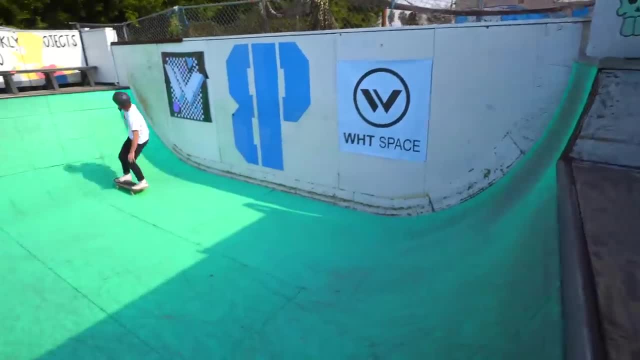 Welcome to Vancouver, everyone. This is the start of your new adventure. Well, actually I'm not going to do that. I'm going to walk you through the whole thing. You're not going to walk me through, so On your way. 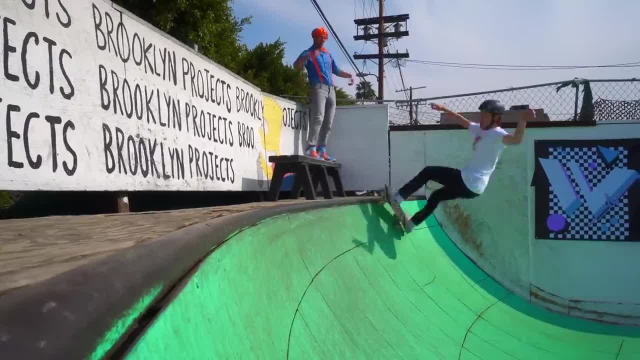 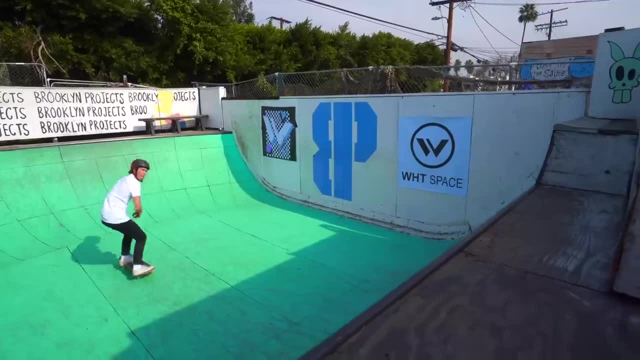 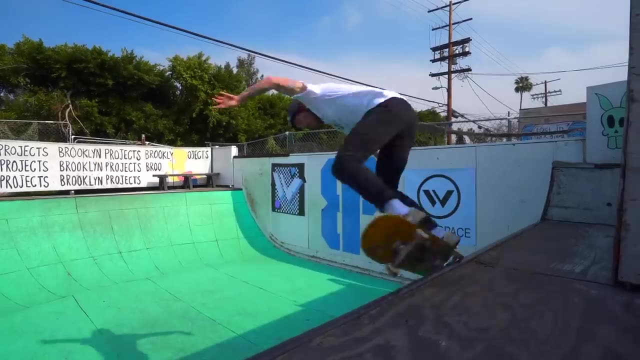 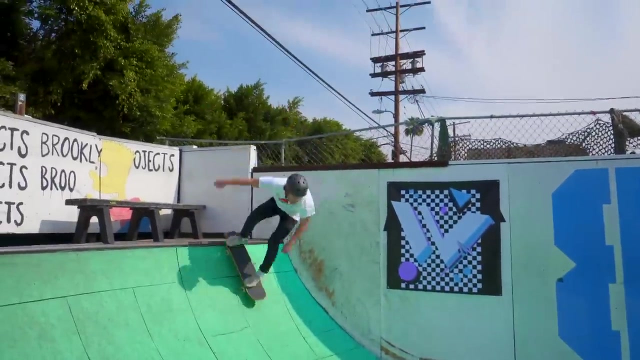 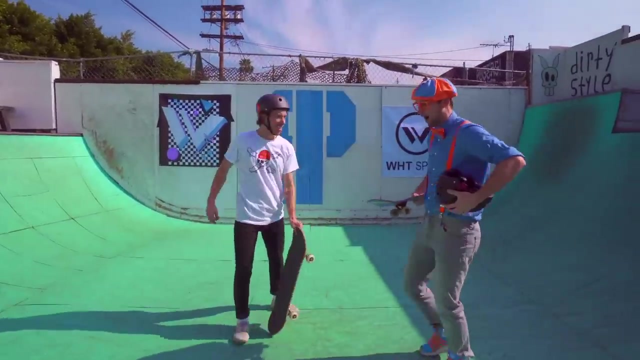 On your way. I've always wanted to do that, So what are you going to do? Alright, what do you think That was so cool? Well, you know, I've been working really hard at this for a long time. 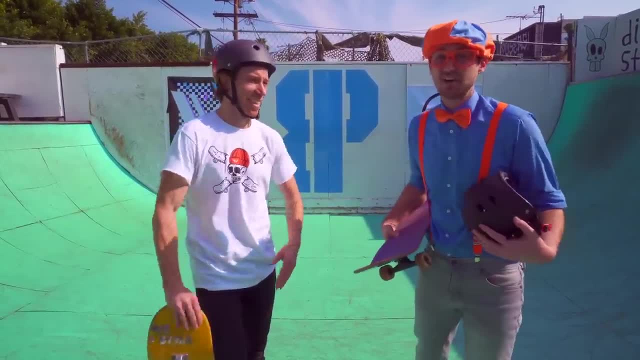 So if you practice, you'll make perfect. Oh well, that's good to know. Can I try now? Of course, Okay. Okay, first thing, put the board down. Okay, I'm going to put your helmet on, Alright. 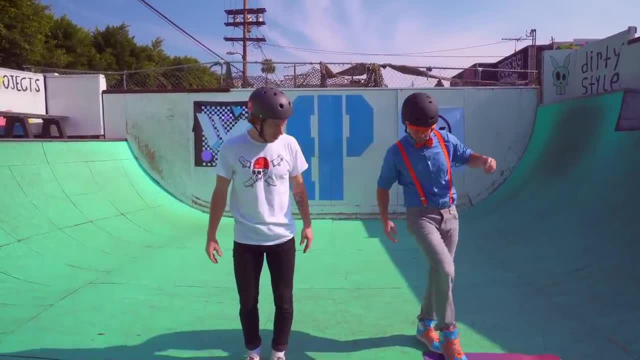 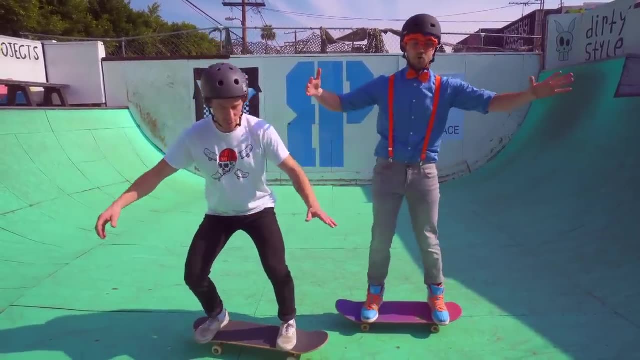 There you go. Okay, Now put whatever front foot feels good. Okay, Right toward the front of the board, Alright. And then you pull the back foot on. Oh, And then you keep your knees bent. Oh, That's the key. 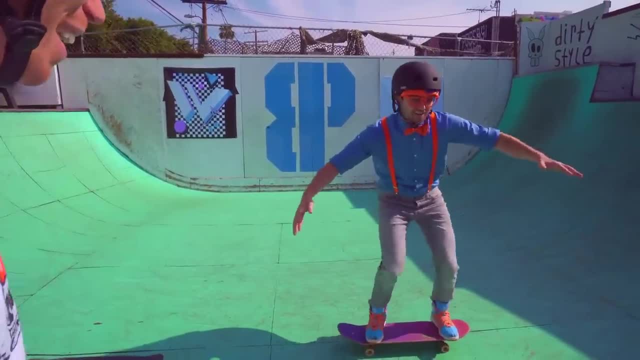 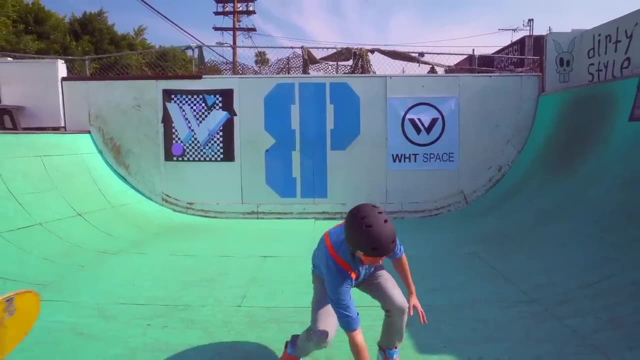 Whoa, There you go. Whoa, Whoa, Whee, Whoa. This is harder than it looks. Whoa, Oh, Oh. All right, That was pretty good, Yeah, But I think I know what you're missing. 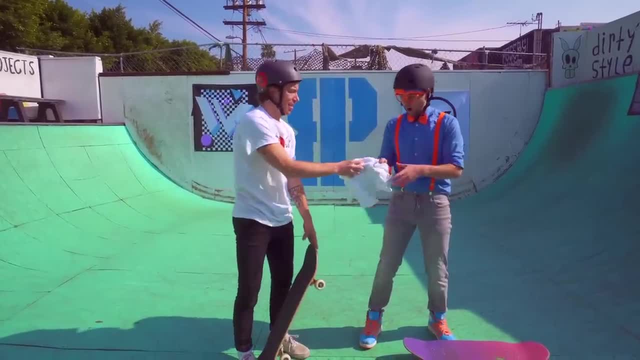 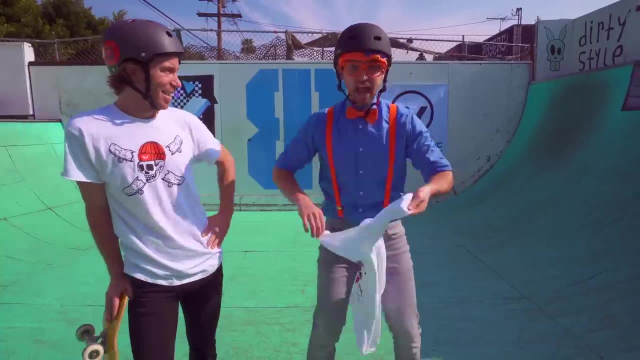 What is it? Yeah, Here we go. Whoa, Got that for you. An official Sean White white space t-shirt. Yeah, That's totally what I'm missing. Okay, Let's put this on. Right on, Here we go. 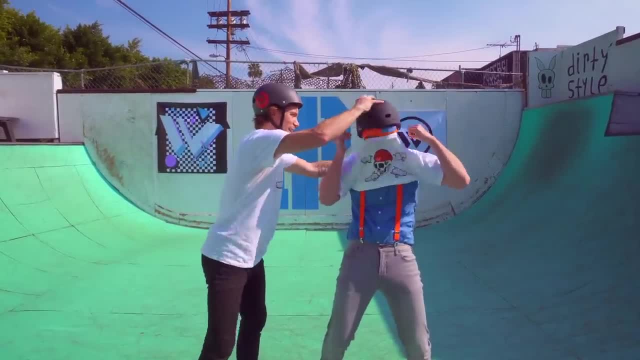 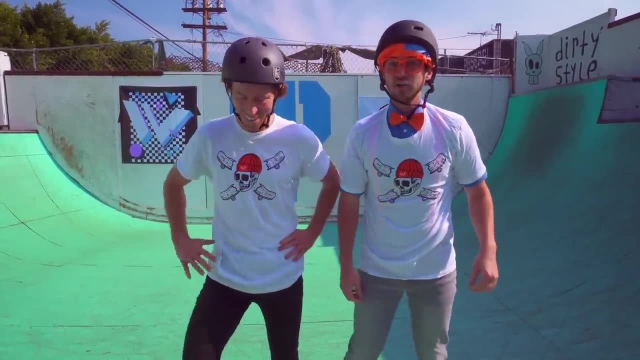 Here we go, I'll help you there. Oh, That's silly. Okay, All right, Looking pretty good. How do we look? Looking pretty good? Yeah, Oh, And you know what else? Yeah, The souls of the animal kingdom. 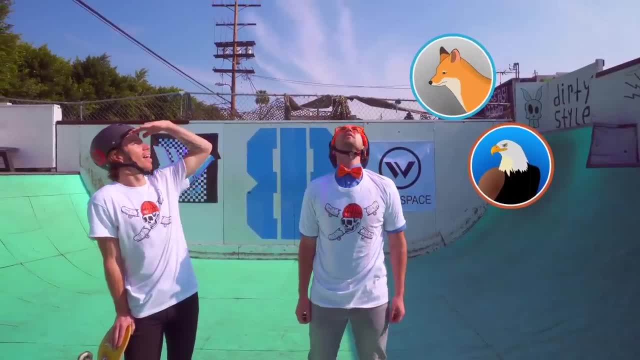 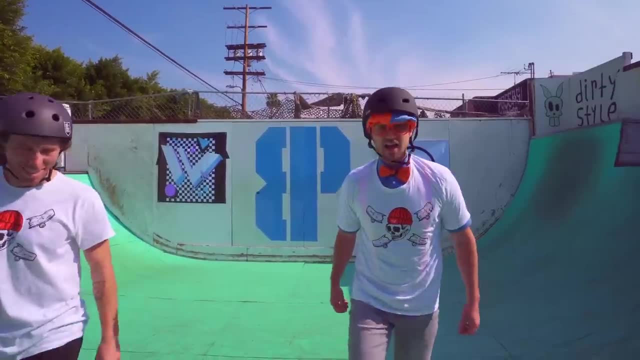 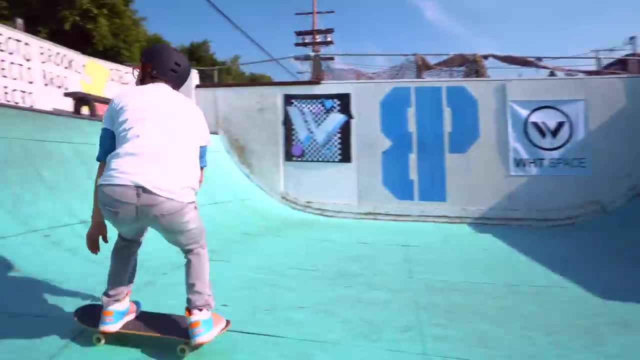 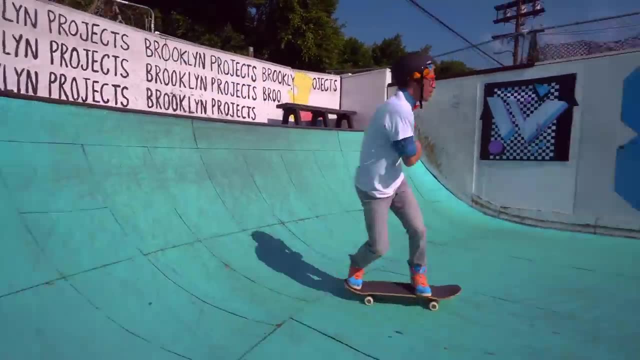 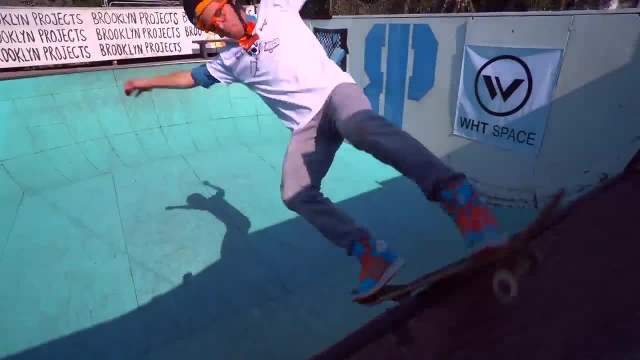 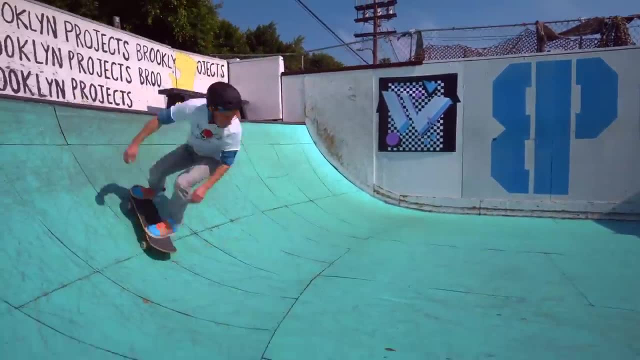 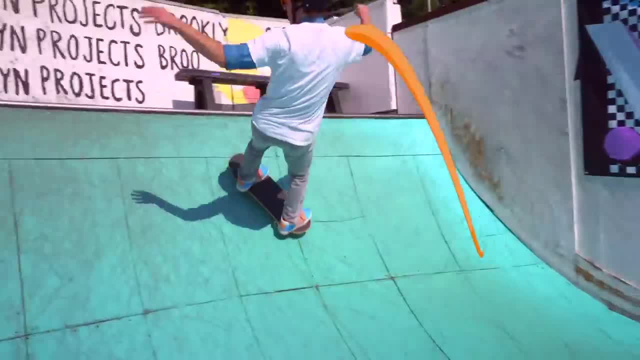 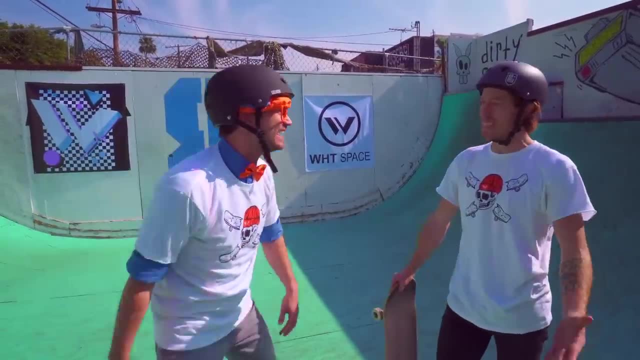 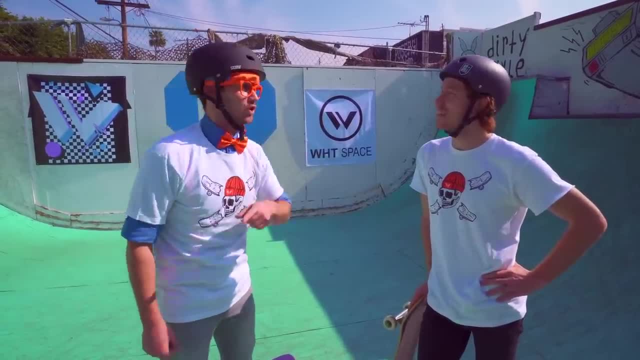 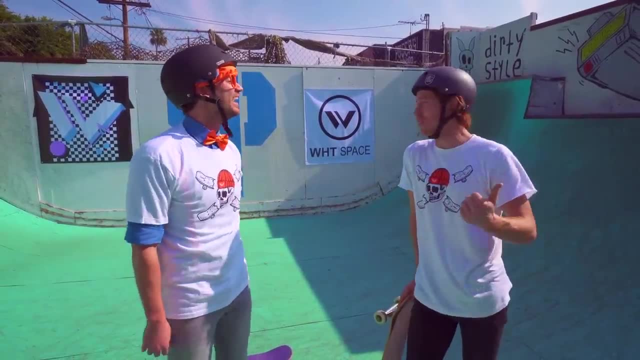 Really, Yeah. Well, thank you very much for teaching me. With a good teacher, you can do a lot of cool things, No problem at all. Well, hey, I had an amazing time skating with you. I've got to head to another skate park, but we should do this again sometime. 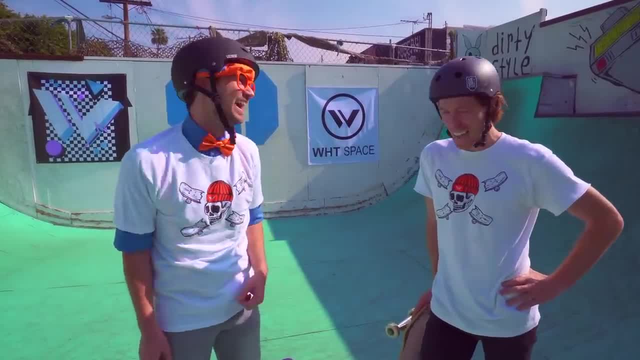 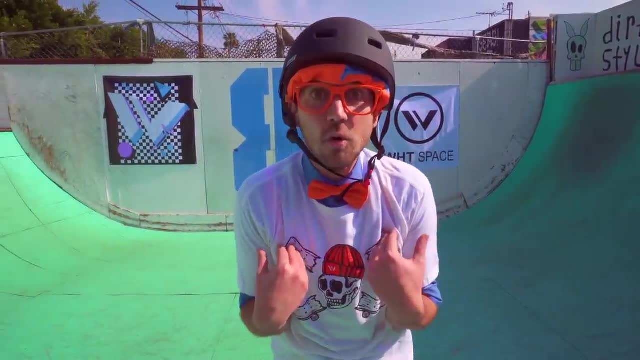 Maybe I'll take you to the mountains and go snowboarding. Really, Yeah, Try that out. Well, I really appreciate it. All right, See you, bud. Did you hear that Maybe I'll get to go snowboarding with Shawn White? 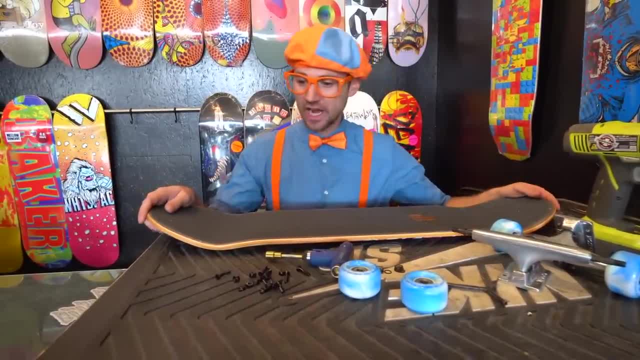 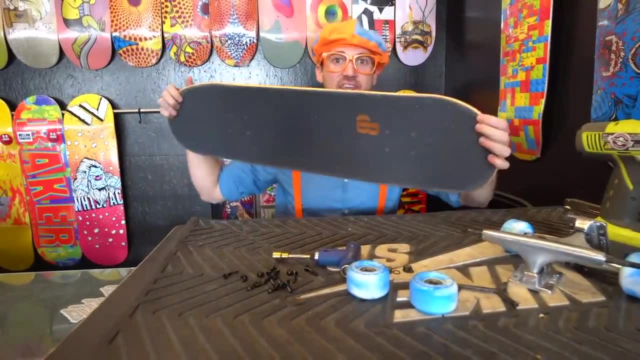 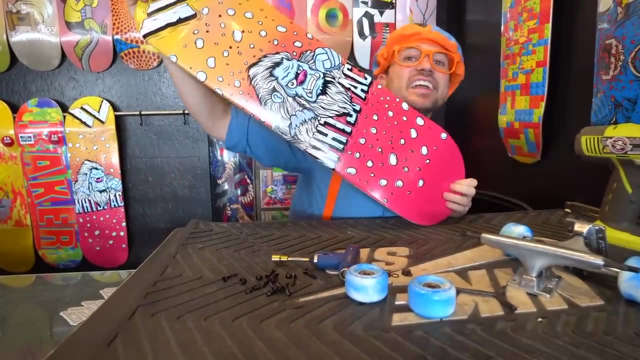 Whoa, Hey, Whoa, Check it out. Let's learn how to build a skateboard. See this, Whoa, This is a skateboard deck. Whoa, And this one has a really cool design. Check it out. Whoa, That's silly. 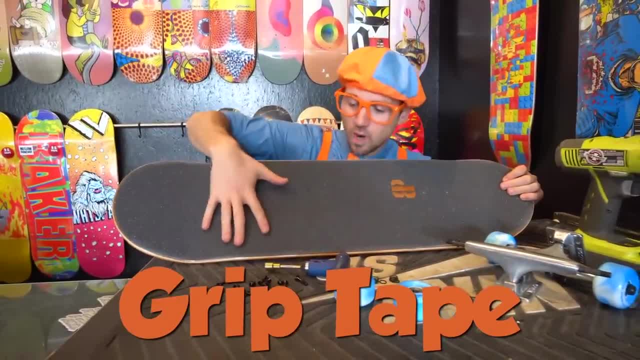 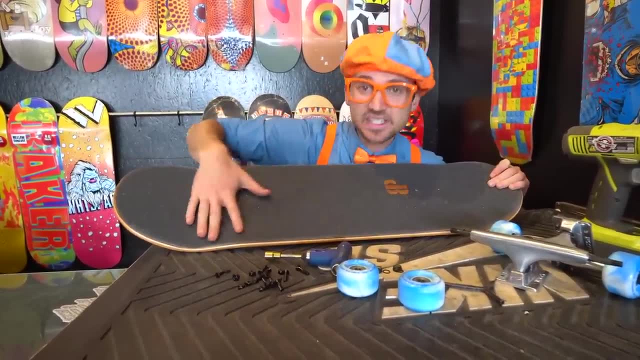 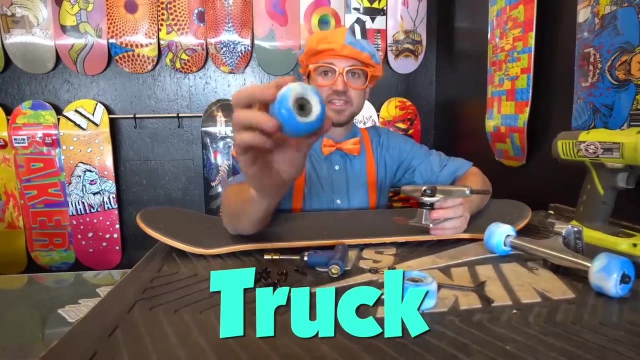 And see this on top. This is grip tape. Whoa, It's kind of like sand and you can't move at all. So then your feet don't slip and slide. Okay, And this is what's called a truck. Ooh, And you know what these are, right. 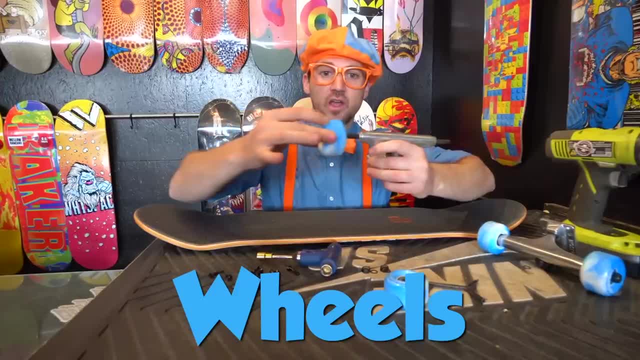 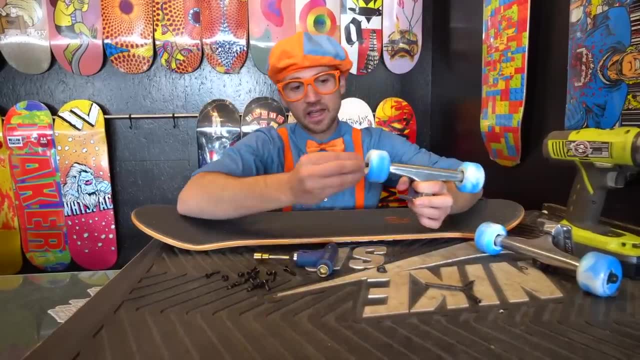 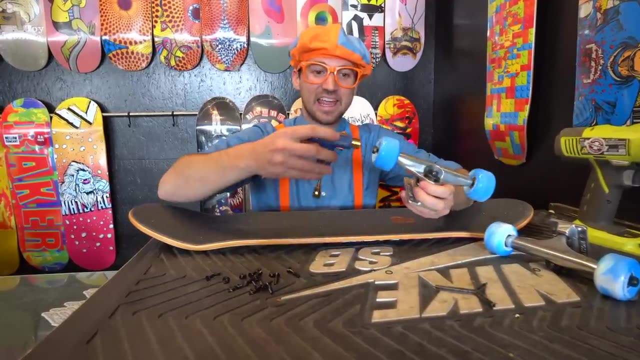 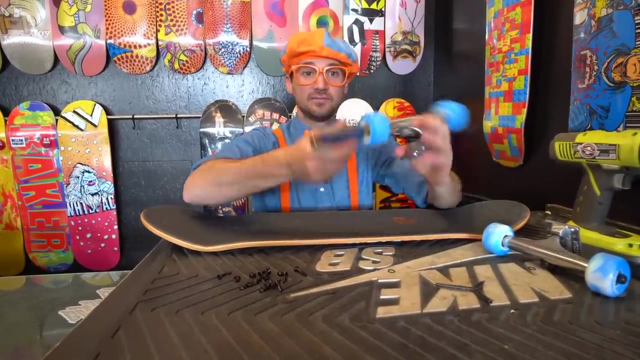 Yeah, Wheels And how these work. you put the wheel on the truck, put the other wheel on the truck, and then you screw in the nut and make it nice and tight, And then you do the other one. Whoa. 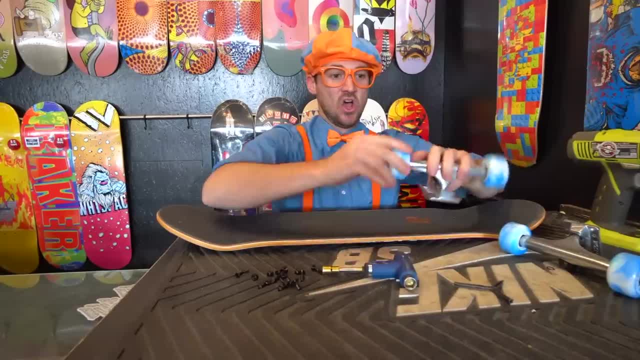 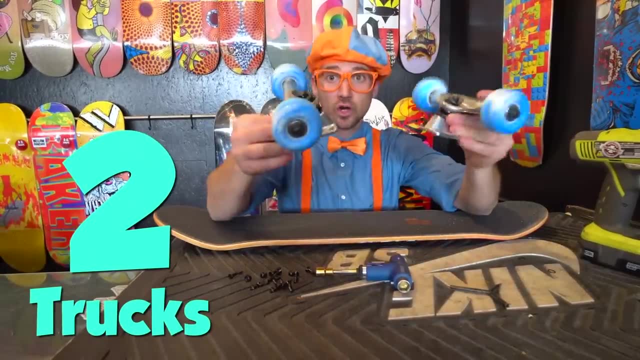 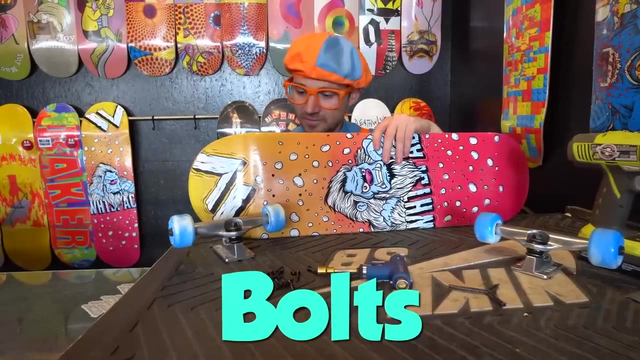 All right, There we go. Whee, See it spin, Perfect, Perfect. All right, So you have two trucks, All right, And then put them on the bottom. After you put these bolts, let's put four of them in there. 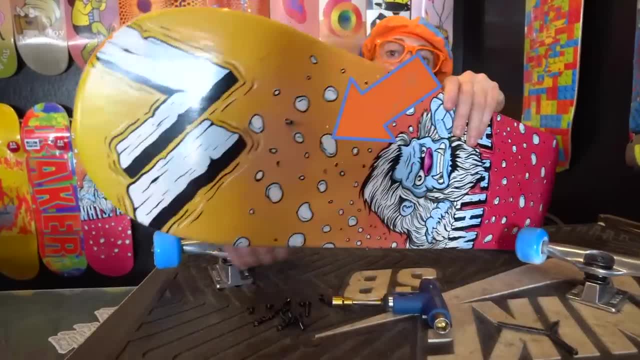 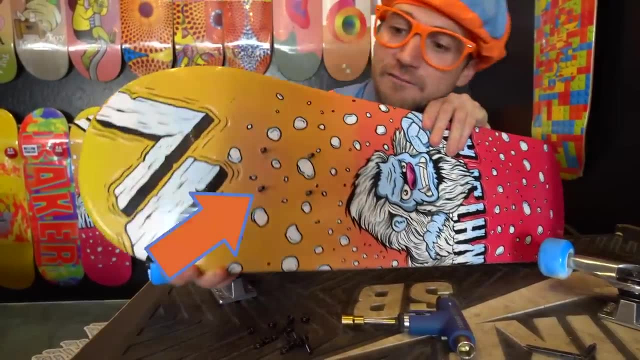 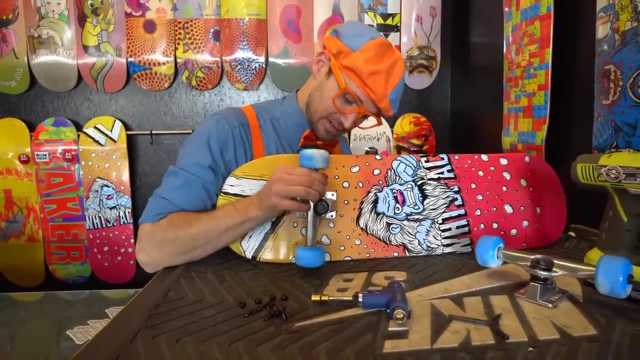 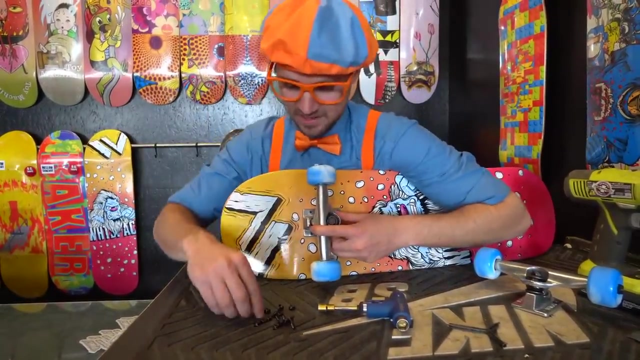 One, Two, Three, Whoa Four, Perfect. Okay, Let's put the truck right here. This is a little tricky. Okay, All right, There we go, All righty, And then you put some of these, And then you put these right on there. 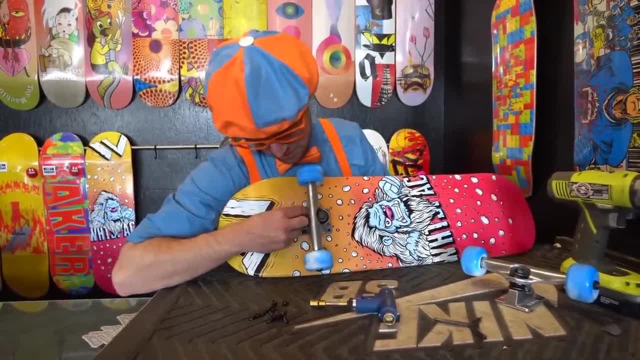 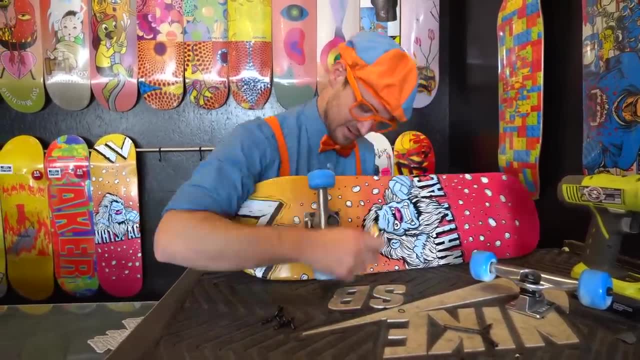 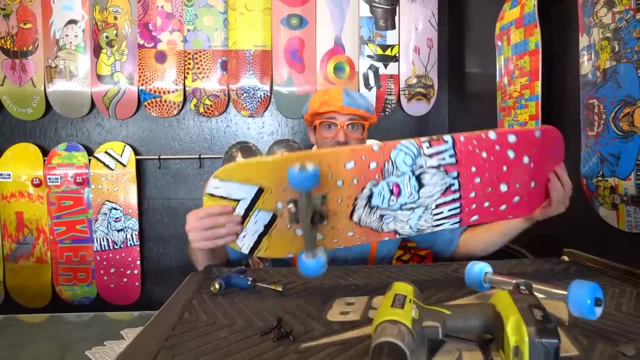 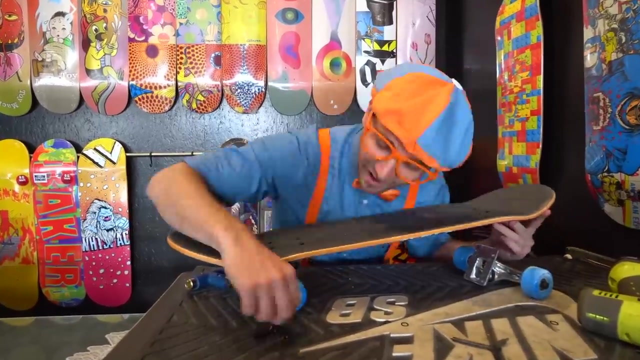 and you spin it around And you make it nice and tight. Okay, Watch this. Okay, One of two is done, Perfect. And then this other one. Okay, One of two is done, Perfect. And then this other one. 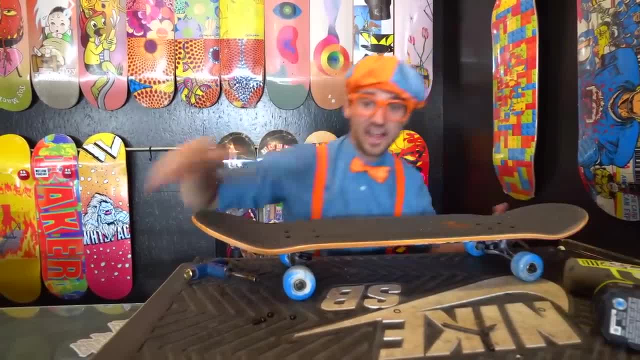 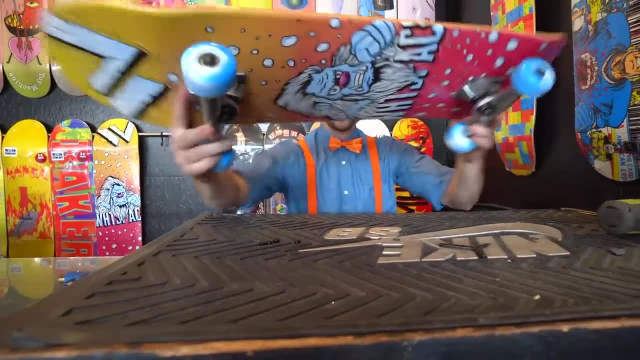 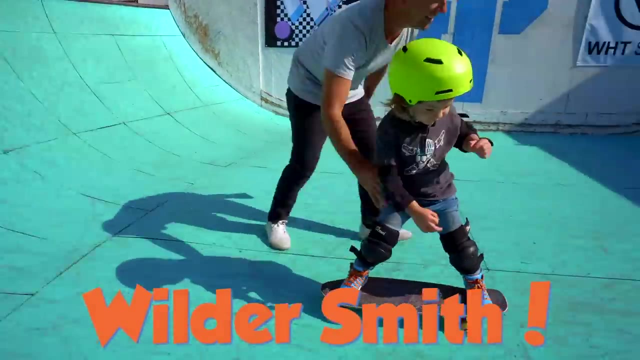 And then this other one. Okay, One of two is done. Alright, kids, So it's done. Cool, Perfect, Great. There we go, Check it out. It's a completed skateboard. Pretty cool, huh, Yeah, Walk out. 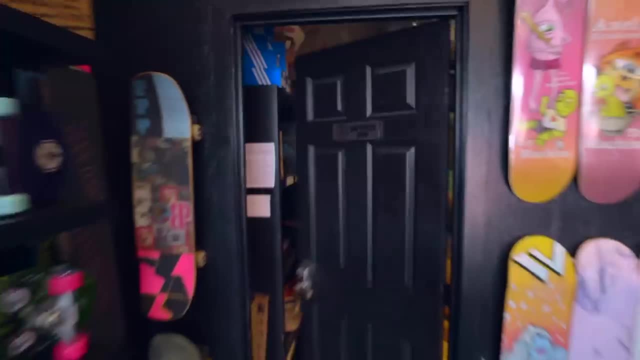 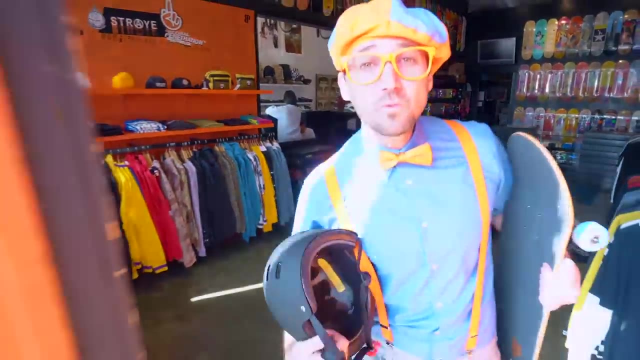 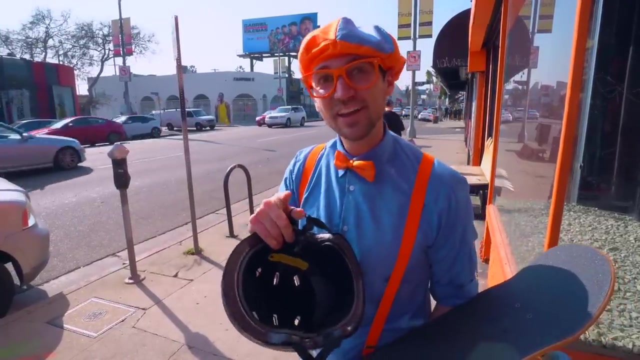 Yeah, Yeah, Don't forget to Gen grease. There you go, Perfect, There you go. Bye guys, Bye, Bye, Bye. Oh, that was so much fun learning about skateboarding with you. If you think skateboarding sounds fun, you should try it. 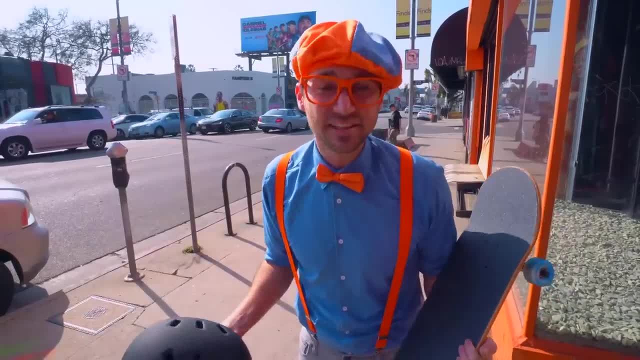 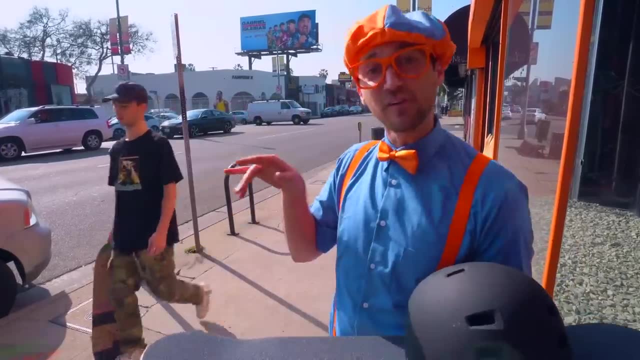 But always remember, wear your helmet and all of your safety equipment. But hey, this is the end of this video, But if you want to watch more of my videos, all you have to do is search for my name. Will you spell my name with me? 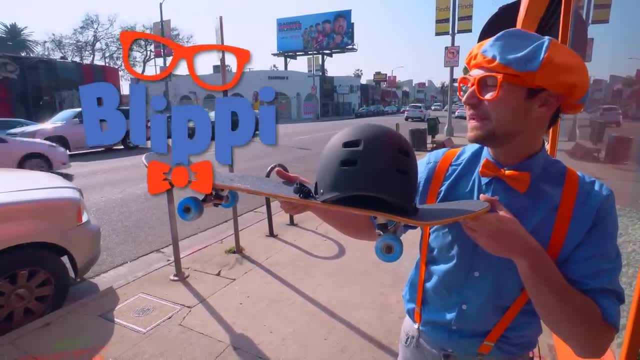 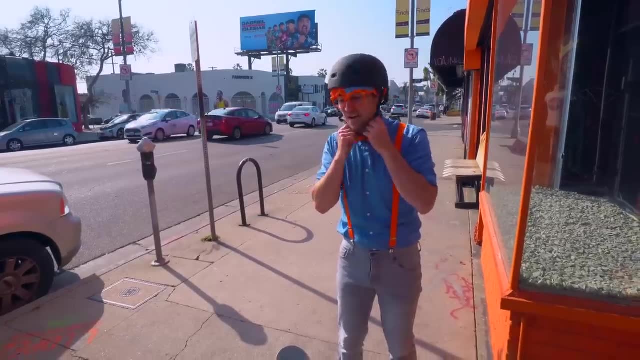 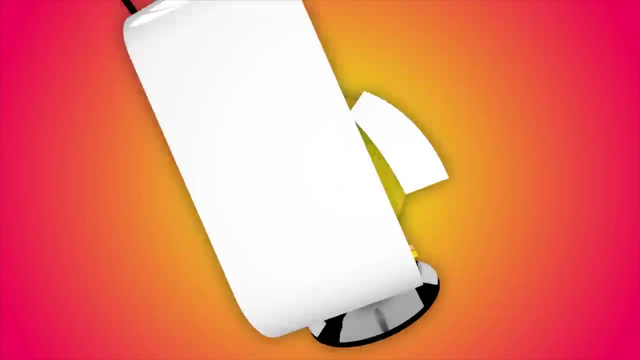 B-L-I-P-P-I- Blippi, good job. All right, let me put on my helmet. Okay, there we go. Let's go see you later. So much to learn about. It'll make you want to shout. 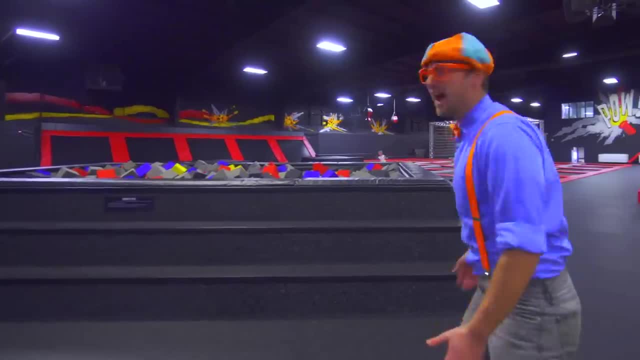 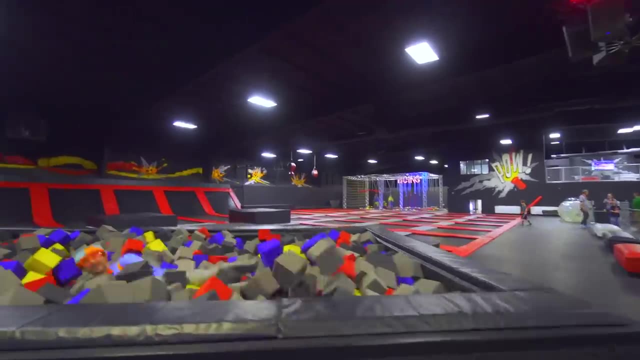 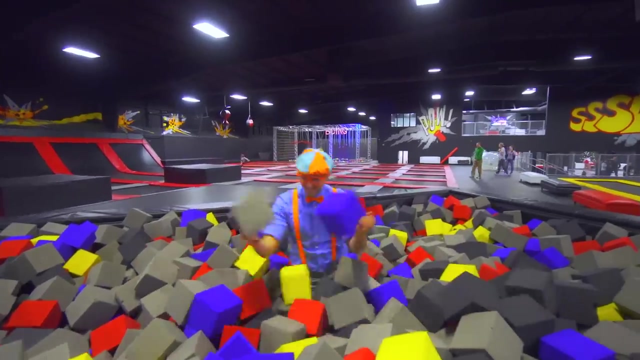 Blippi, Whoa. look at where I'm at. I'm at Boom Shaka in Olympia, Washington. Come on And you're singing Whoa. look at these. These are the color gray, yellow, purple and red. 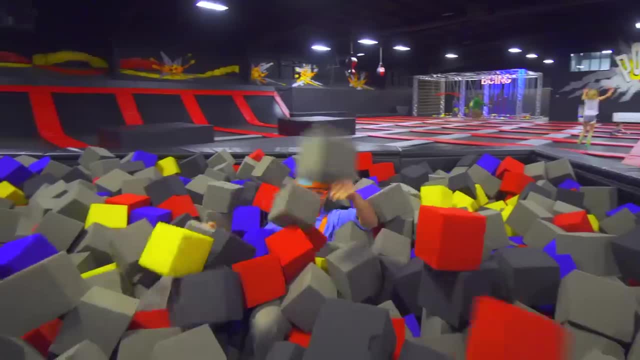 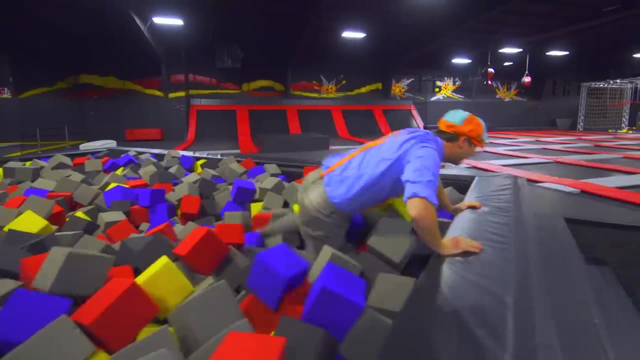 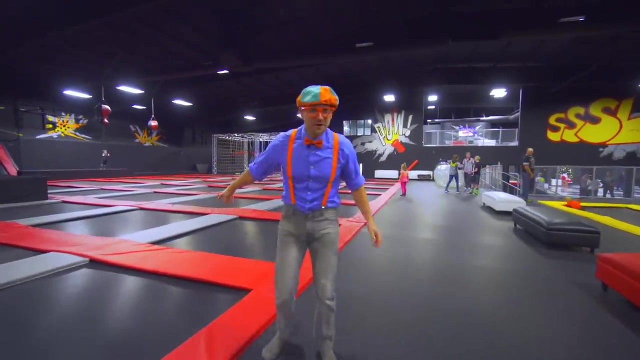 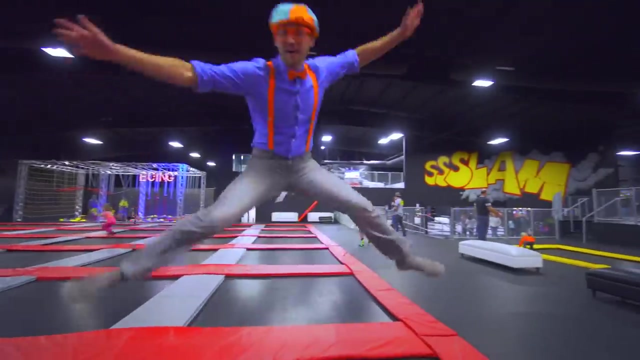 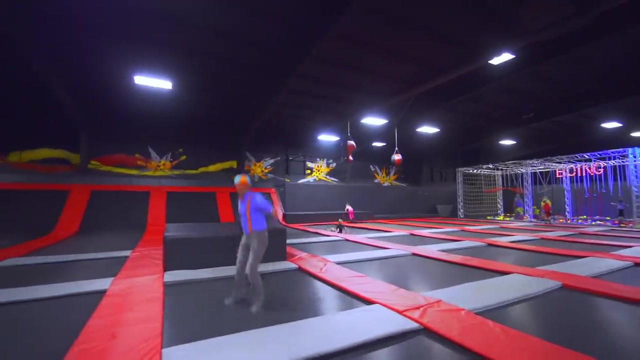 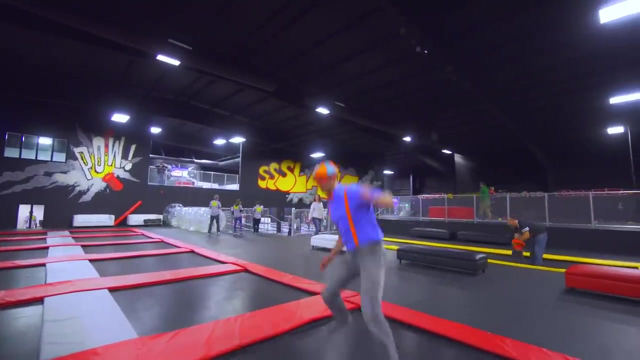 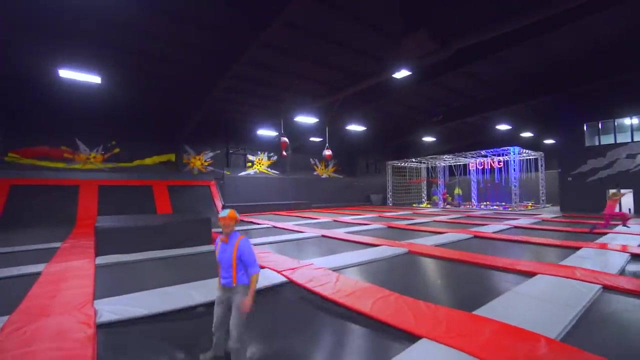 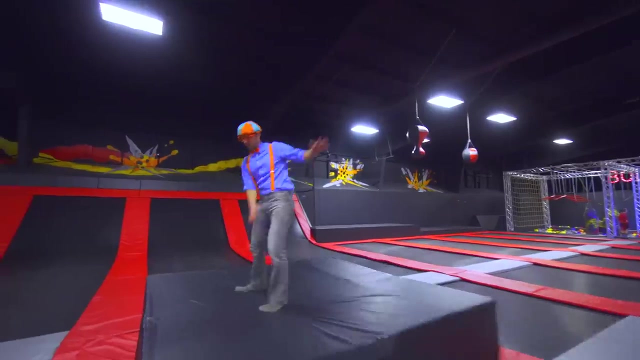 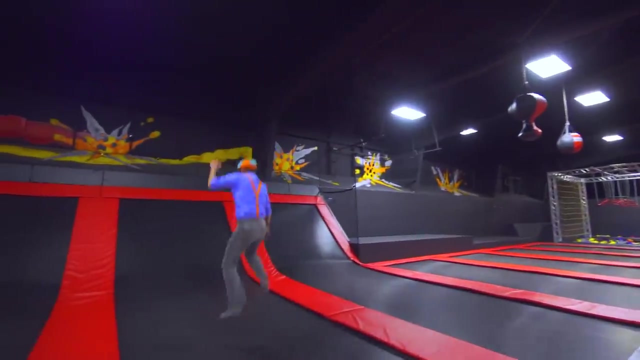 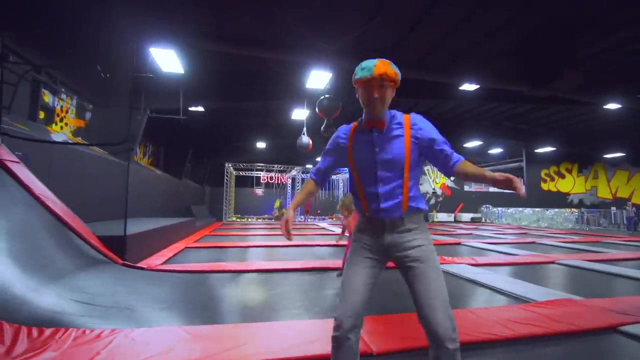 Whoa. Come on, Whoa. What are these? Look Boing Whoa, Let's go that way. Come on, Whoa, Here we go. Whoa Whoa. This is so much fun Jumping on these trampolines. 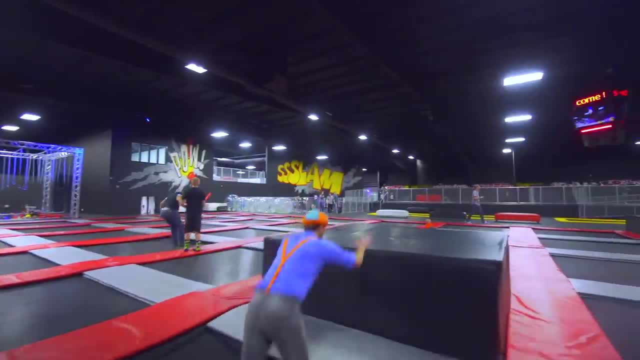 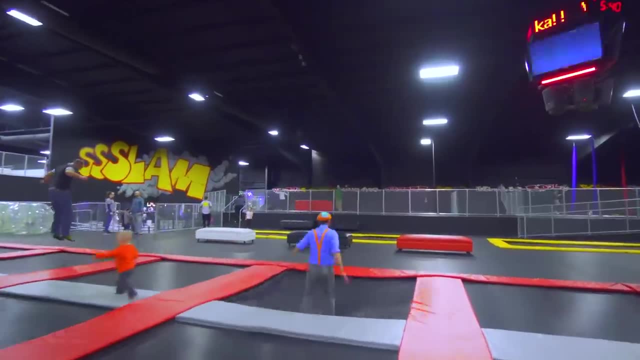 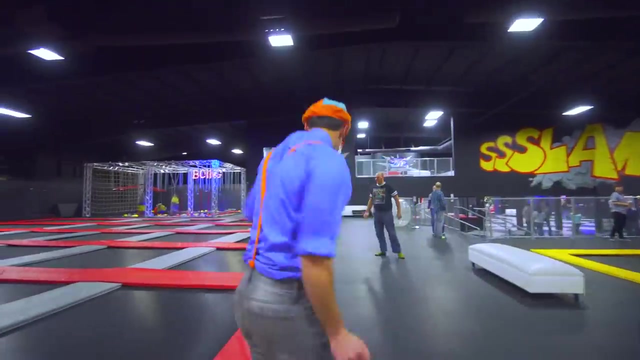 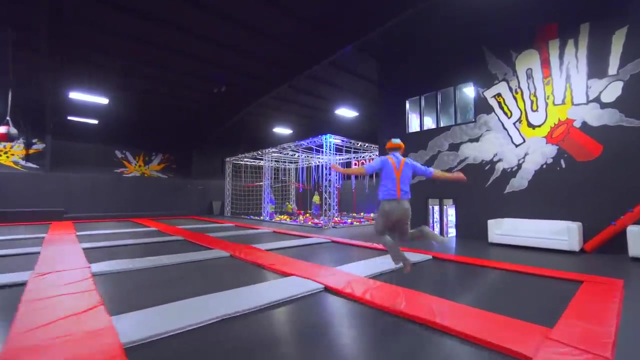 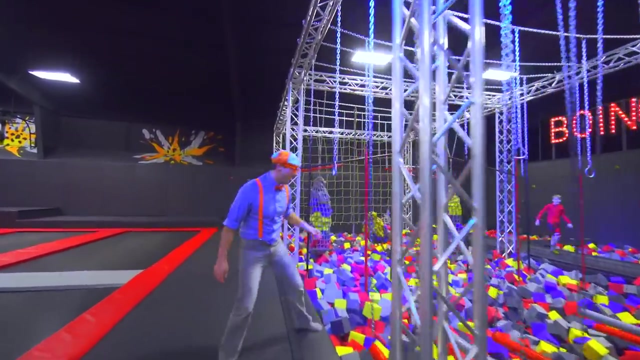 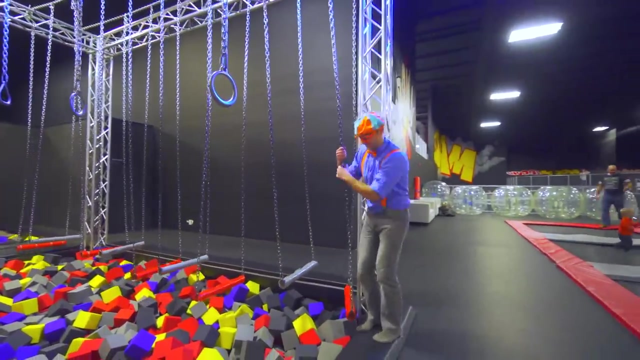 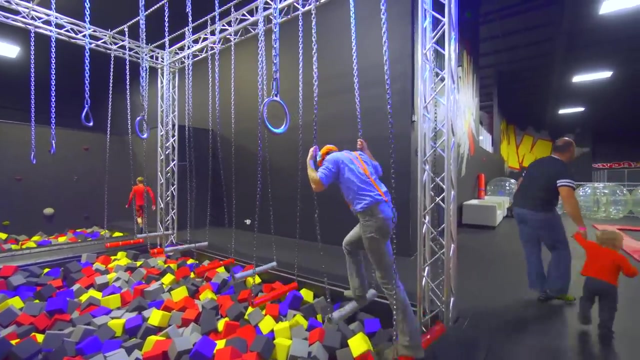 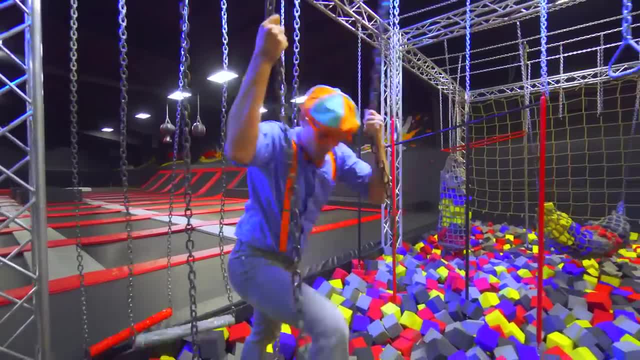 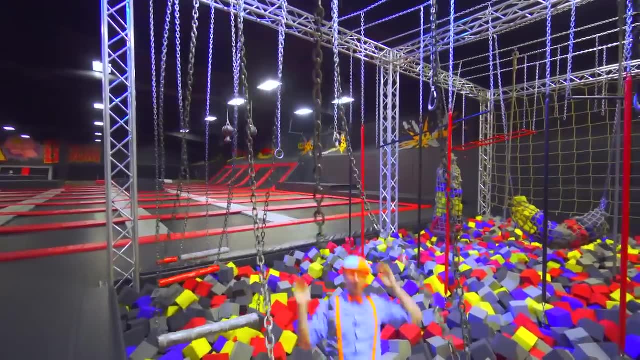 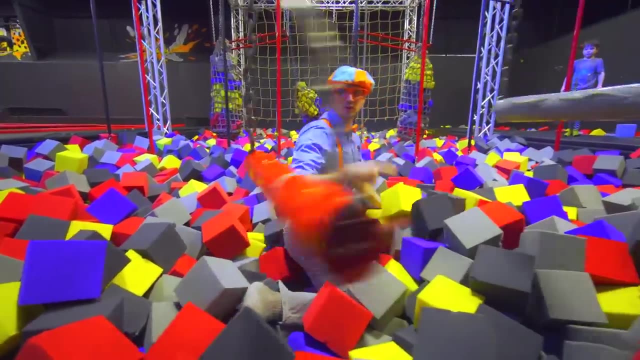 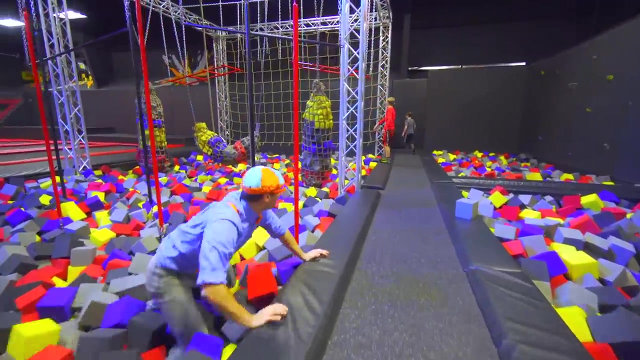